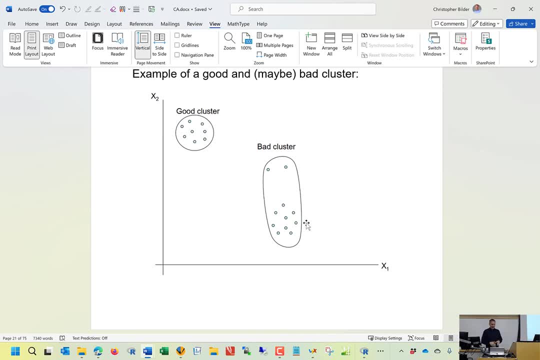 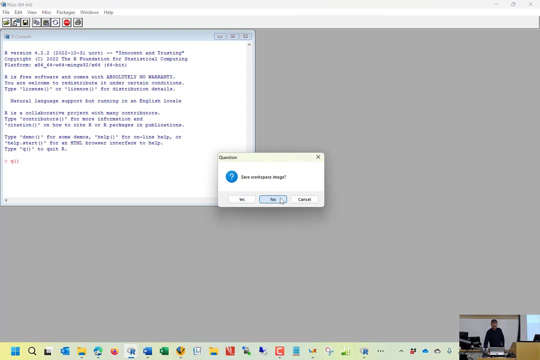 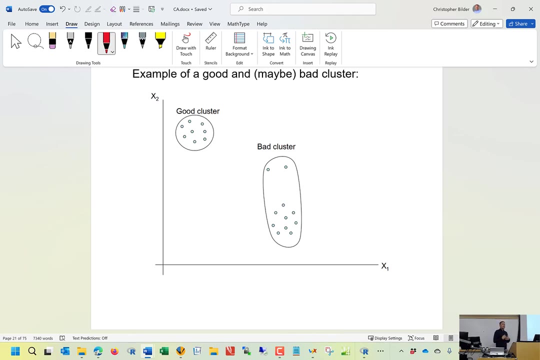 two variables, x1 and x2.. And in the upper left-hand corner we have what I would call a good cluster. Notice how all those points are nicely close to one another, meaning that they are similar. The distances between those points will be relatively small. 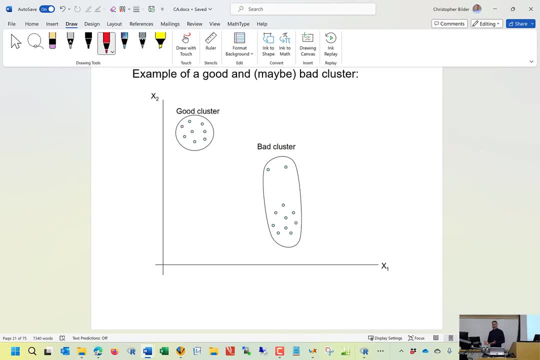 Then on the right-hand side, here we have potentially maybe a bad cluster Where, you know, we have two distinct, let's say, sets of points here, But they have been. I guess I've drawn a line around them to say, well, maybe this is a. 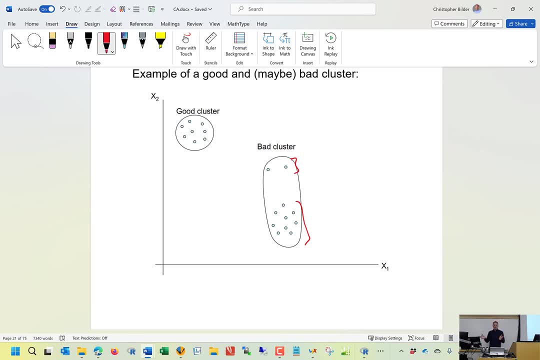 cluster itself. Now, relative to x1, you know we see these points are similar to one another, But relative to x2, they are not, because we have this big distance here. So typically, in some kind of clustering process that you use, you're going to get to a point that looks like this, where now I've 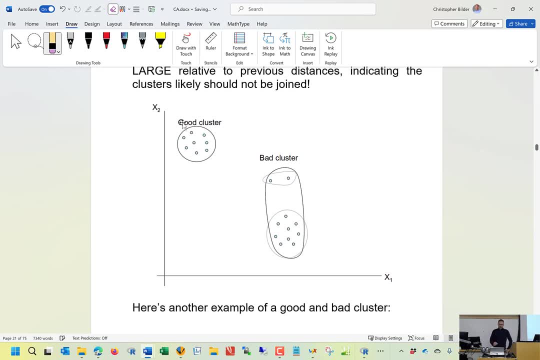 drawn lines, dotted lines, around what might be a more natural set of clusters, so that we would actually have three clusters. And so you often will get to a point like this: Now, before we get to this point, you know, rather than having three clusters, 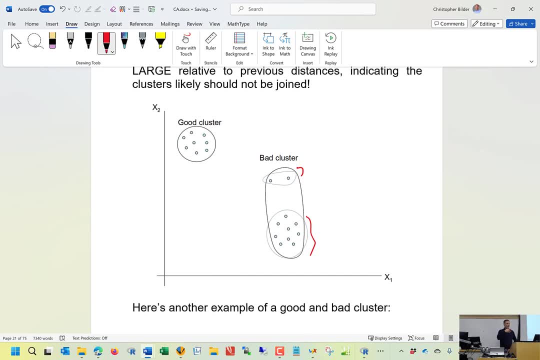 imagine if we have four clusters, five clusters, six clusters. you know the way that these hierarchical methods work. The distances that you're going to have when you go from, let's say, six to five clusters or five to four clusters is. 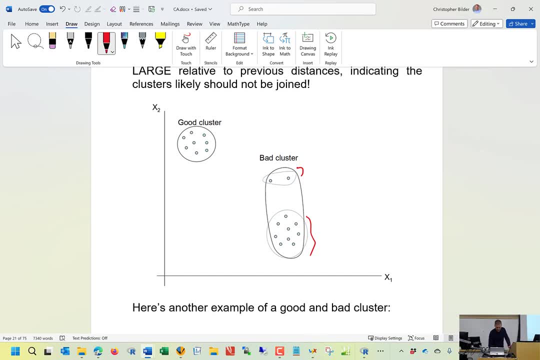 going to be relatively small. So perhaps, for example, maybe when we had four clusters, we might have had something that looked like that. And if I were to, you know, look at the distance between, let's say, this cluster and this cluster. the distance would be. 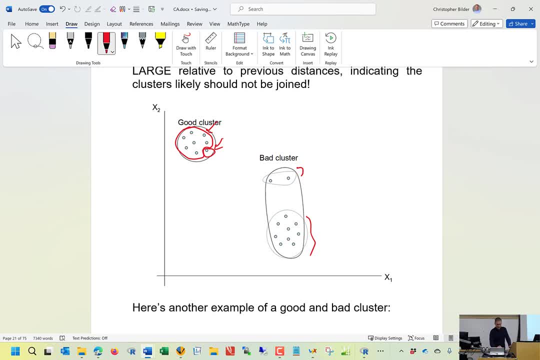 relatively small. But let's say again, we get to this point where we have these three clusters To make a decision about. well, should this here go with that cluster or should that go with that cluster? do you think the distance is? 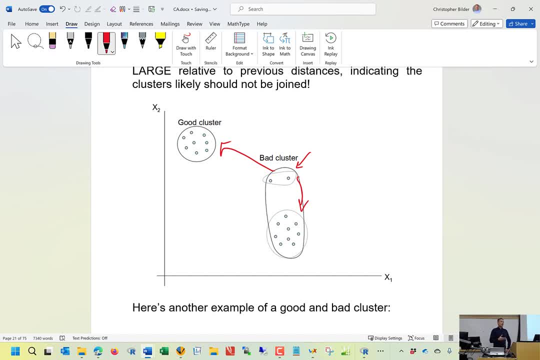 going to be large or small. It's going to be large relatively to everything that we've done previously, And so this is a very, very, very key point here. is that the distance to make a decision about what's going to be put together next, that distance or that? 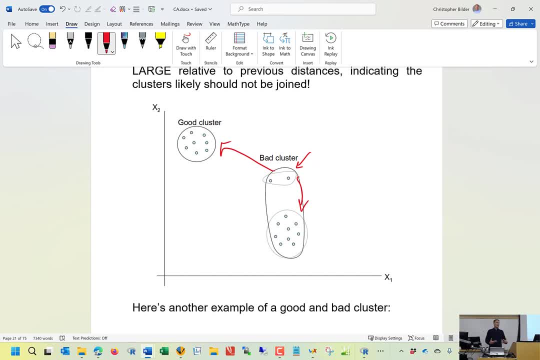 similarity is going to be large relative to your previous distances that you've used To join clusters together. That is a key point. Once you see something like that happen- and I'm going to repeat myself- where the distance is large relative to. 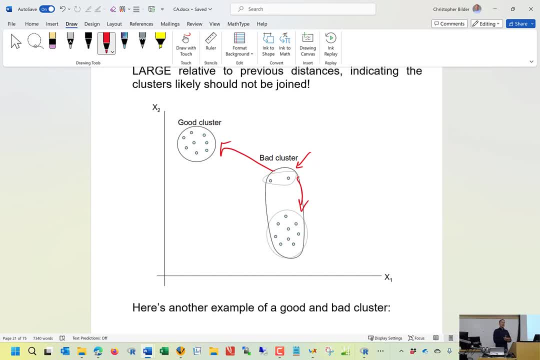 what you've been doing before in terms of joining clusters. once you see that happen, then you might be thinking, uh-oh, maybe I don't really have two clusters here, maybe instead I should have three. And essentially you say, okay, I'm going. 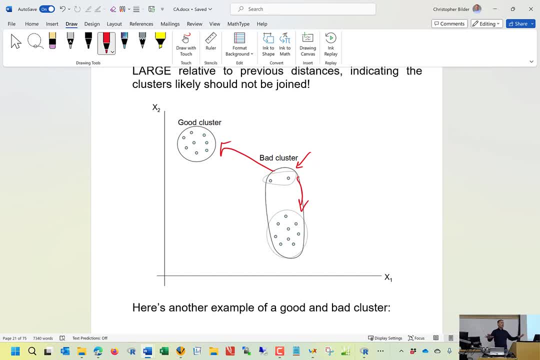 to stop. I'm going to go with three clusters. That is the kind of logic that we're going to use to make a decision about how many clusters we should use. Hopefully that seems intuitive to you, Because I think in the end it is, And we can easily, you know. 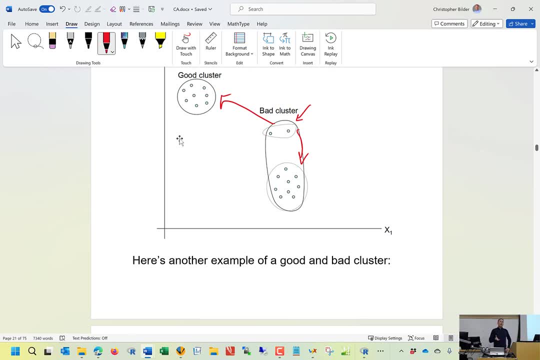 diagram this out in two dimensions. but you know again. you know what happens if you have, let's say, five variables, ten variables, twenty variables, hundred variables. You still make that same, you still go through that same thought process, While you're not. 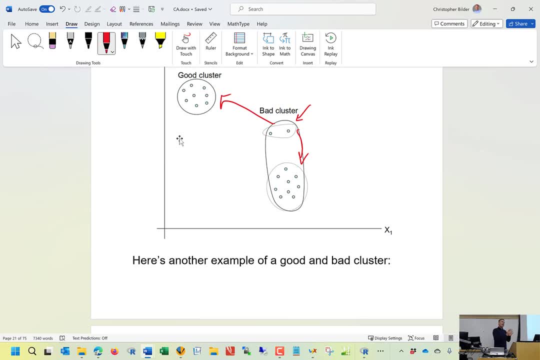 going to be able to see a lot of this. you can compare distances that are found during your higher clustering process And when you see a large distance relatively to what you did in the past, that should be a warning message to you that, okay, maybe I've gone. 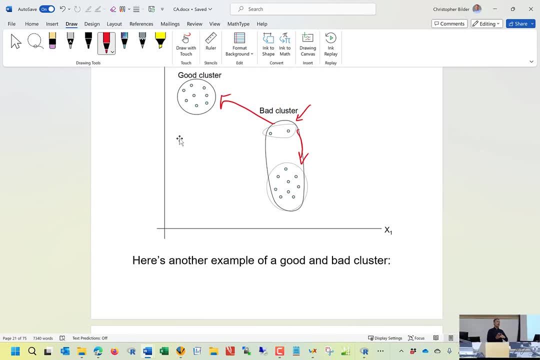 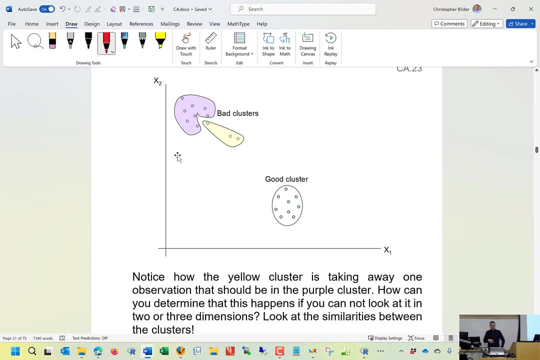 too far And I should actually, in this case more before. Okay, Okay, And I'm going to go with three clusters. Here's another graphical example of two variables. So again we can see we have a nice cluster here. 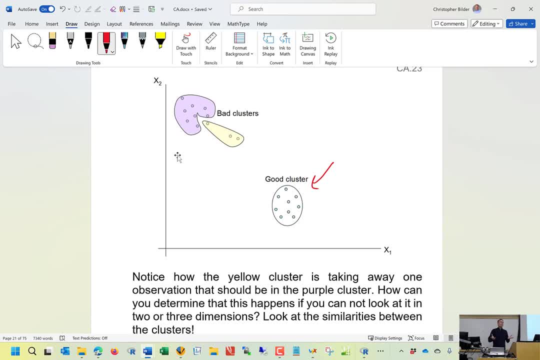 None of these seems kind of similar to one another, And people would refer to this as a compact cluster. It's rather, you know, if you think of it this way, the radius is about the same throughout the cluster. That's a good cluster. 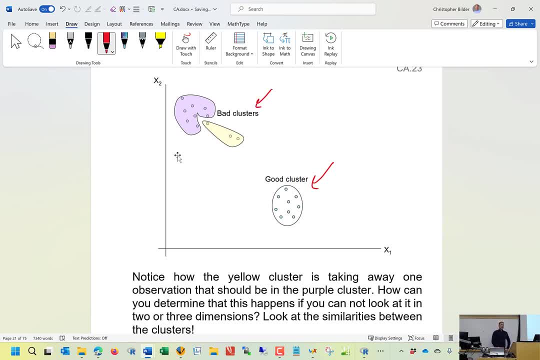 This is. This is: Let's set them back- clusters here, And hopefully it's obvious. You would normally think that that one point that's in the yellow there should be with the. at least on my screen, I have a purple cluster and I have a yellow cluster. 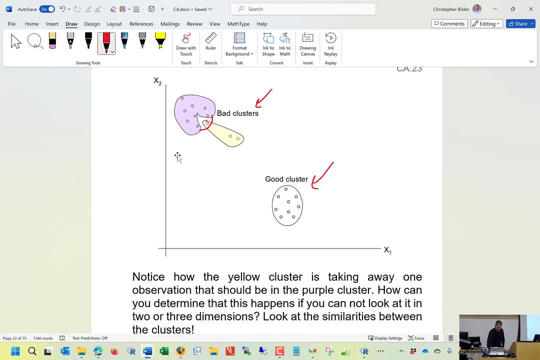 At least from my angle here, it's hard to see. You would think that this point here should be with those other points. That's what you would think, But in actual clustering methods the clustering method might come up with something like this: This is an example of that cluster. 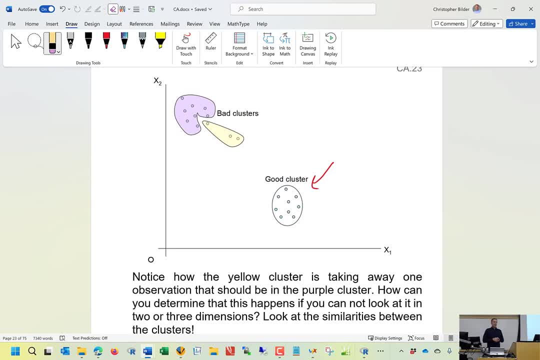 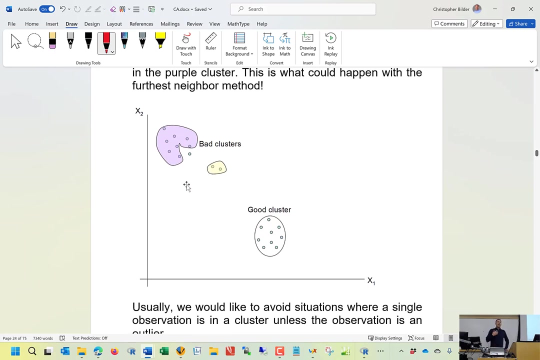 Or you might think of a way it's like what cluster can we do something with? But think of what firmness neighbor does. The firmness neighbor method defines the discipline, The distance between clusters, as essentially- let me do this, So maybe I got to this point here- 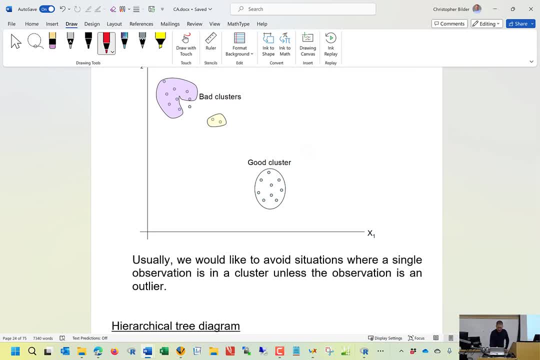 And I'm going to need to make a decision about which clusters to join. next, And I'm probably going to center on that little point there, This cluster that has just one observation limit And, if you think of firmness, neighbor and it's way of defining the distance between clusters. 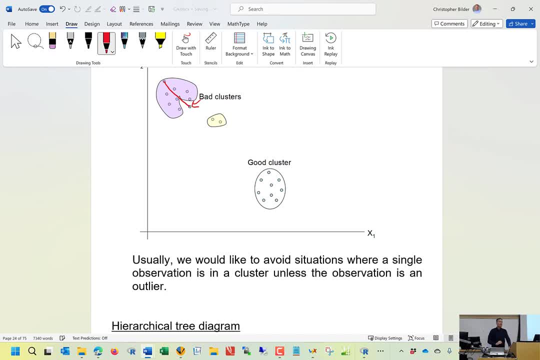 That distance would be between this point and this point. That would make a decision about should that point go to the upper left hand corner cluster, the purple cluster on my screen, And also this point compared to this point in terms of distance, Those distances relatively at least. I was trying to draw it this way. 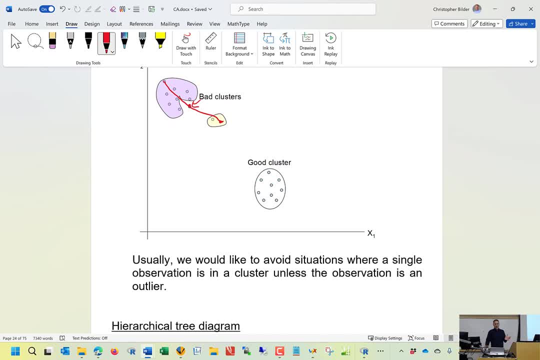 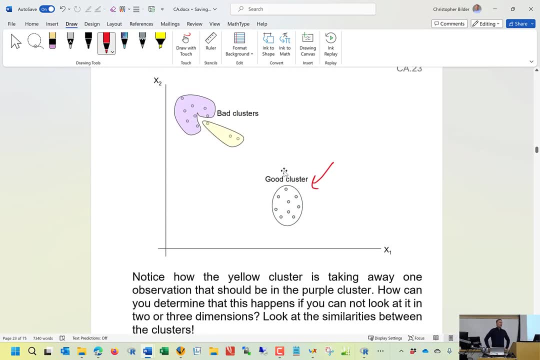 are about the same distance. So if this distance here was just a little bit smaller, then we would have something like this, Which isn't you know. just from looking at it in two dimensions, it doesn't look like it's a good choice. 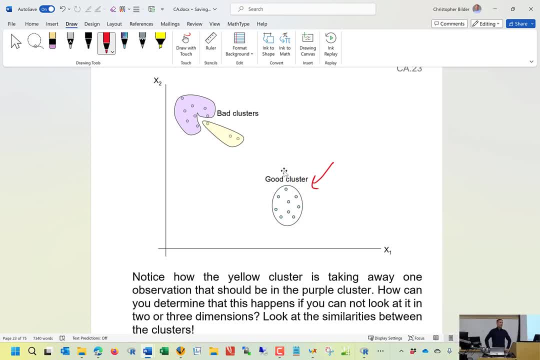 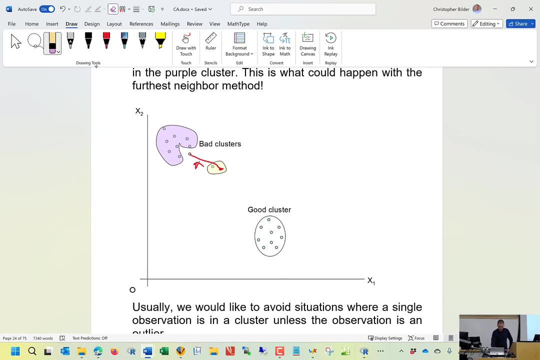 But that's what can happen with firmness, neighbor. Now again, let's think of it in terms of distances. before we got to this situation, Before we get to that situation, you know, relatively the distances or the similarities should be relatively small. 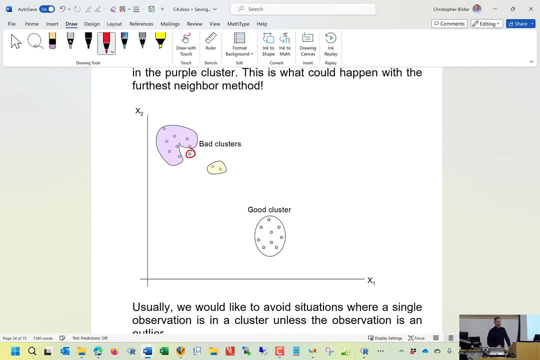 Then, when we get to a process where we have this remaining now, we have a distance that seems to be much larger than what we would probably have before, And so because of that, that might make you think, okay, wait a second, maybe I should stop the clustering process. 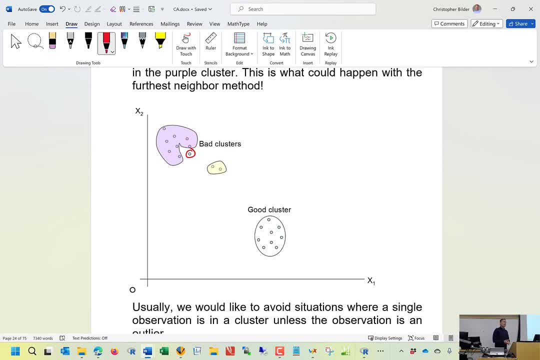 and actually end up with four clusters. Now, in the end, that's not ideal, because we can see- I think all of you agree with me- this is probably the way it should be, But this is also a nice little illustration about how some of these clustering methods. 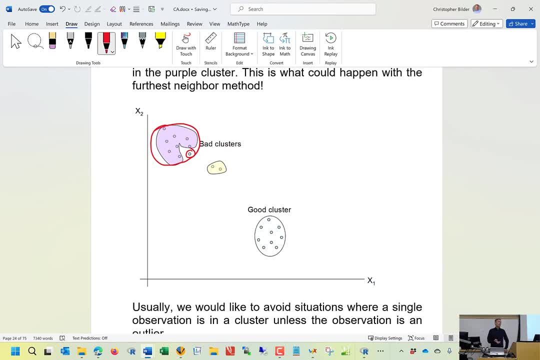 don't always give you results that necessarily always make sense. This is why we look at. you know more than one clustering method. That's why they exist. I should say You know some clustering methods might work well in some situations. 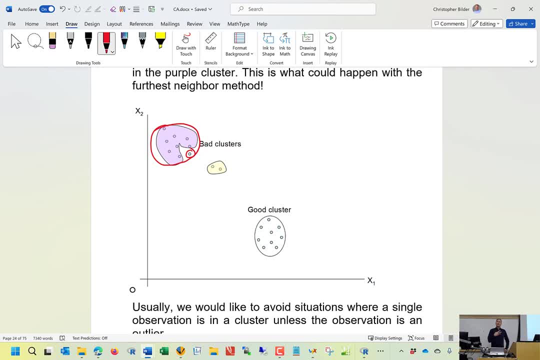 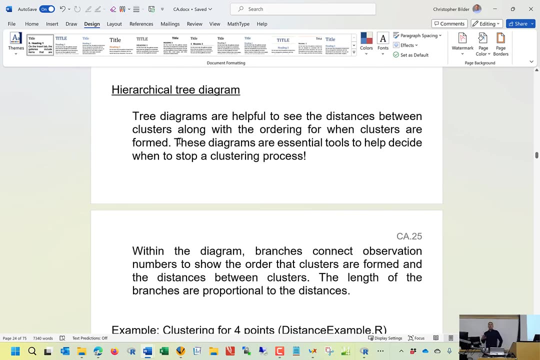 some might not work well in other situations, And so that's why it's often good to try out multiple clustering methods. Okay, Any questions about that? So distances between, let's say, successive, let's say, iterations of the clustering algorithm. 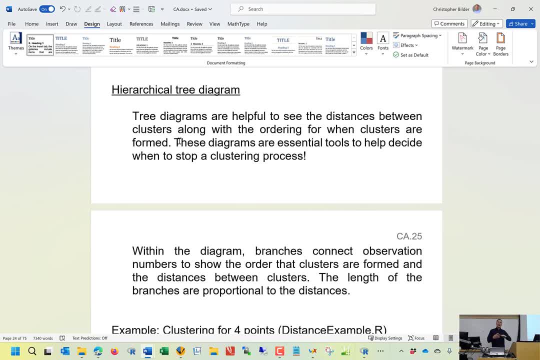 are very, very important to us. That helps us make a decision about when I should stop the clustering process instead of going all the way to just having one cluster, And so there is a nice plot that we can use called a hierarchical tree diagram. 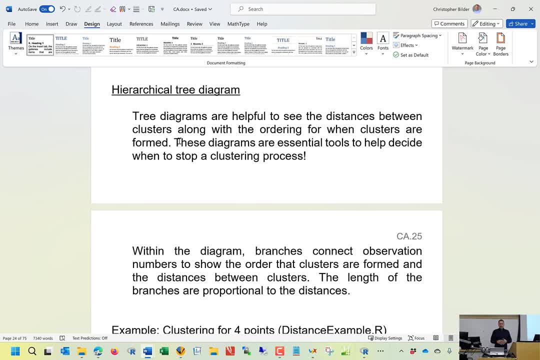 that allows us to see it. So this first diagram, the first example of it, is for that example where we just have four observations And from this plot alone we're not going to be able to make a judgment about how many clusters we should have for four observations. 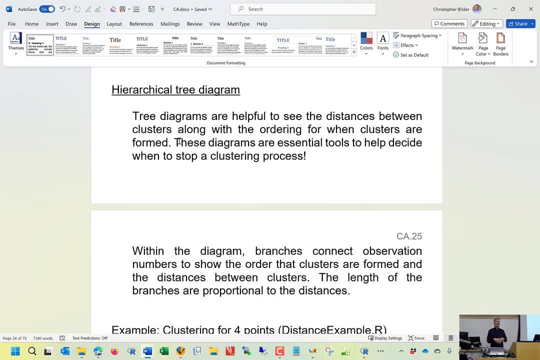 I mean you shouldn't do clustering analysis if you only have four observations. Maybe it's just some very convenient very, very small data set to help illustrate the process of clustering. And so my purpose here- this diagram for this data- is just so that you understand. 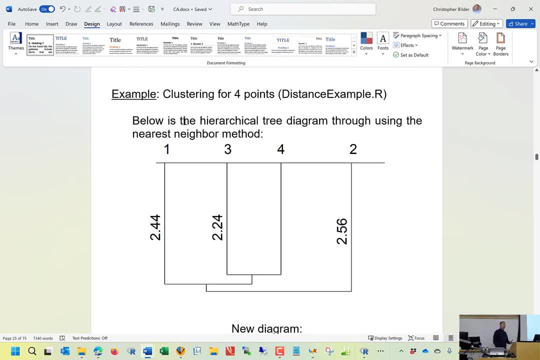 what's actually being represented Now. when I was going through my notes yesterday morning to prepare for this class, I was taking a look at this diagram here and I was, like you know, I think I could do a little bit better. 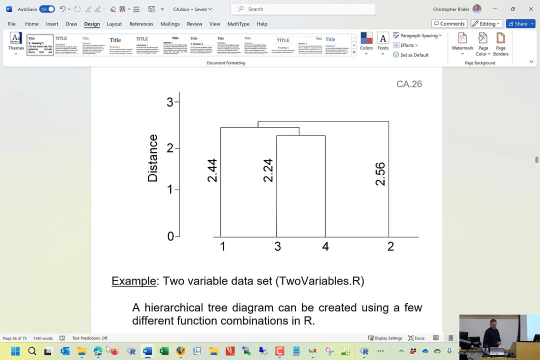 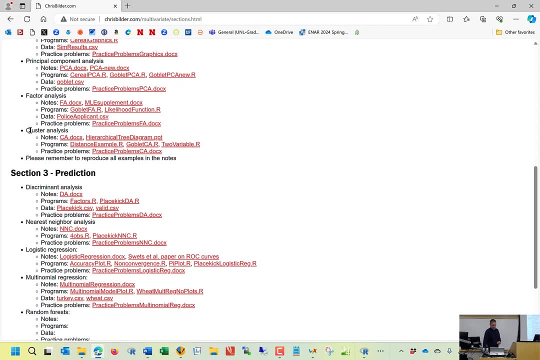 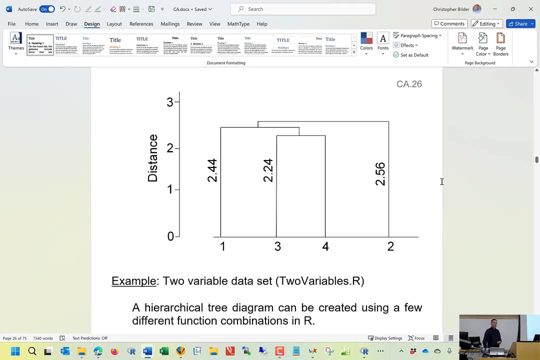 And so I put together a new diagram. If you want to actually download this diagram, it's simply available on my course website under cluster analysis It's called. this is PowerPoint file here. I just chose to draw it this way, basically kind of reverse the way it was drawn. 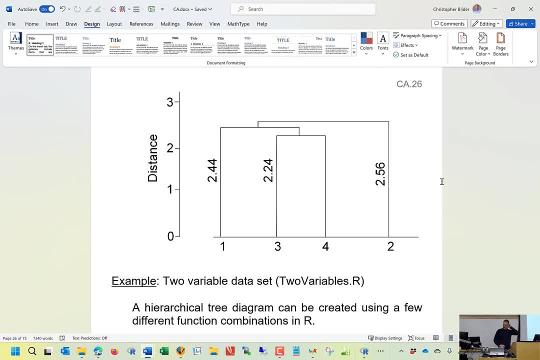 because this is the way that R is going to draw it. Different software packages would draw these kind of diagrams in a different way. For some reason, I chose something that was different than what R did. Okay, So this is what the plot looks like. 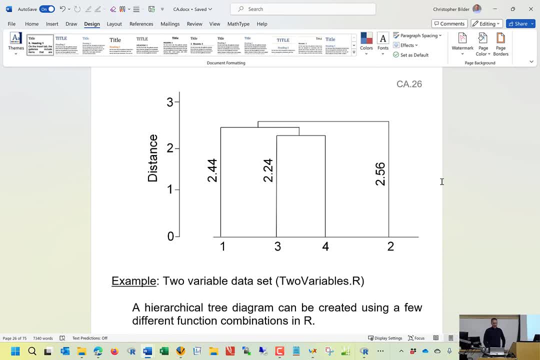 So we can see. we have, on the left side, a measure of distance. This distance represents when I'm joining these clusters together. what is, according to the cluster analysis method, what was the distance between successive clusters that were joined On the x-axis? 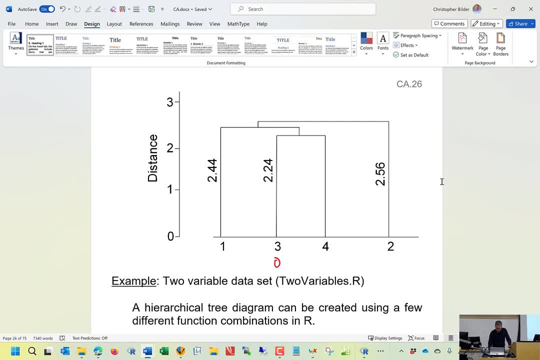 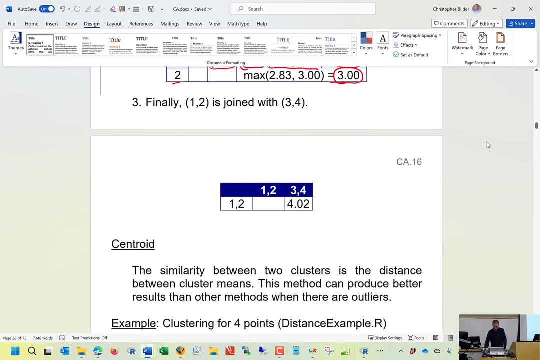 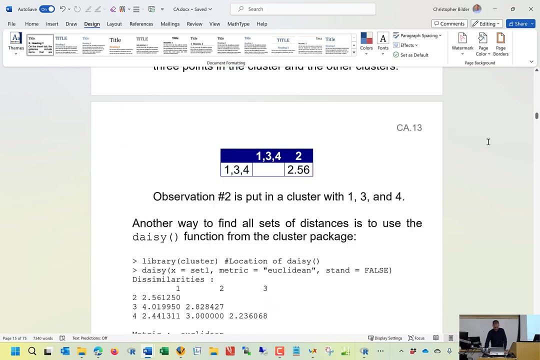 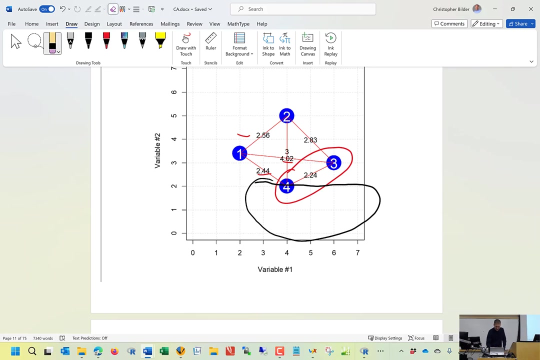 what we see are actual observations. Maybe I should even put that there. Observation number: Okay, Now if we go back, we'll look at nearest neighbor again. Go back to when we first looked at this. Let's see, here We're racing. 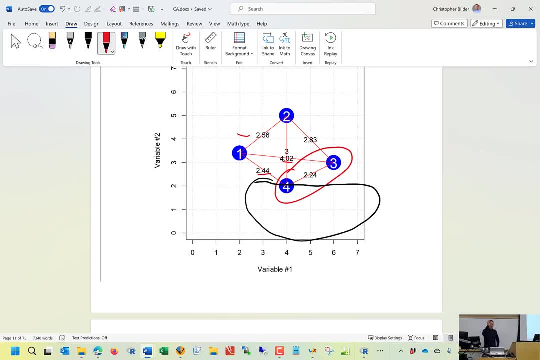 I still have the problem from last time. I'll just ignore the writing that I put on it. So we have these four different observations here. When we use the nearest neighbor method- remember the- we start off with four clusters: The clusters that are first joined. 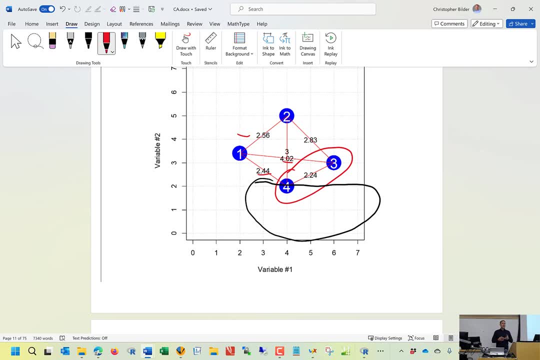 are the clusters that have the smallest distance between one another. Each observation is a cluster. That smallest distance is just the smallest distance between observations, And it would be that 2.24.. So three and four were joined together first. Now in order to decide. 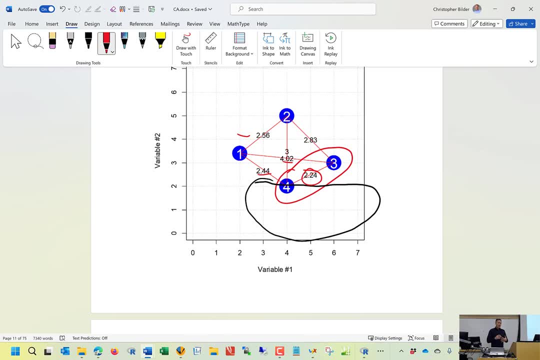 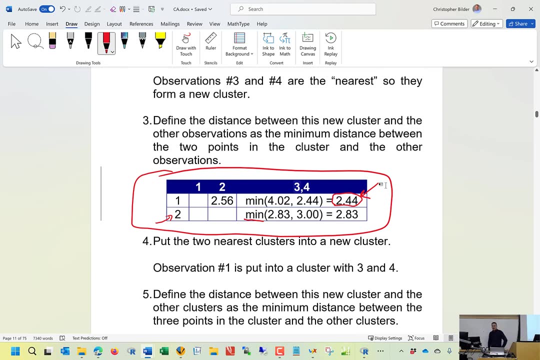 which clusters are joined next. then we look at the minimum distance between clusters And we look at a table such as this And we saw that the minimum distance was the distance between observation one and the cluster that had three and four in it, And so that would be joined next. 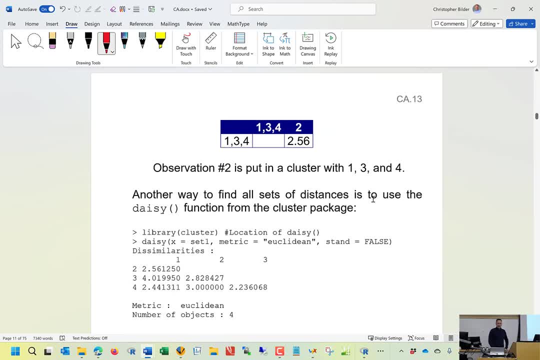 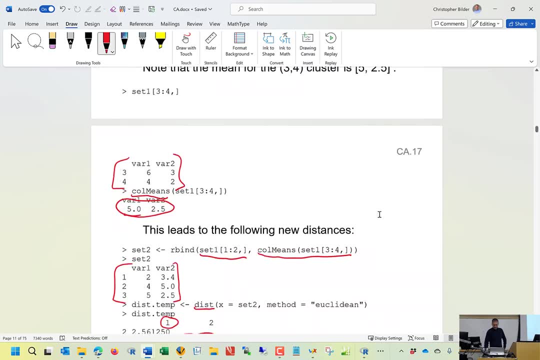 So I have one, three and four, And then of course at the very end then I join two to that one. three, four cluster, Okay, And I have a distance of 2.56.. So those distances now are actually shown in this plot. 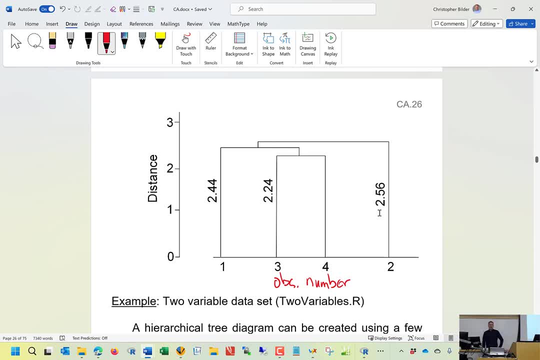 So, again, remember, three and four were joined first, And so the way that this is drawn is that we need to show that we have a connection between three and four, And so that's why you see these lines connected like this that connect three and four. 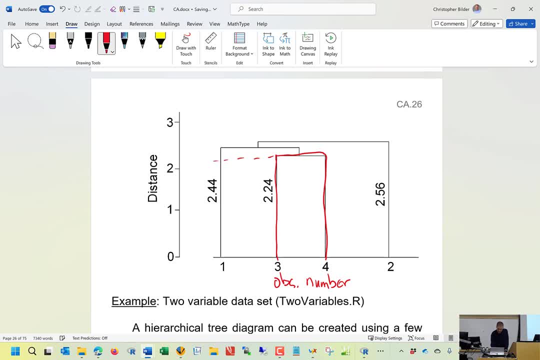 Notice it's drawn out to 2.24, which was the distance between those clusters, in this case observations. Okay, Next, remember, one was joined to three and four, And so we can see that, indeed, here's one. 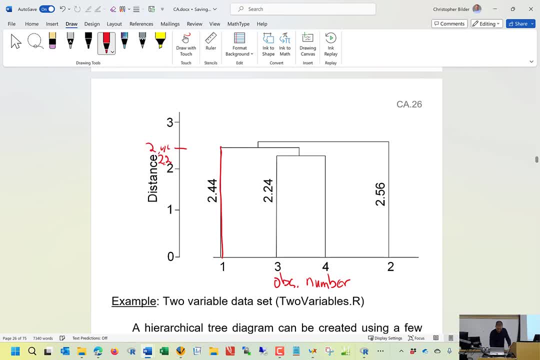 It's drawn out to 2.44.. And it's joined into what we had for three and four, And then, lastly, you can see how two is joined to the other ones. So this is a hierarchical tree diagram. It kind of gives you a history. 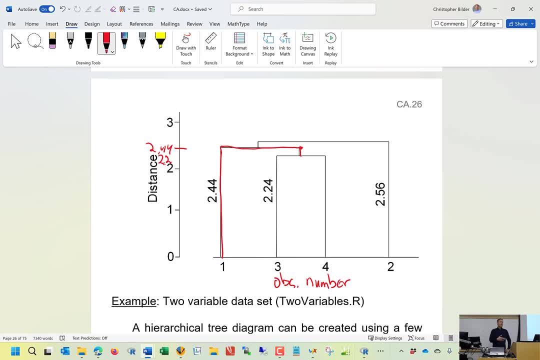 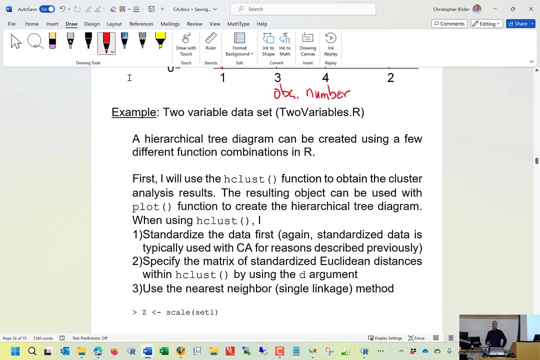 of the clustering process. It also shows you the distances. Typically on these plots you will not see this written out like that. I just did that there for emphasis. Okay, So let's actually take a look at a little bit larger data set- still small. 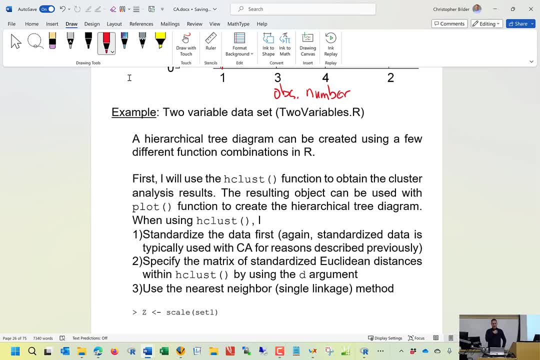 to help us understand what's going on here. It's simply also just two variables. This will also give us some experience with how R, how you can approach the process in R. So the main function that people use in R to do these hierarchical clustering methods. 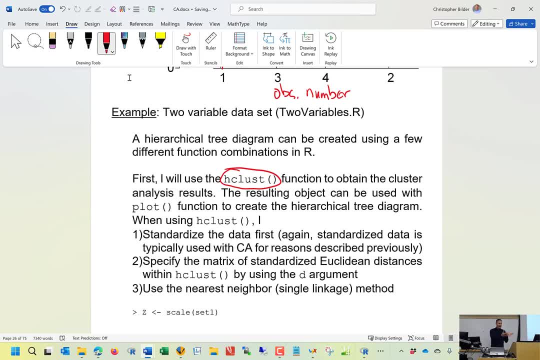 is what's called HCLUS, H for hierarchical CLUS for clustering. Okay, Now, in order to use this function, we actually have to do some stuff beforehand. First, remember how we typically always use standardized data, So we're going to need to use the scale function. 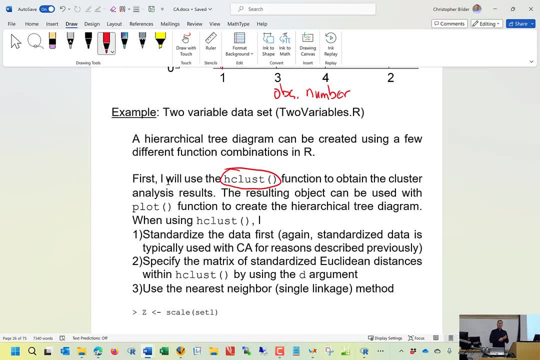 to standardize our observations. Second, we need to find all pairwise distances between the observations. We did this before. This was with the dist function. Then the results that you get from that dist function, all these pairwise distances. that's what you basically put as the first argument. 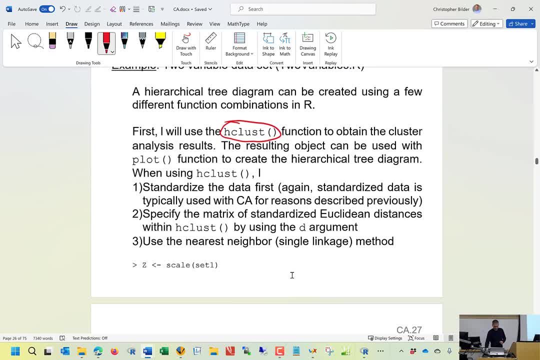 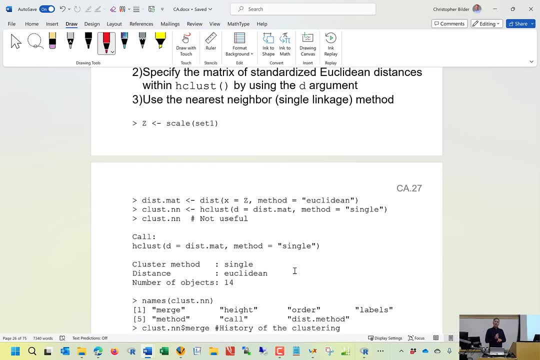 for HCLUS. So let's take a look at how this works when we actually use the nearest neighbor method. Remember? there's another name for it, called single linkage. That's going to pop up here, So let me actually just jump on over here to R. 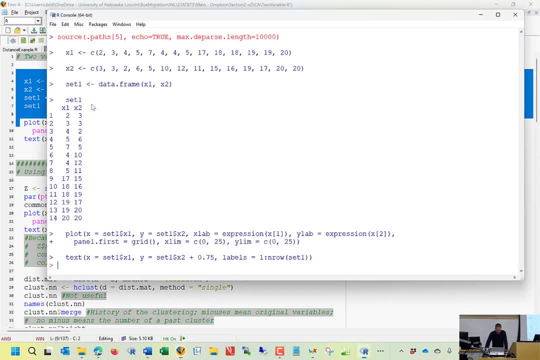 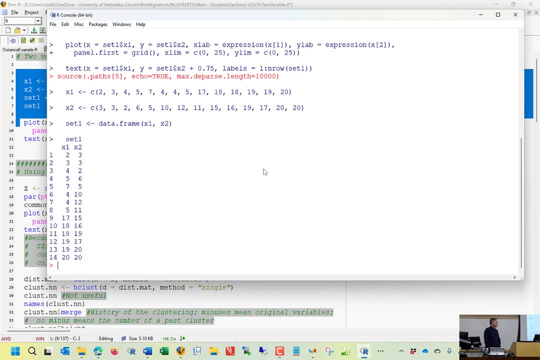 So here's my data. For some reason I didn't actually display it, I don't think- in the notes, So we have simply 14 observations. The variables are called X1 and X2.. I can do a plot of my data. 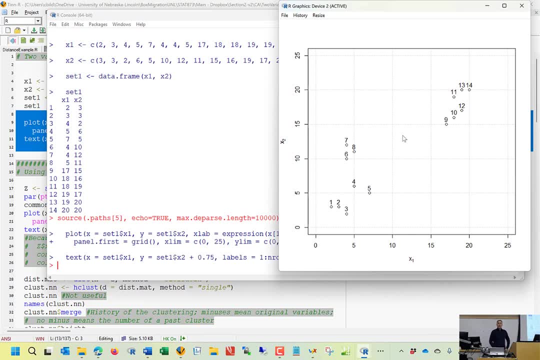 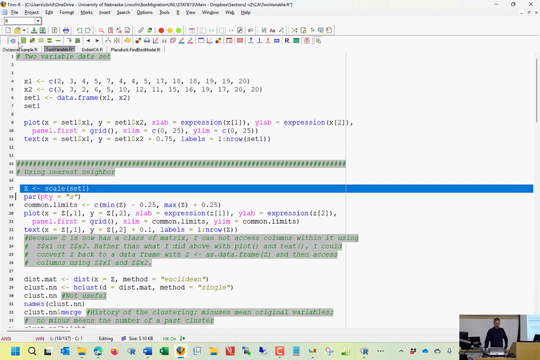 And here it is. So we definitely see some differences amongst these observations, But just again, remember we're going to actually be using the standardized values. So to standardize, remember we use the scale function. So I'm going to put that into an object called Z. 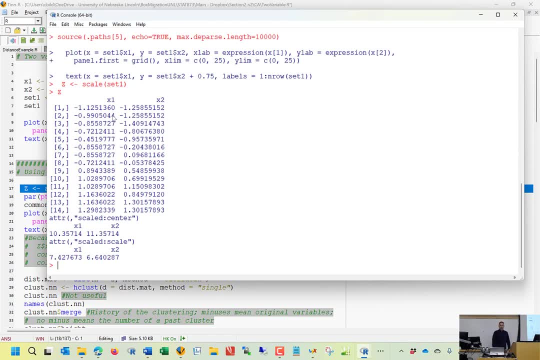 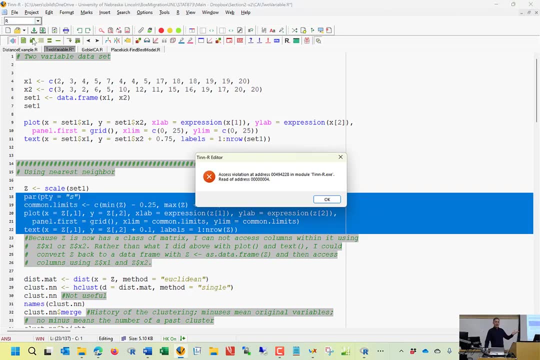 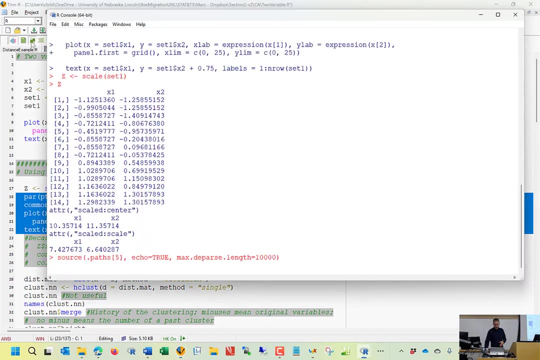 for the life of a better name. And there we go. Let's actually plot, then, the corresponding values of the corresponding data, just using the plot function for a scatter plot, then using the text function to identify corresponding observations, And this is what we get. 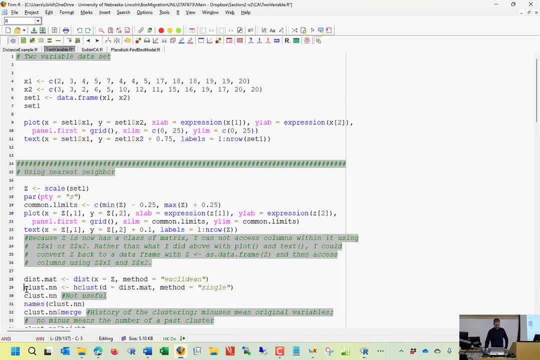 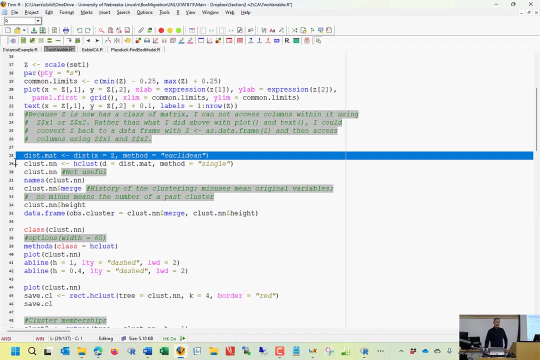 Okay, Again, we see some differences there. So the first, once I got my data, then I need to use the dist function to find all pairwise distances between the observations. Let's see how this works. Dist first argument is X. 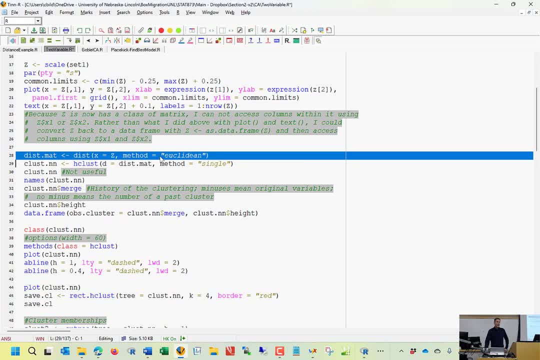 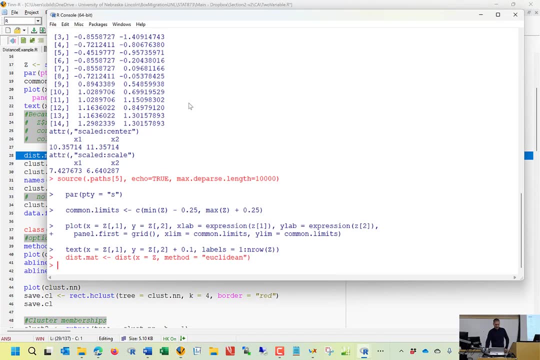 equal, put in your data, Then method equals Euclidean. So I'm going to use an Euclidean distance with standardized data. Then to the object. let's see, we'll call it distmat And we can see, here we have all these distances. 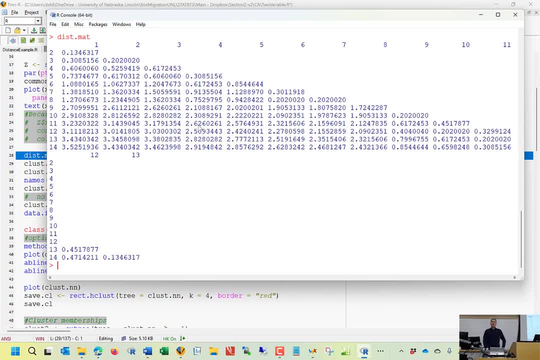 So now imagine if you have a very large data set, thousands of observations, maybe millions of observations. Finding all these pairwise differences could be quite time consuming, And so later in the cluster analysis section- we won't get to it today- we'll look at other methods. 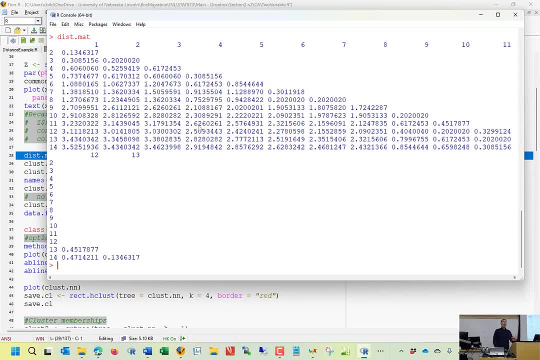 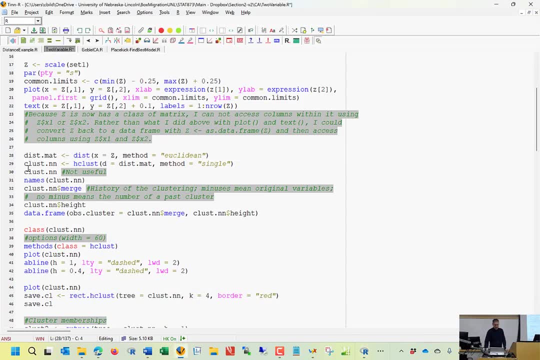 that avoid the need to find all pairwise distances, which can be very helpful when you have large data sets. Okay Now H plus D for distance. that's the first argument I put in my distance matrix and the method for cluster analysis I want to use. 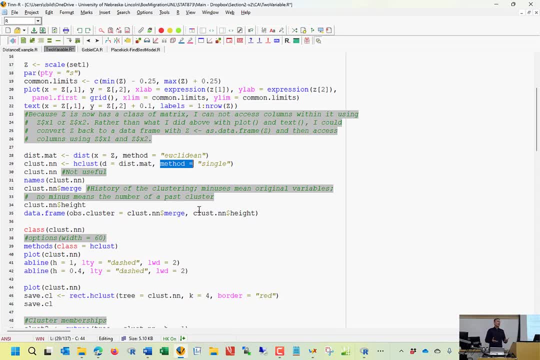 nearest neighbor, also known as single linkage. So R happens to use this alternative name. So I'm going to put the results into clusternn and then for nearest neighbor, and then we're going to just print off clusternn. This is what we get. 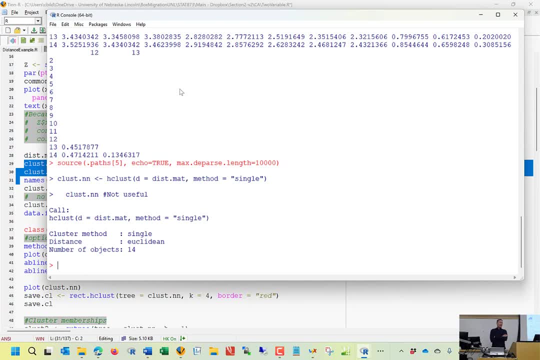 In the end it's not very descriptive at all, Not very helpful to us, But there is a lot of stuff that's actually stored in there. So clusternn is actually a list type of object in R and so to see the components of the list: 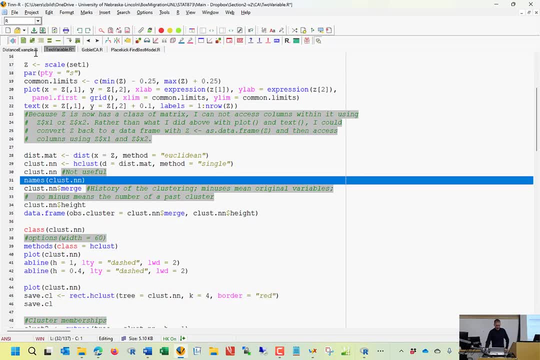 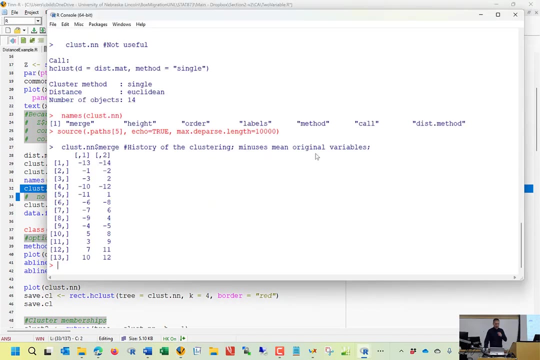 as we've done many times before, we say names clusternn and now we can see the stuff that's actually stored inside there. And in particular, if we do clusternn dollar sign merge, we get now the entire history of the clustering process. 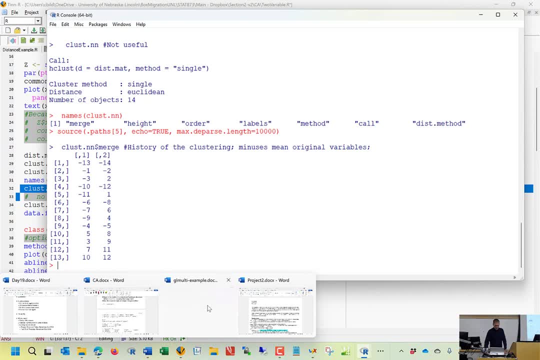 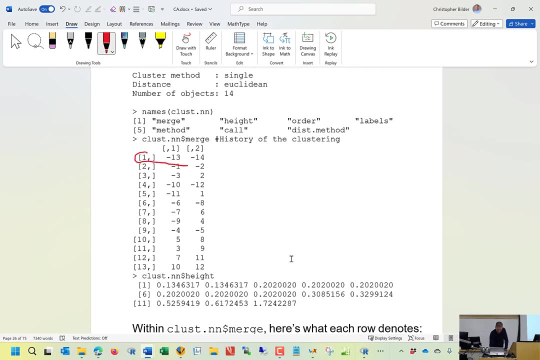 Let me jump back over here to Word. Okay, What this is saying is false. I start off with 14 clusters for the 14 observations, and observations 13 and 14 are joined together first. That's why you see 13 and 14 there. 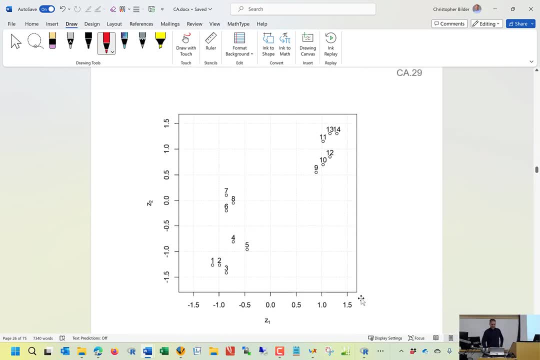 And if I actually look up at the plot, notice how this, you know, makes sense. 13 and 14 were joined together first. So that's my first set of clusters, And R will actually refer to this as cluster 1.. 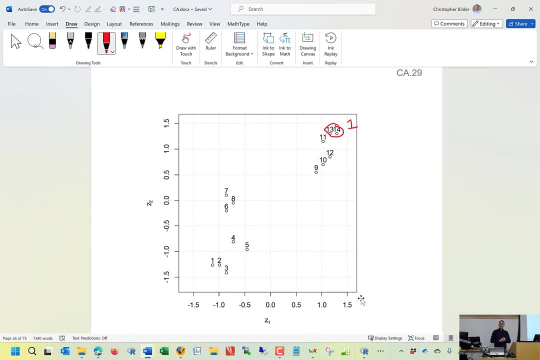 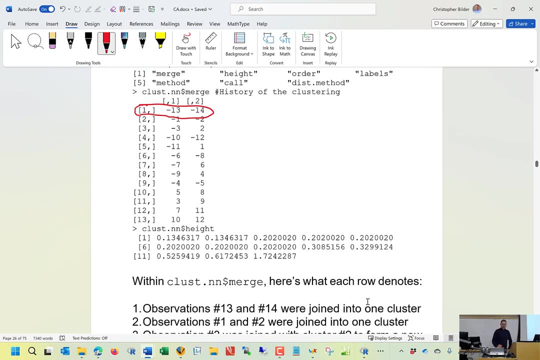 Yeah, just from looking at that, that looks like that's probably about the smallest distance between the two points, between any two points. So now I have 13 clusters and R needs to decide: well, what do I join next And what it decides to do. 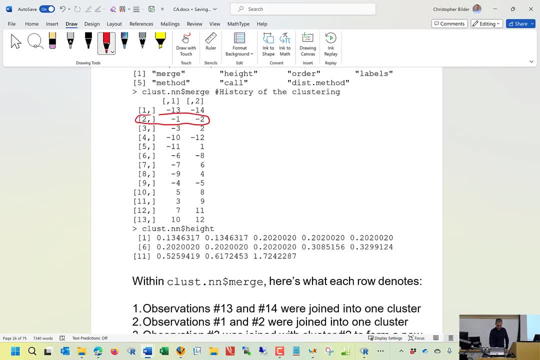 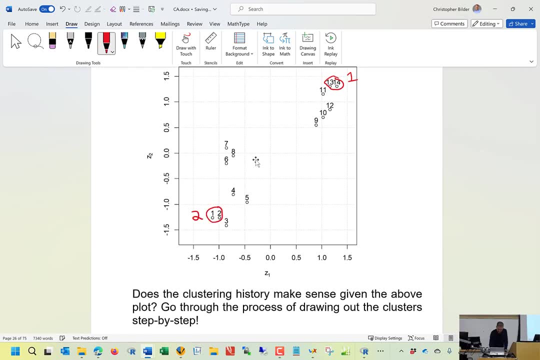 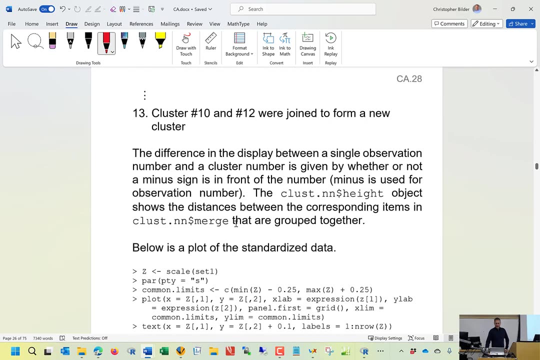 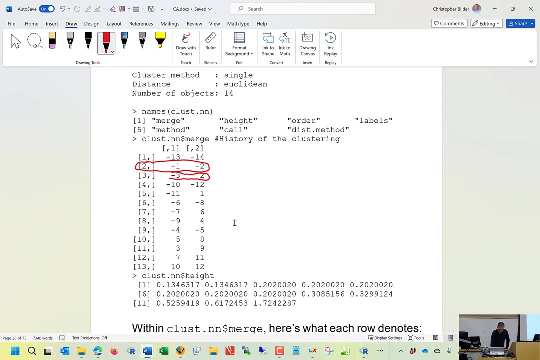 is actually join. observations 1 and 2 next Come here. So this is my second cluster that was joined. Again, that looks reasonable In terms of distances, what we can see. And then next it's going to join observation 3. 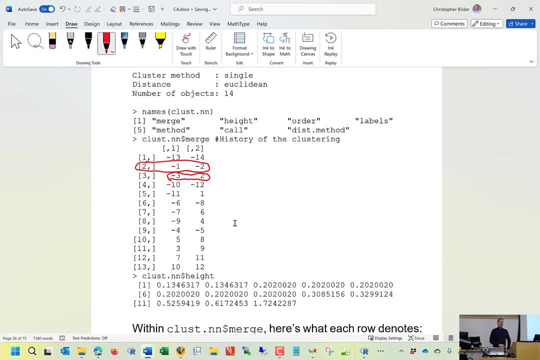 with cluster number 2.. So notice we have some numerical values that have a negative out in front and some have nothing out in front. Whenever you see a negative there- that's R's way of saying this- is an observation number. Whenever you see nothing out in front of that number. 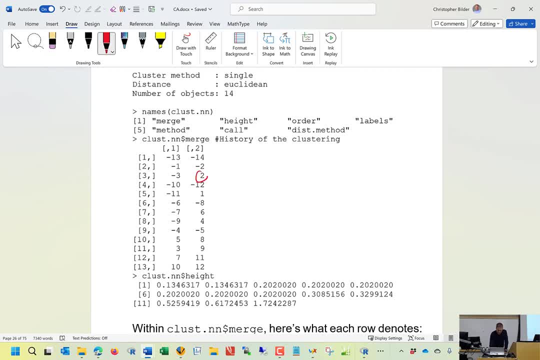 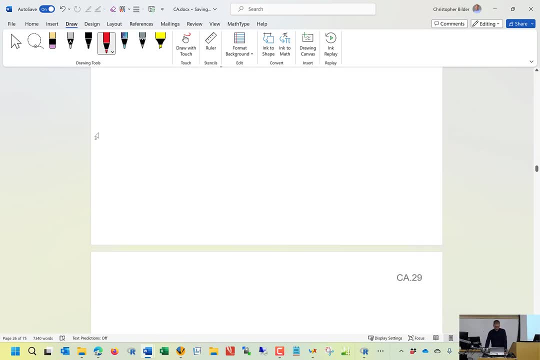 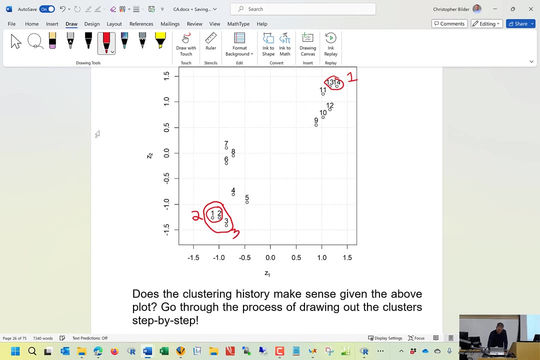 that means this 2 corresponds to cluster 2.. So now I can keep on drawing my lines here, And that's cluster number 3.. And that again seems to make sense. Remember how R is making a decision about what the distance is. 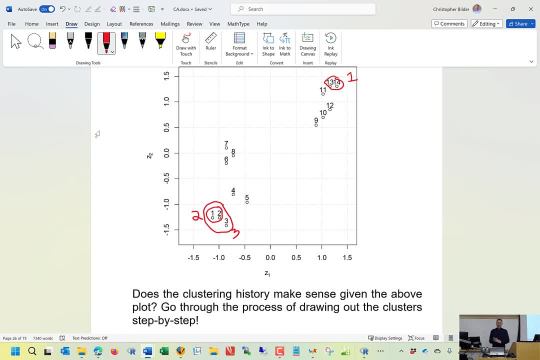 between cluster 2 and observation 3.. It's using the nearest neighbor, So it's taking this point and this point and it's finding the distance. Furthest neighbor would take 1 and 3.. Find that distance, But we're using nearest neighbor here. 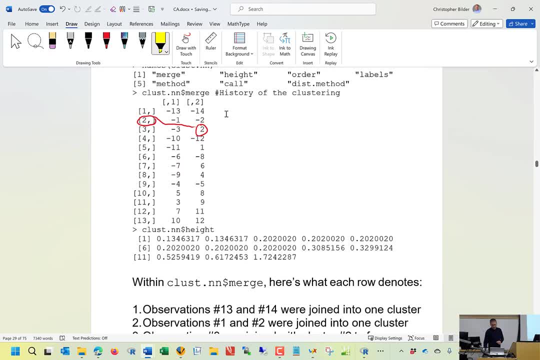 And so, on your own, I do urge you to do this, or I recommend that you do this. You know, actually keep on going through here, You know what's joining next, What's joining next, And actually draw it on the plot. 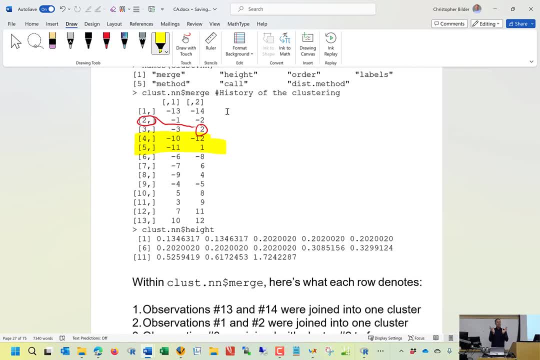 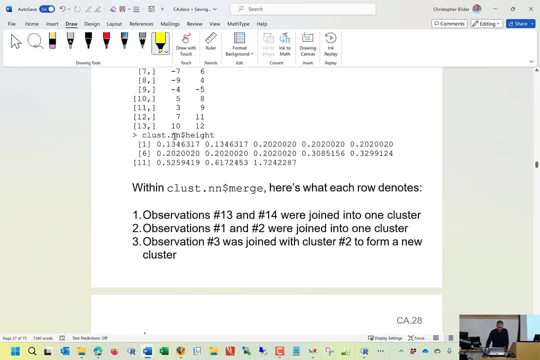 so that you can see the process, so that you can see- yeah, that makes sense- about what's actually occurring here. Next, we can look at the height component of clusterinit And this actually gives you the standardized Euclidean distance. So to do the 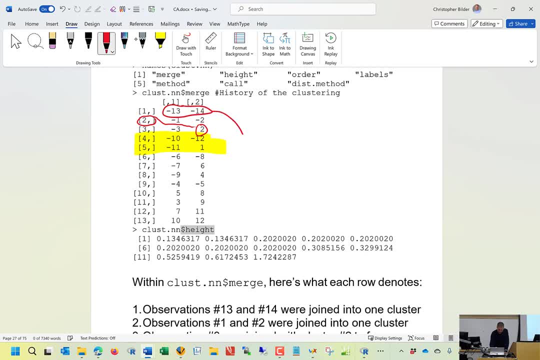 13 and 14, when that was formed, that was at a distance of 0.1346.. So why is this called height instead of distance? Well, when we actually show it on one of these hierarchical tree diagrams, how high you know, the joinings are shown. 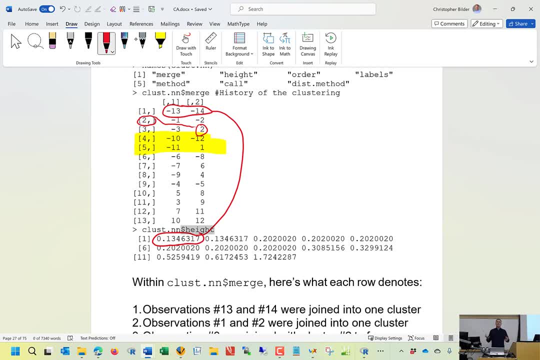 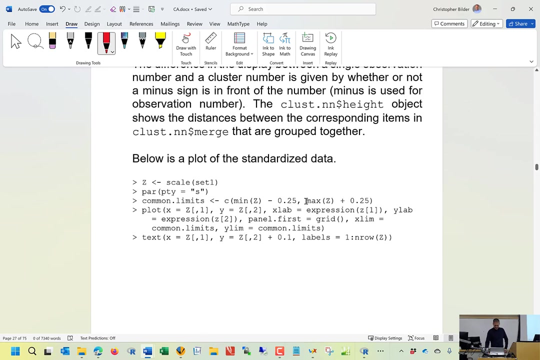 corresponds to distance, And so for some reason, height is used rather than distance as the name of the component. So notice also: between observation one and two it happens to have exactly the same distance. What is the scale of the distance? It's just the scale that. 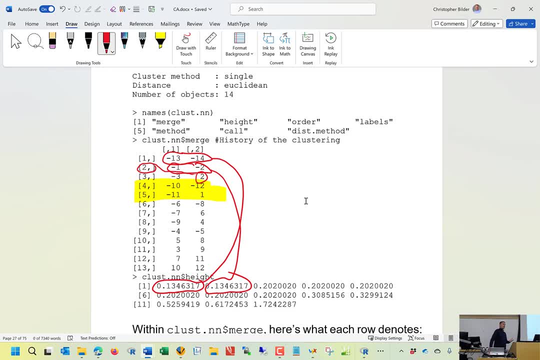 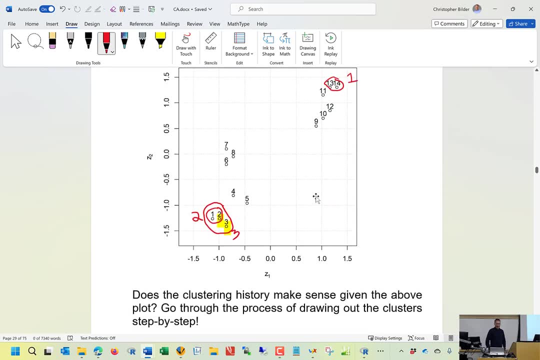 It would just simply be Euclidean distance between the actual observations. So you know, simply, you know, if you look at one of these plots and if you have a ruler that was appropriately scaled to what these axes are, it would be the ruler distance. 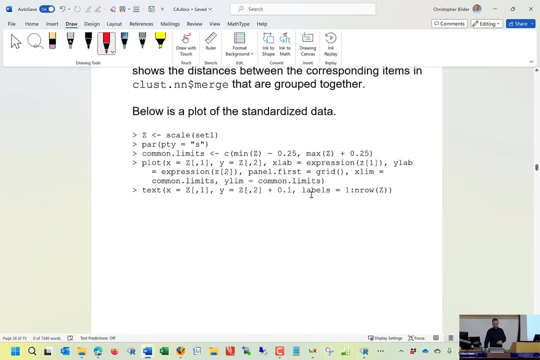 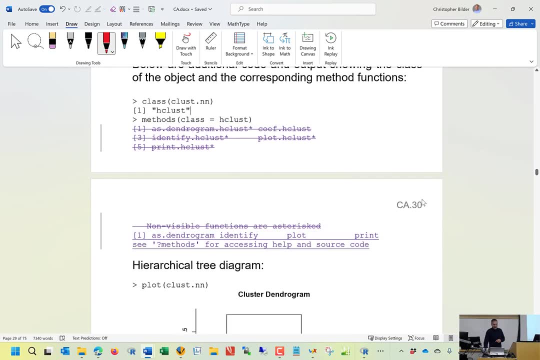 Okay, So you know I did the plot the normal way so you can take a look at that. Okay, Now you know, whenever you know you're approaching approach using a new, you know function: R. 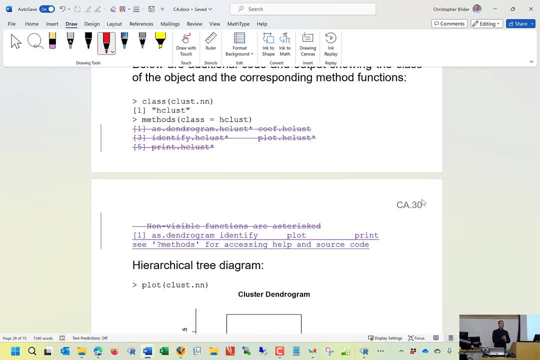 you know, I showed you how you know. it's always good to use the names function with it so you can see what's actually stored inside of it. You should also use the class function so you can see what is the class of the corresponding object. 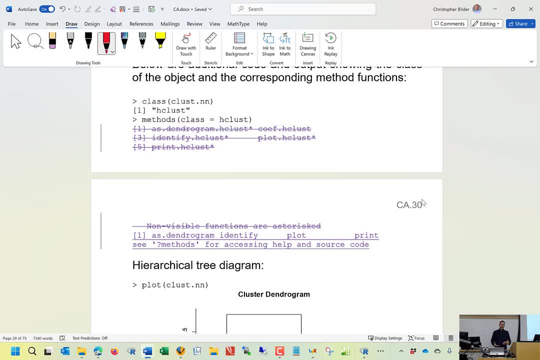 And it just so happens to have the exact same name as the function name. It doesn't have to, And general applications are, but very often programmers will make that decision and do that, And so if I did, methods class equal h plus. unfortunately, this is an old version. 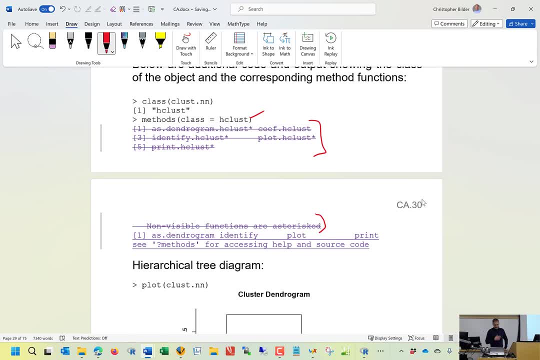 of what would have happened when I for a previous class that I taught a few years ago. what it looks like now is what it looks like here, And we can see that we have a few different generic functions that we can use with the results from each class. 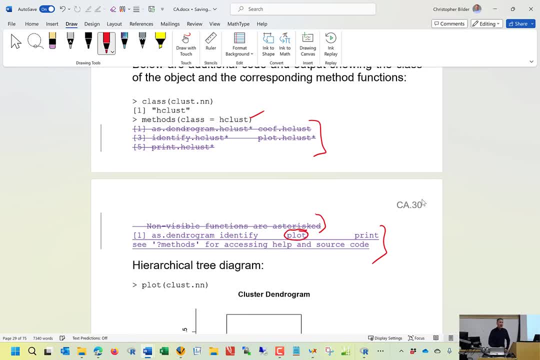 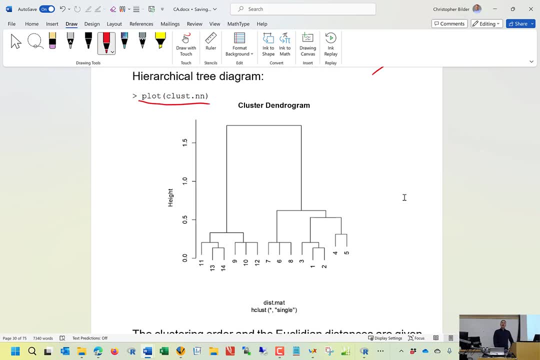 We will focus typically on just this plot function here, because when I use plot with the results from each class, this is when I get my hierarchical tree diagram, or what R calls a cluster dendrogram. That's not the standard name. Let me make this a little bigger. 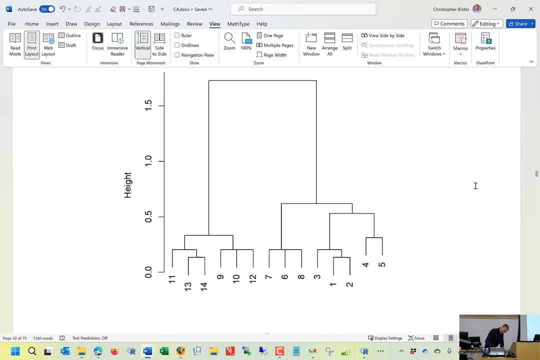 And so on. the y-axis R calls it height. This is what I was referring to before as distance. On the x-axis, we have the observation number, And so remember what was joined together first: 13 and 14.. So we see 13 and 14 here. 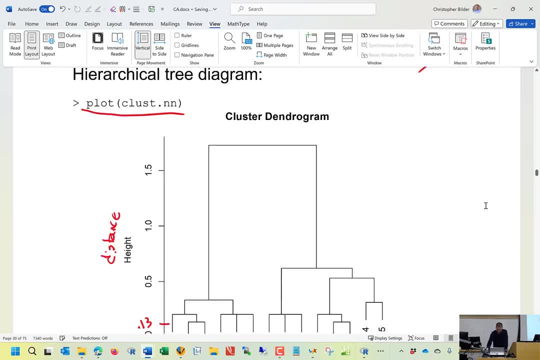 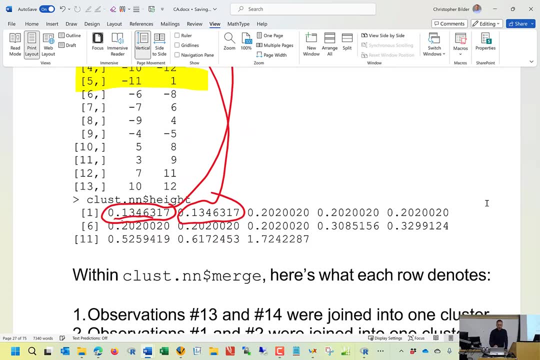 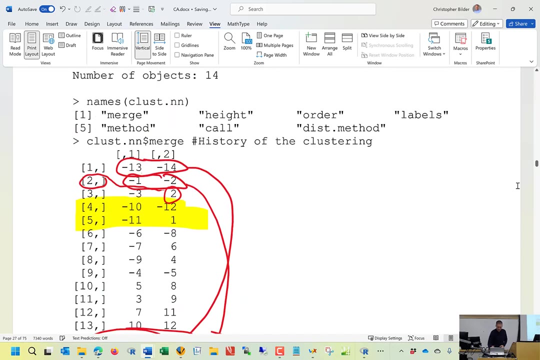 It was at a distance of 0.13, I believe, Yeah, 0.1346.. And so, essentially, what R does to do this plot? it extracts these distances, these heights. It also extracts what's in merge and then uses that to create the plot. 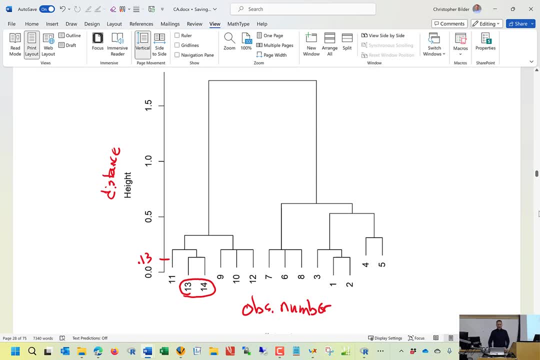 Now notice that these numbers that you see here are not in numerical order, And the reason being is because you know it depends upon where the observation numbers, observations are on the plot. You know it wouldn't make sense to put, let's say, 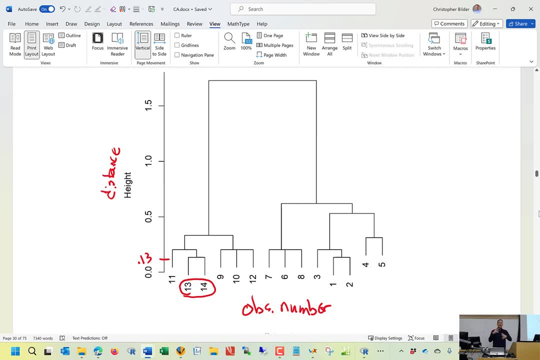 the way that I drew the plot so that the numbers were often near each other. But you know it nicely, tries to arrange it so that you don't have lines going all over the place, And so the observations are close together. They're going to be joined together more. 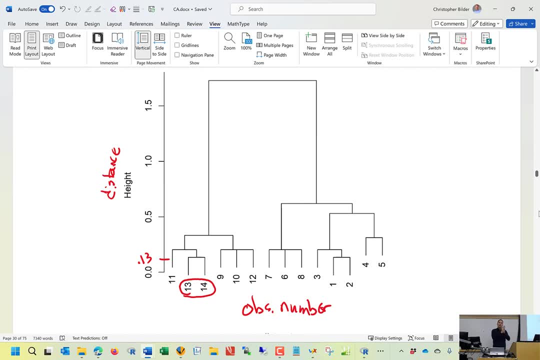 more quickly in the process. So the numbers are just arranged so that these observations are going to be close together on that x-axis. Yes, So here, depending on this plot, so we can say that we have two big clusters or we just go with the small ones. 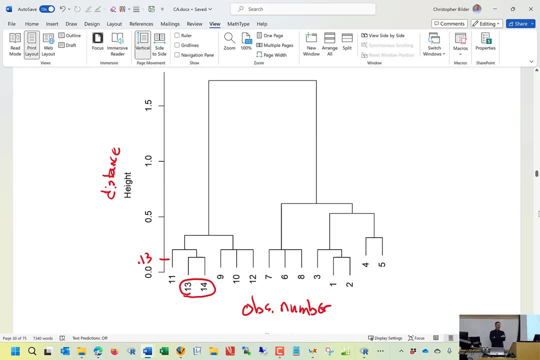 Yeah, And so that's what you're getting at. You're foreshadowing where I was going. So yeah, thank you, And so what we see. so again, remember, we're looking at when the distances between clusters, when a distance is, let's say, 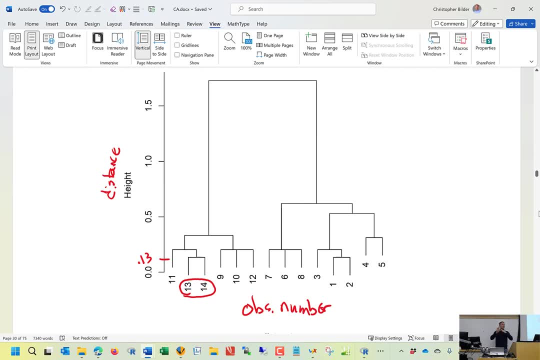 much bigger than, relatively, what the distances were before. And so we can see that when I go from, let's say, two clusters- so maybe I have this here- when I have two clusters now, that distance becomes really, really big In fact. let me just 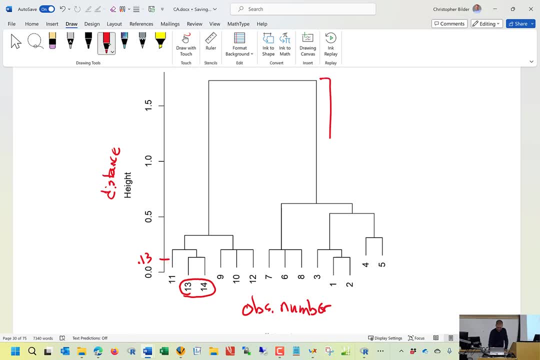 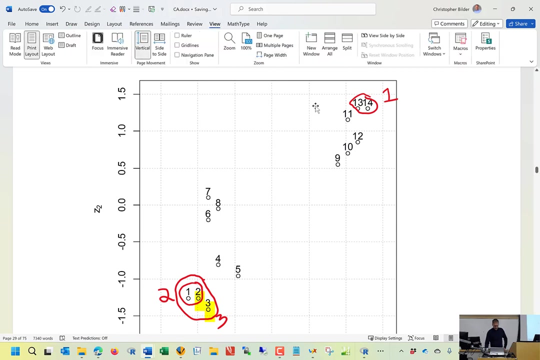 let me draw it a different way. So I'm looking at this distance: relatively to what we had before, That's huge, And so because of that I probably want to stop, which is two clusters, And if we go back here now, let me make that smaller. 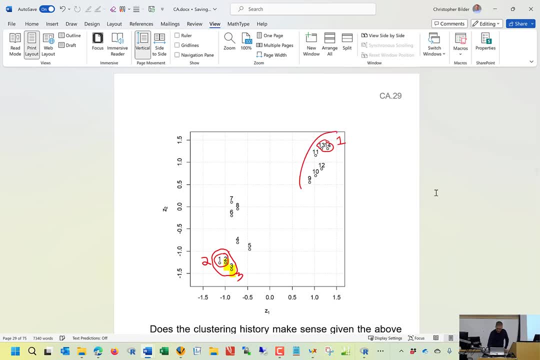 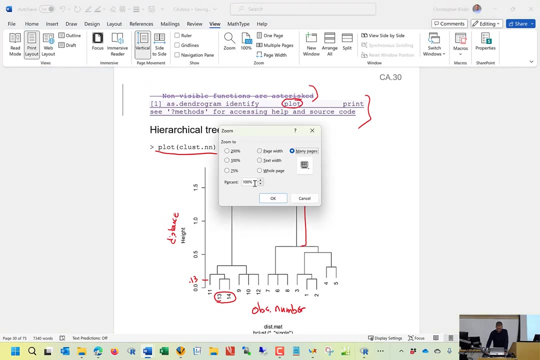 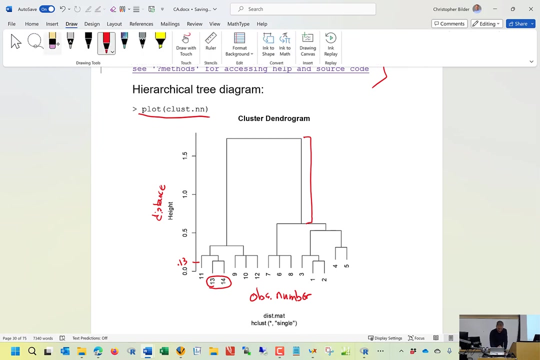 Yeah, that should make sense. You know, what we see here is perhaps two clusters, So let me come back here. I'm going to make this bigger again. So what people often do when they look at one of these plots- and you can see how this is kind of 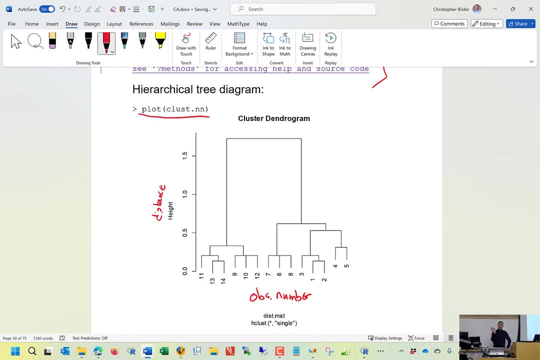 a little bit of a judgment call, because there's other possibilities for the number of clusters too in this case. But what people will do is, once one of these plots are drawn, is that they'll look to see. where do I see these large distances? 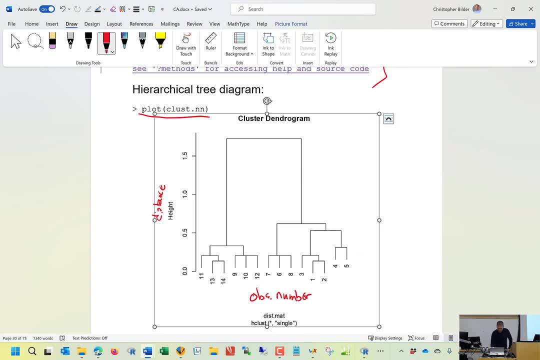 Where do they pop up? And we can see. from going from two to one cluster, we see that distance. So what people will do is typically somewhere on the y-axis, and it doesn't really matter where, they'll just simply draw a line across there. 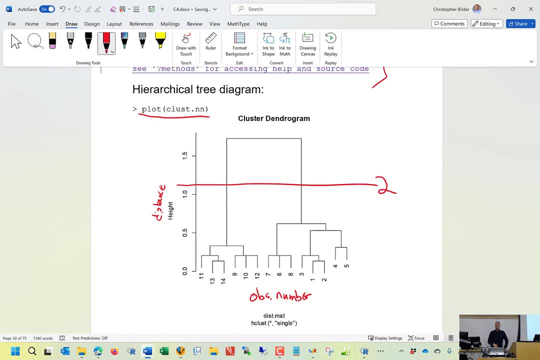 Maybe even we'll label it with how many clusters. Notice how that horizontal line that I draw intersected the branches you could say of the tree twice. I have two clusters Now. there are potentially other places where I could draw that line too. 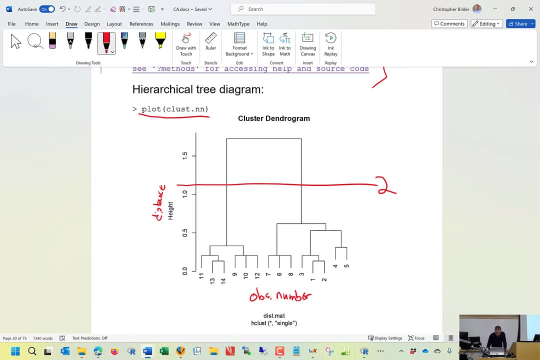 that would make sense. So, for example, look at, this is going to be. actually I'm going to just draw like a little dotted line over here. It's meant to be a horizontal line, even though it's not. So look at when I do this connection here. 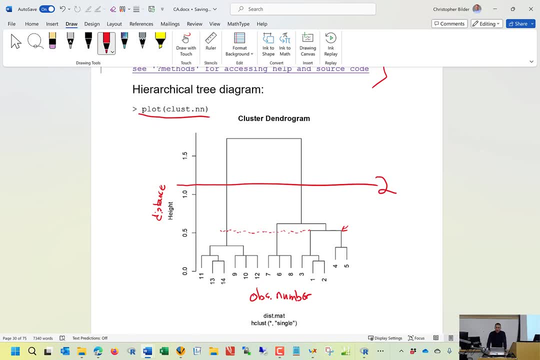 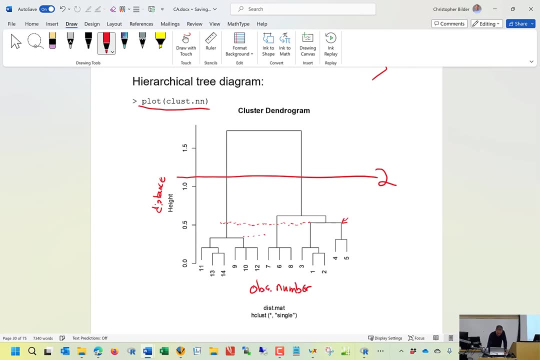 between one, two, three and four and five. Compare that to when I made the connection between 11, 13,, 14,, 10, 11, 12.. Look at this distance here. So this is in succession. 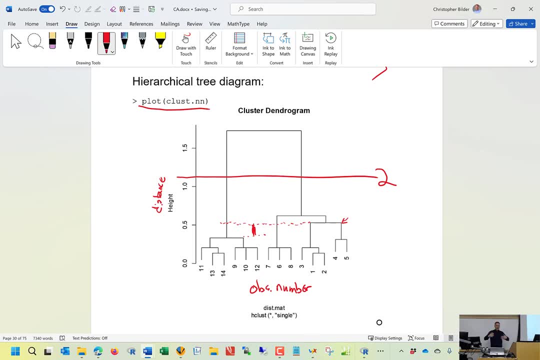 Remember, we're doing this in a hierarchical manner. I would connect these two, and then the next set of connections was between these two clusters, And so that's what I'm looking at. in terms of the distance between successive joining of clusters, I am not. 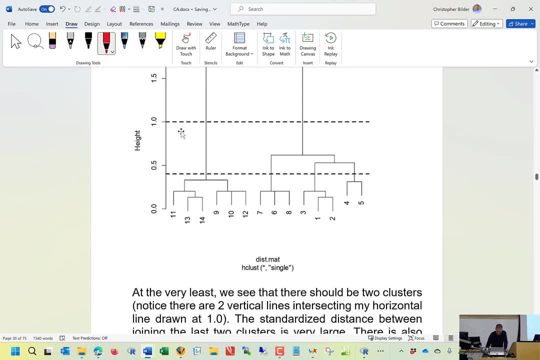 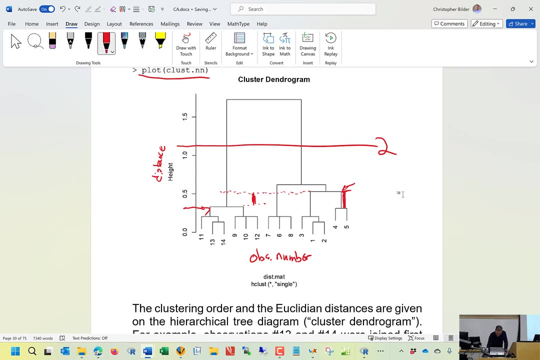 oops, where was I? There we go. I am not focusing on this distance, Because this distance here is larger relative to what I have been doing. I would draw a line across and that would correspond to, let's see, one, two, three, four clusters. 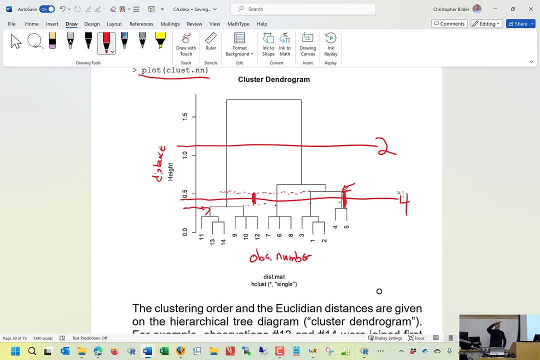 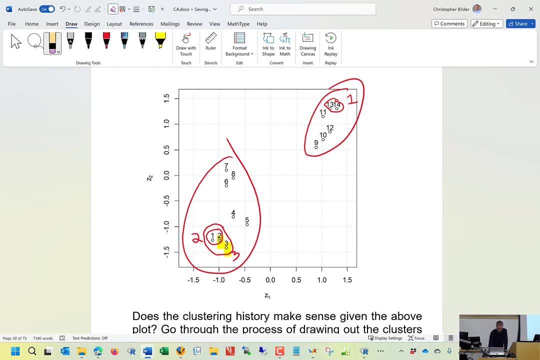 Because of the number of times that that horizontal line intersects the branches of the tree. Now let's look at what that would look like here. Let me do some erasing. That would be this, this, this: Let me just double check that. 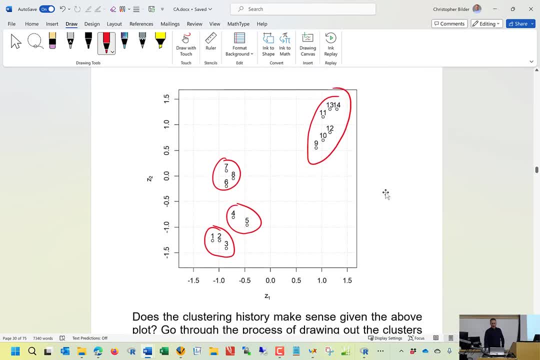 Yep, I would have these four clusters And again, that makes some sense relative to what we see in this plot. And once again, you know, in other applications you typically have many more variables than this And so you are not going to be able to see this. 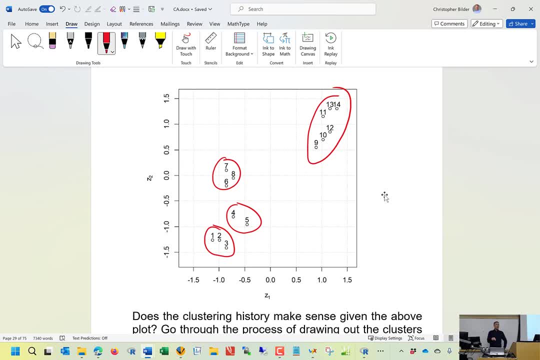 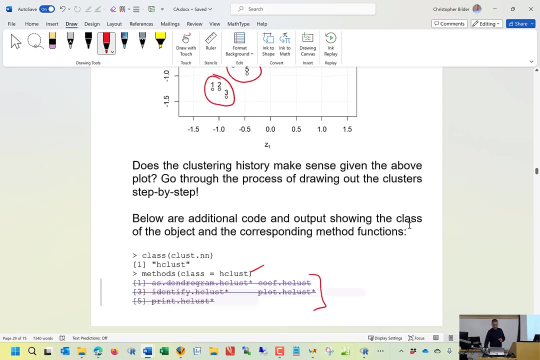 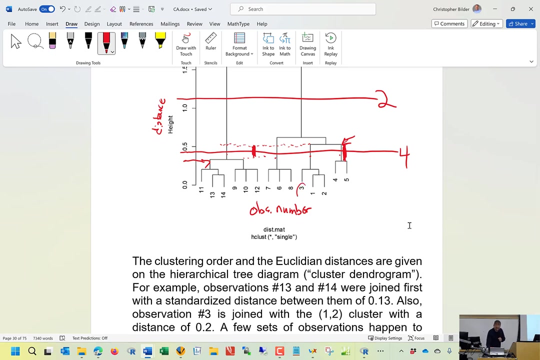 in this particular kind of a plot. Instead, you will have to rely on the tree diagram alone, And so this makes some sense to use four clusters. Now let's see here. So look what was joined next, and after that, Essentially, it was these points: 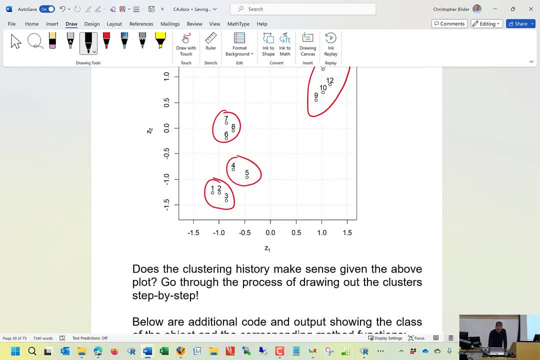 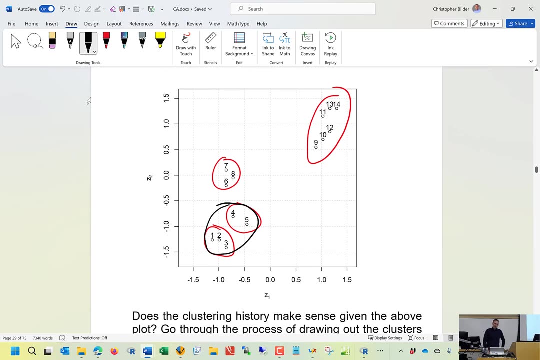 In other words, let me do this: These are joined next. Relative to cluster analysis, that makes sense for those to be joined next. Those seem to be kind of the closest of the remaining ones, But perhaps that's just going too far. 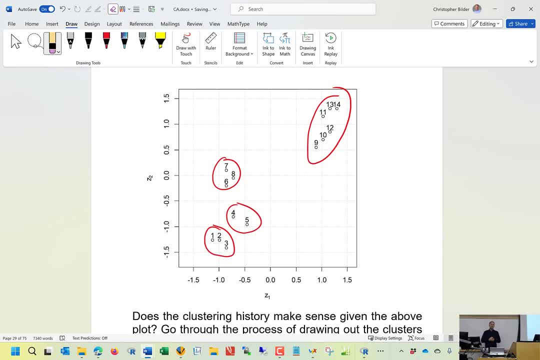 So we do see some separation there, But also you can see here again that you know this is somewhat. there's probably more than one answer here, And so, like on a test or a project, I want you to justify your choice. 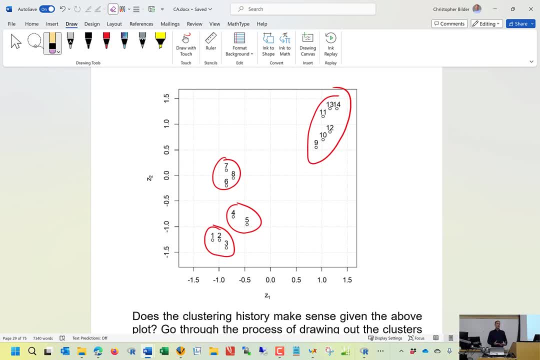 eventually, at some point where you might have to actually choose the number of clusters, And you go to that higher tree diagram and that's how you make that choice. Now, shortly, you're going to see some other methods that I'm going to use as well. 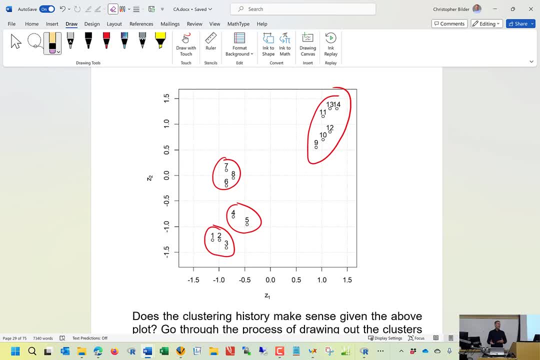 to justify the number of clusters too. When you start off with that tree diagram you can say: I can see two and four clusters are justified because the distances between successive hierarchical joins. we see a jump in it. We see it relative to what we've done before. 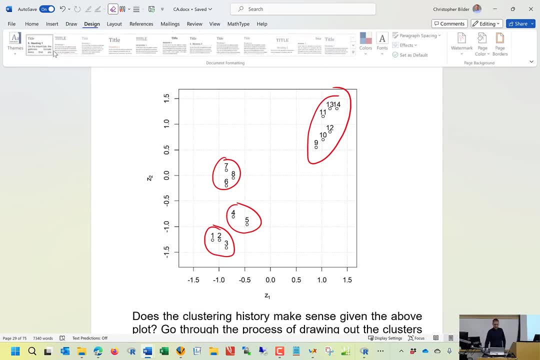 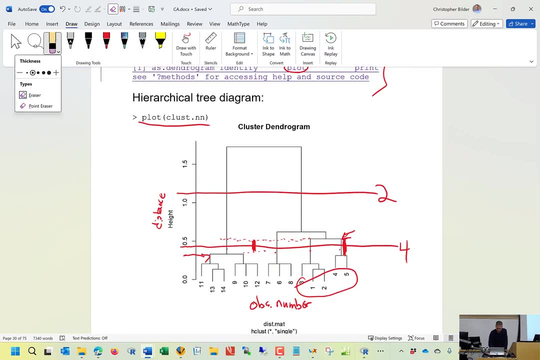 we see some differences. Now notice here, I am not. I am not. let me do a different color here, since it's not. I am not drawing a line right there, because we can see that that distance there is actually even smaller than the previous distance that we just had. 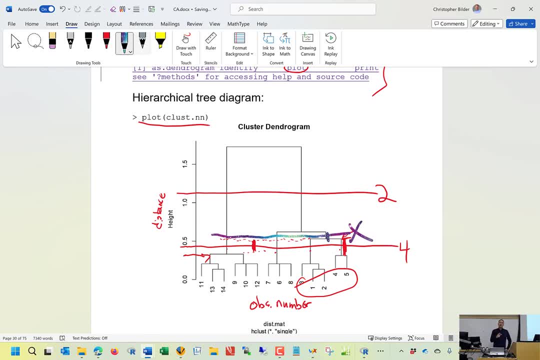 when we were trying to choose the number of clusters. That distance is smaller. So no, I'm not going to, I'm not going to draw my line there and say that I have three clusters for this particular method. Now some other method might say: 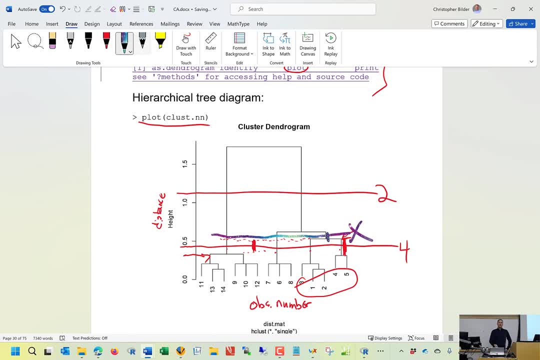 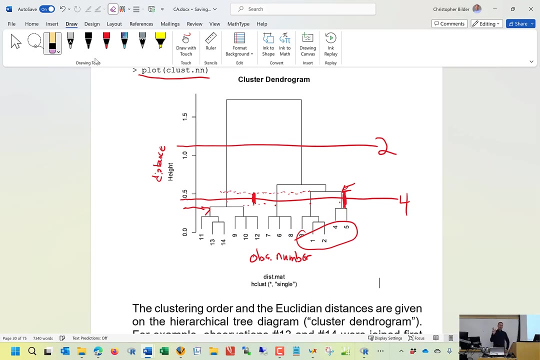 yes, three clusters is justified, but not for this method. So just to emphasize again, because this is sometimes where students get get mixed up: When I was making that decision about getting four clusters, I was not looking at that distance. 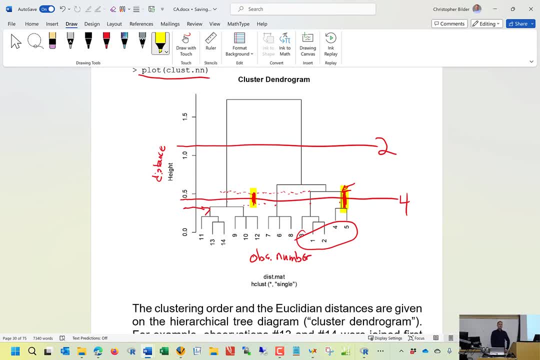 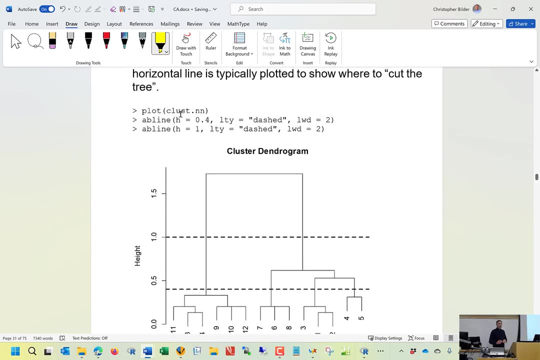 I was looking at this distance, Even though they were for different areas of that tree diagram. I'm looking at successive points, So you can see that I I like to draw those. well, anybody who's doing this likes to draw those vertical lines. 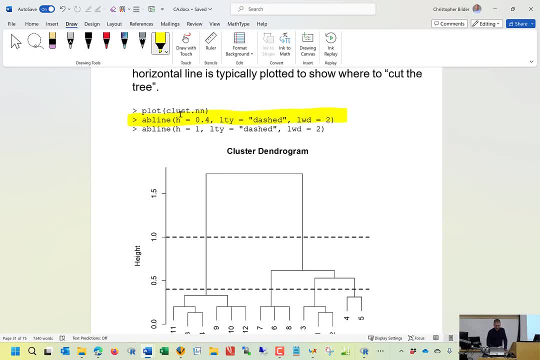 And so there's an easy way that you can do that in R. It is just to use the avline function. The h argument means horizontal line, And basically you just need to draw the horizontal line at a particular location. In this case, 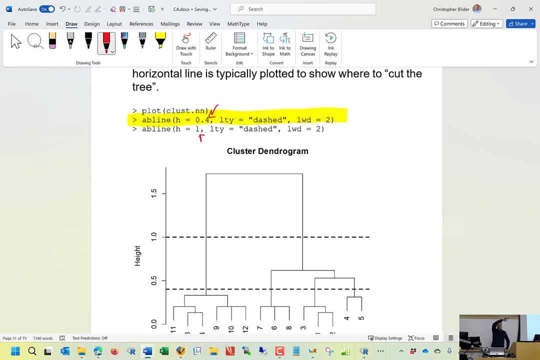 I chose point four. I chose one. I'm going to intersect the tree diagram in the correct spot, So I could have simply chosen maybe one point two. I could have done that. I could have chosen point nine. The key is it just needs to be somewhere. 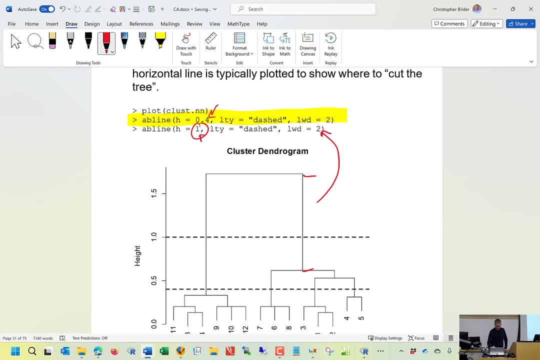 between here and here for this one there. Line type: equal dash. I use a dash line to help differentiate it from the solid lines that you see on the plot. We're ready for the diagram And also line width two to make it stand out. 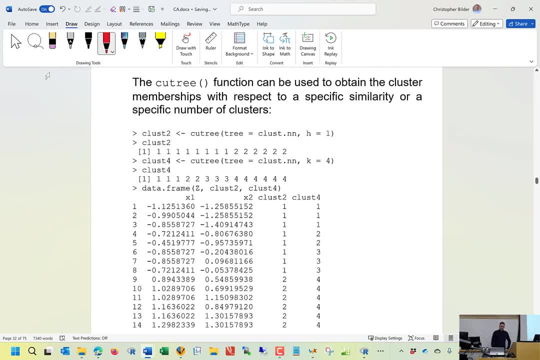 Now there's also some functions that are available to help you see which observations are in which cluster. This is going to be very helpful for us when we do some other plots, And we can use a function called cut tree. Notice, it's actually spelled. 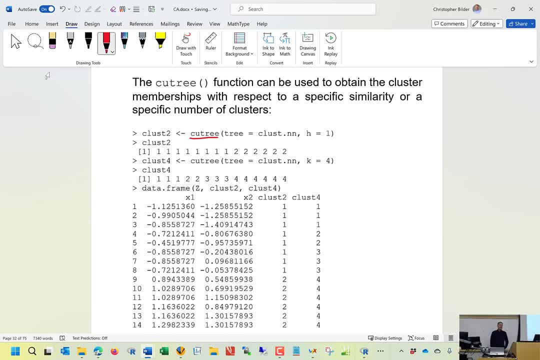 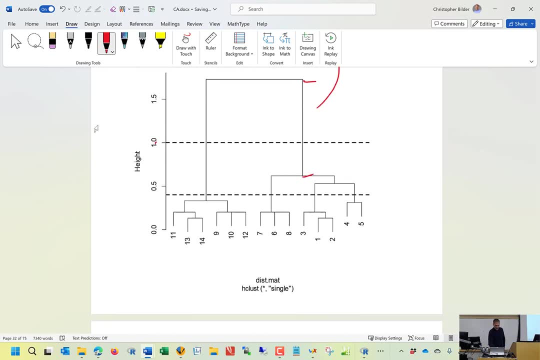 c? u tree, But it's meant to mean I am cutting the tree. In other words, I am simply drawing one of those lines: I am cutting the tree. I don't know why it's not c? u t and then t r e, e. 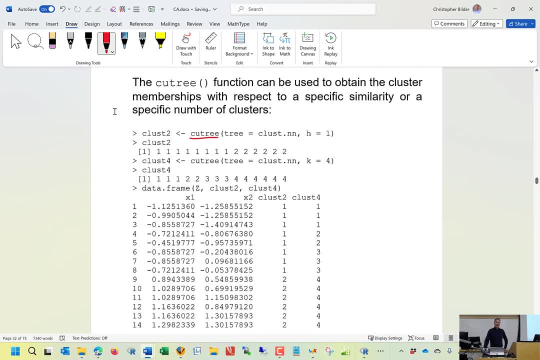 but I'm just going to pronounce it as it is: cut tree, And so what I can do for the argument tree is put in the results from each cluster And then say: where do I want to cut the tree at? Where do I want that line to be at? 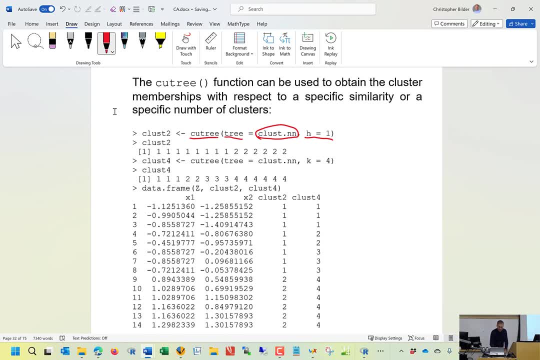 Let's say F1. And then what's going to be returned is that all the observations are going to be given a cluster number. So actually observations 1 through 8 are in cluster 1.. Observations 9 through 14 are in cluster 2.. 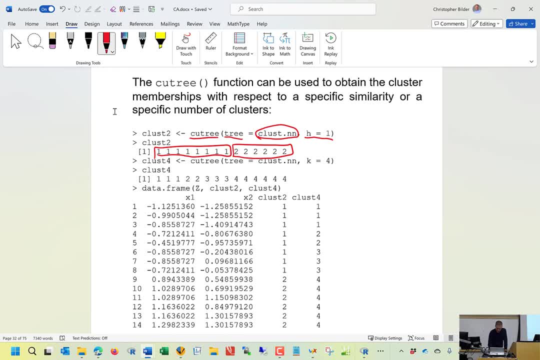 I can also use cut tree this way, where if I use a k argument, that shows how many clusters do I want, So if I choose four clusters, then we can see observations 1 through 3 are in cluster 1.. I can form in a data frame. 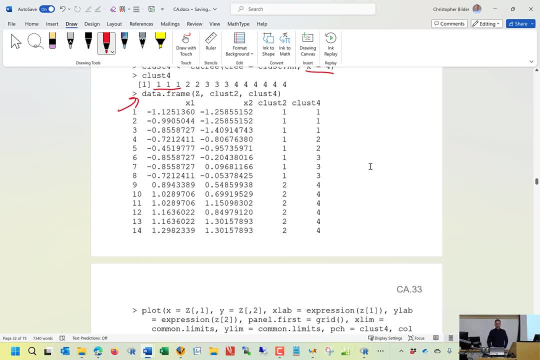 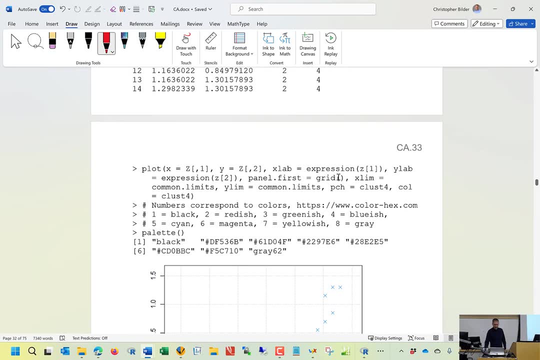 with this information so that I can actually see the observations with the corresponding cluster number, And then this can be very helpful then to actually do a plot. So I use a do a scatter plot where I have the plotting character, so the PCH argument. 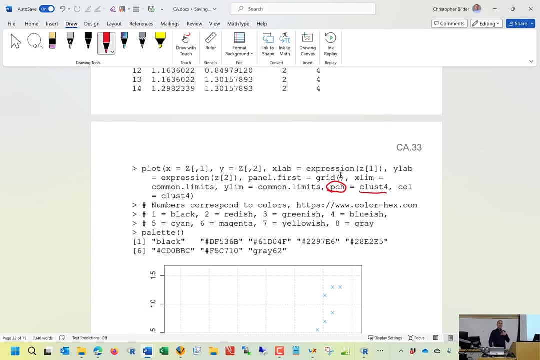 corresponds to these clusters And I've chosen to work with the four cluster set. And also, if I use COL, for color R automatically designates particular numbers with a set of colors Up to eight different colors, And so color 1 is black. 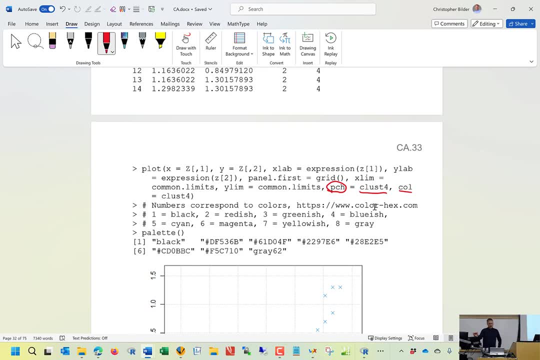 color 2 is a reddish color, color 3 is a greenish color, and so on, So that when I say col equal class 4, which are numbers in there, I have different colors for the different clusters. And so now you can see. 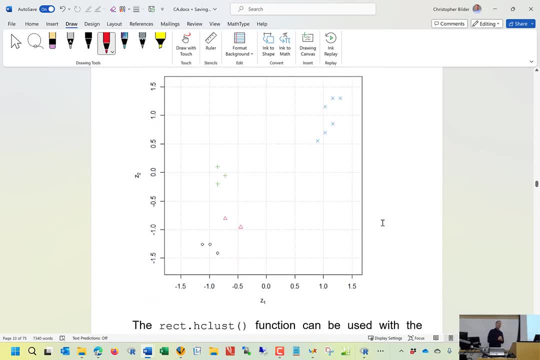 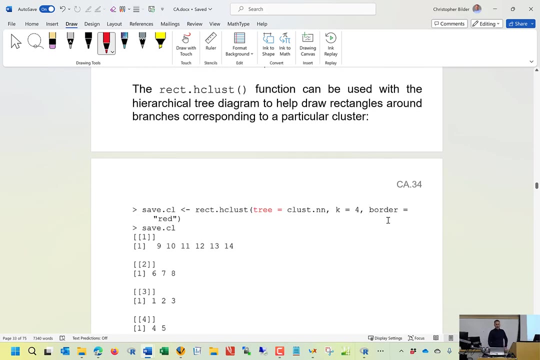 this is what those clusters look like. when I have four clusters, Everything is uniquely identified or not uniquely identified. the clusters are uniquely identified. right: The color implies the color. There's also a function called rect, dot h plus Rect stands for rectangle. 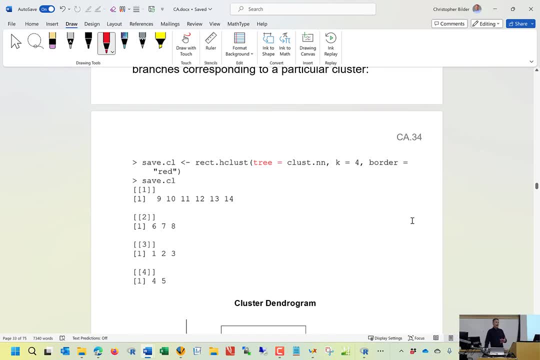 And this is going to help me with my hierarchical tree diagram also to identify the different clusters. So if I say, after I've actually drawn a hierarchical tree diagram, I use this function and say tree equals, again the results for each cluster. 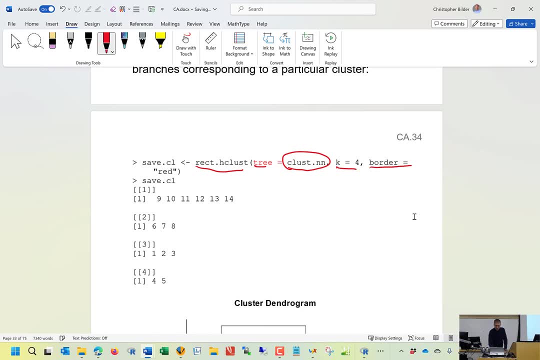 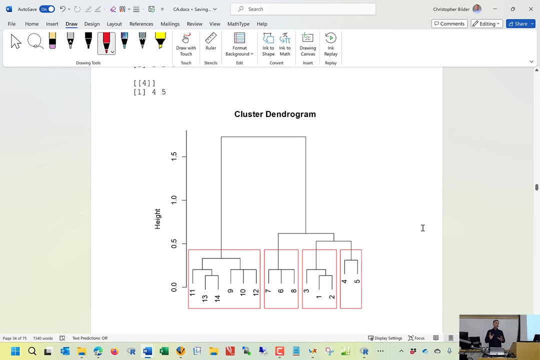 I want four clusters and I want to draw like a rectangle in red around the actual clusters. what's returned to me is again the different clusters and what's actually automatically drawn on the plot is a rectangle around those clusters. Just to help you see. 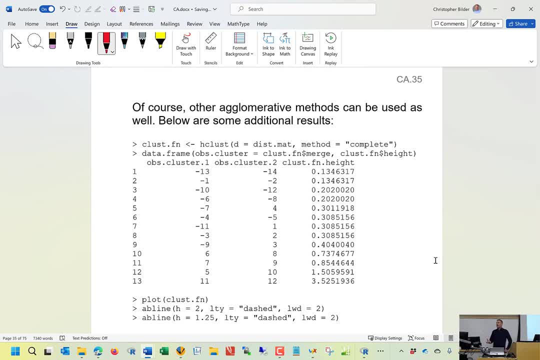 Okay. Well, what if I chose to use some other clustering method? Would I get the same results? I think the answer is actually no, And very frequently in actual applications it's going to be no. So let's say I want to use the first name method. 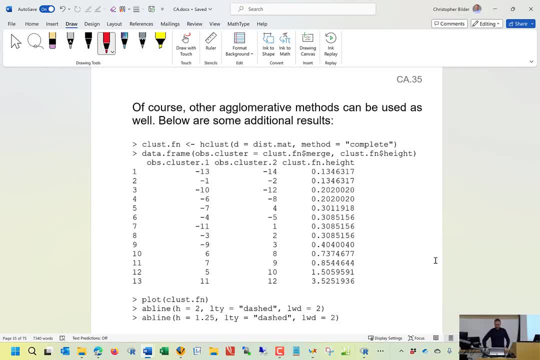 Remember another name, for it is complete linkage, and R uses this other name to represent the actual method of each cluster. So again, each cluster, my distance matrix method, equal, complete. I put the results into clusterfn. fn, saved for furthest neighbor. 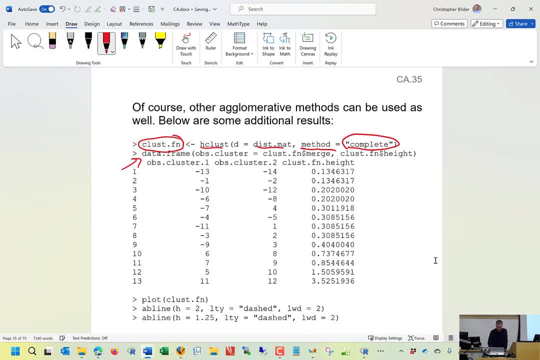 I can put it all in a data frame so that I can see the actual merging process, I can see the actual distances, the heights of these clusters, and so we can see once again that R first puts together observations 13 and 14,. 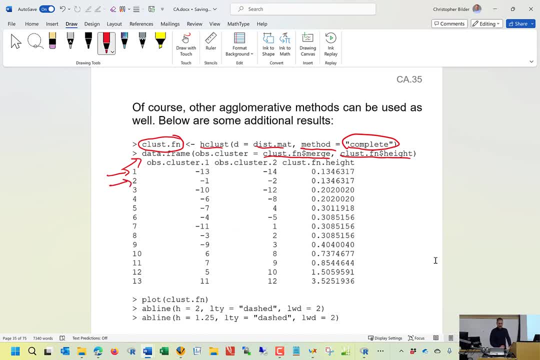 next it does 1 and 2, but now we have a change from what we have with nearest neighbor, where before 1,, 2, and 3 were joined together. now we have 10 and 12 joined together. Let's look at one of these plots. 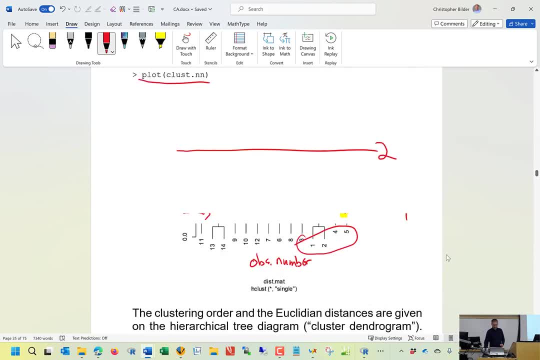 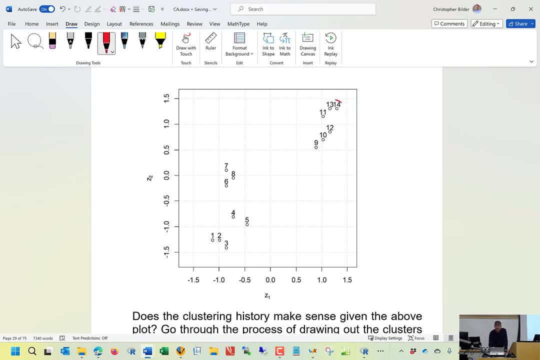 from the plot of the data to see if it makes sense. So again, 13 and 14 is cluster 1,, 1 and 2 is cluster 2, and now I forget what was joined next, 10 and 12.. 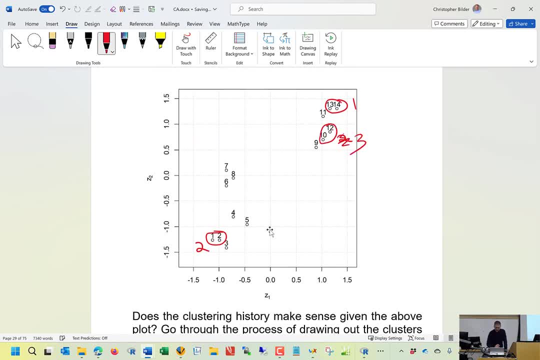 10 and 12 is joined. oops, it should be 30. Okay, Here I guess it makes sense Again. think about what furthest neighbor means. You know, nearest neighbor joined 3 with 1 and 2,. 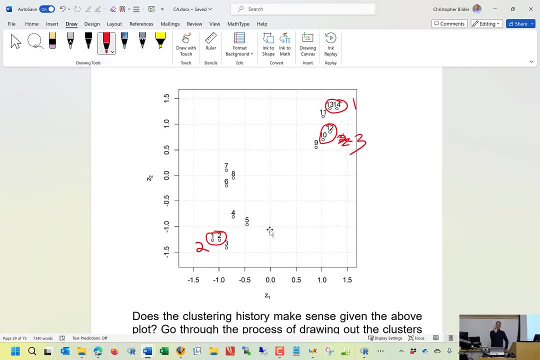 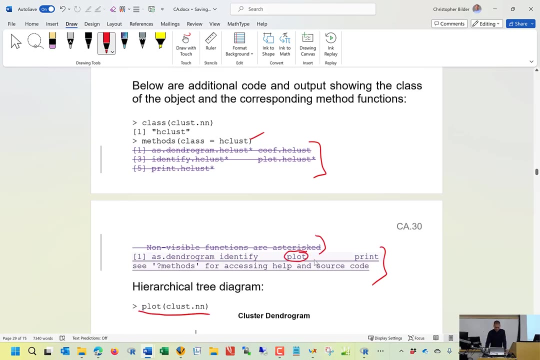 but now we can see that furthest neighbor, that distance between the 1, 2 cluster and 3 has greatly grown, because now I'm looking at this distance here That's bigger than what it was for 2 and 3.. 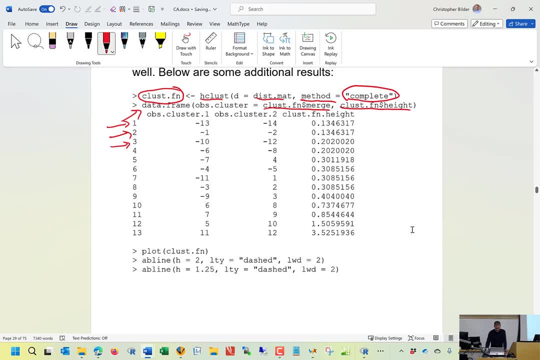 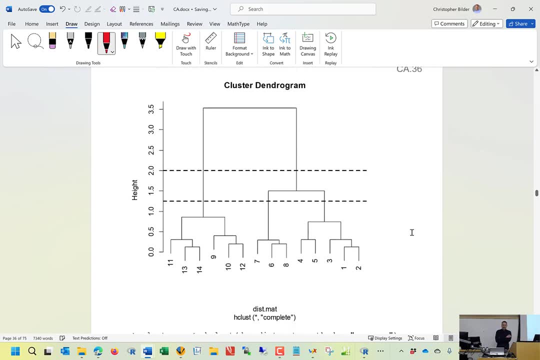 Okay, So I can do the hierarchical trigonometry. This is the diagram and this is what I get. Notice: 2 clusters make sense again, but now 3 clusters make sense, To emphasize my point, because again, this is a place where students 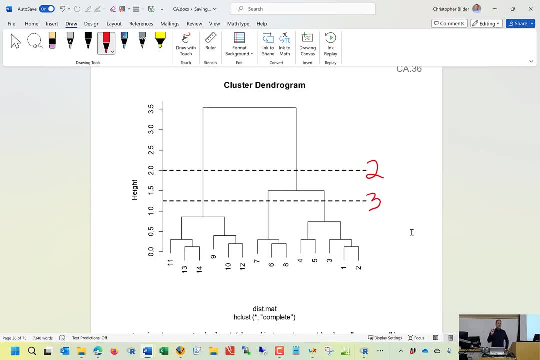 often make a mistake. When I chose 3 clusters here, I was not looking at this distance here. I was not looking at that. Rather, what I was looking at is the distance between successive joins. Oops, So I was looking at here. 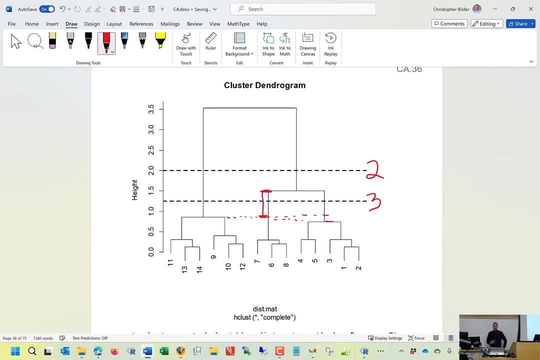 to here. That's the thing. That's what I was looking at. That distance seems to be larger than what we've just recently had, Much larger, Kind of much larger, really- What we just recently had during this hierarchical clustering process. 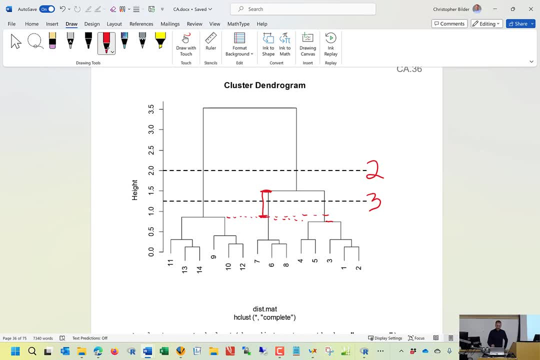 In other words, when I say what we just had, I'm looking at these distances, Definitely for 2, that makes sense, You know, to go from 3 to 4 clusters. yeah, it's not as big of a distance. 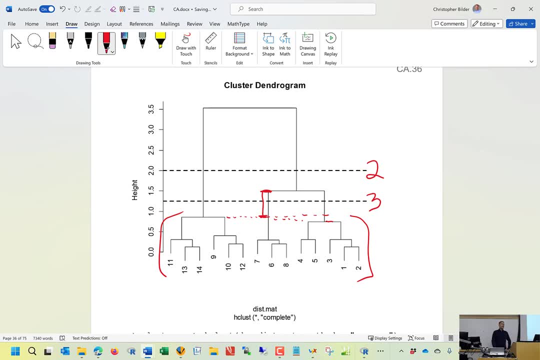 as what we've seen from going from 3 to 2.. But you know, if you go from 3 to 4 clusters, yeah, it's not as big of a distance as what we've seen from going from 3 to 2.. 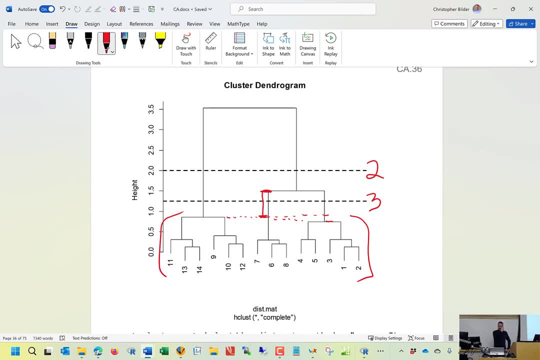 But you know, it's not as big of a distance as what we've seen from going from 3 to 2.. But it is larger. Notice how 4 clusters would not make sense here, Because if I were to draw a line going across, 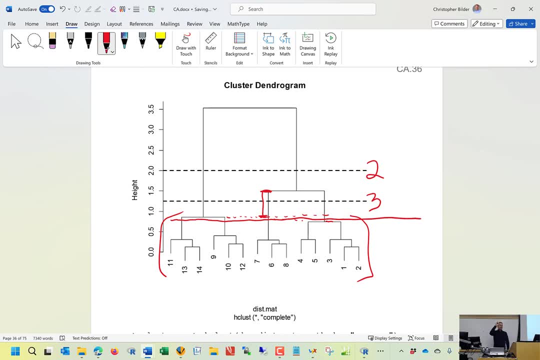 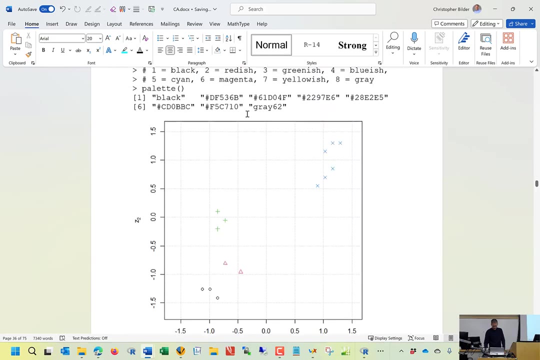 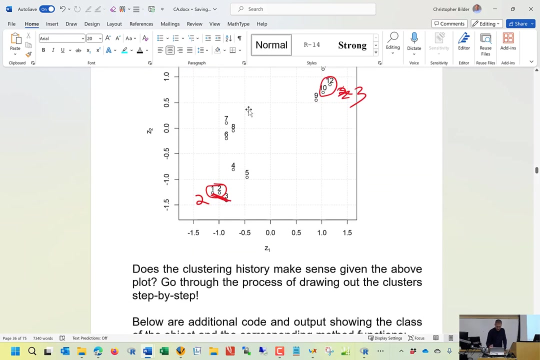 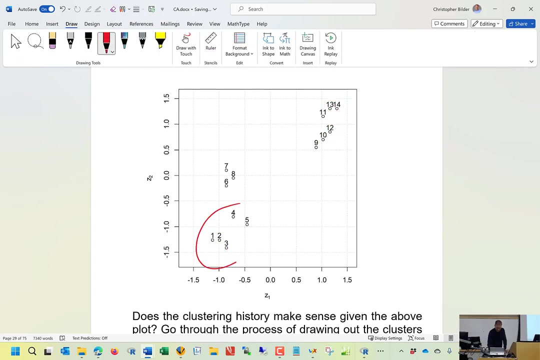 there's only a little bit of change in distances there, So 4 would not make sense in this particular case. So what are the 3 clusters? Let's see here. We'll just go to this diagram here. Those are the 3 clusters. 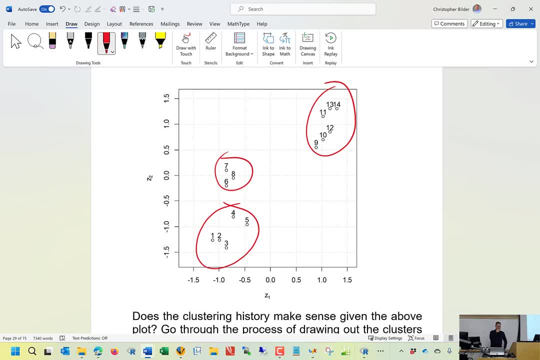 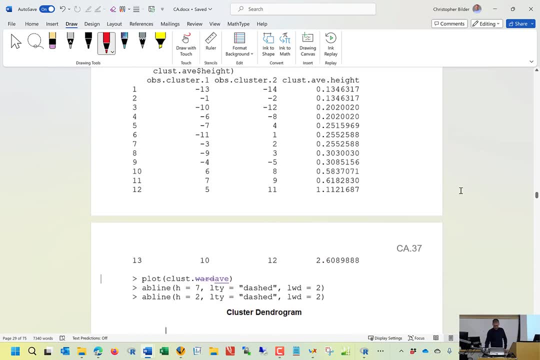 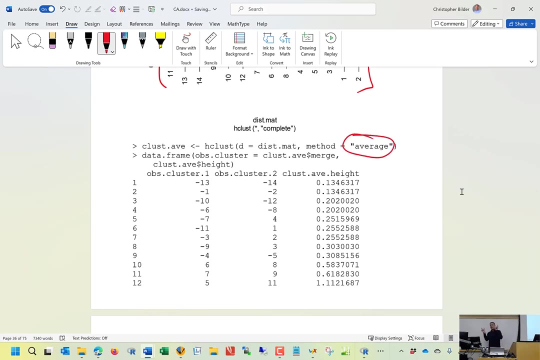 And again, it makes some sense to choose that. Okay, So you know, if I were to draw a line going across, that would make sense. Well, what if I used the average method? Remember what the average method does. Let's say, if you have, 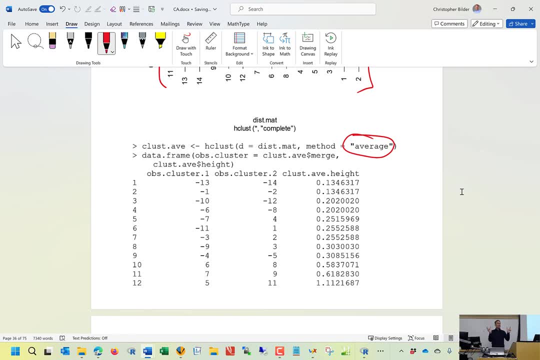 2 clusters. you need to find how similar they are, or in other words the distance between them. What it does it looks at, let's say, if I have 5 observations here, 5 observations here in the different clusters, 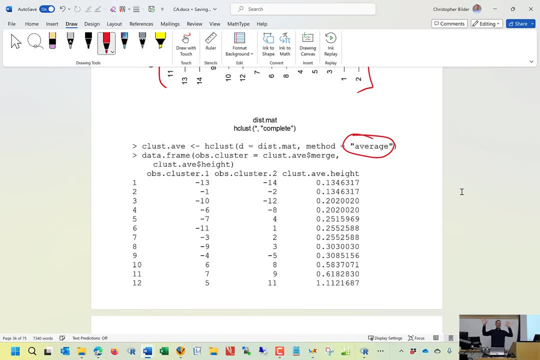 It looks at 25 different distances, all pairwise distances that could happen between these observations and these observations, And it simply averages those distances And that's then the distance between this cluster and this cluster. And so, in this particular case, when I use the 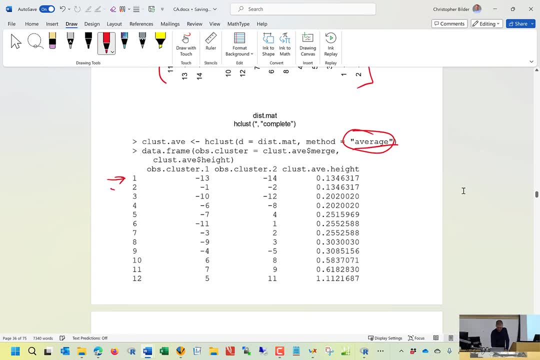 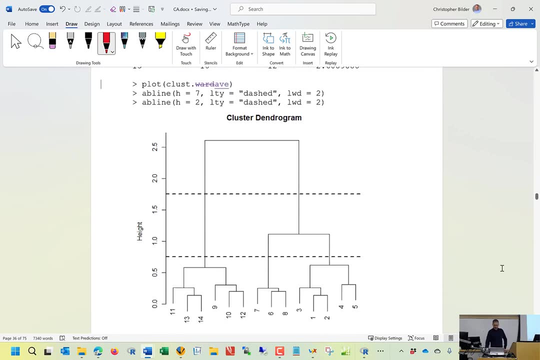 average method. again we start off the same way, And actually even the third step is exactly the same as what we had with furthest neighbor. Here's my hierarchical tree diagram. Once again, 2 clusters and 3 clusters make sense. 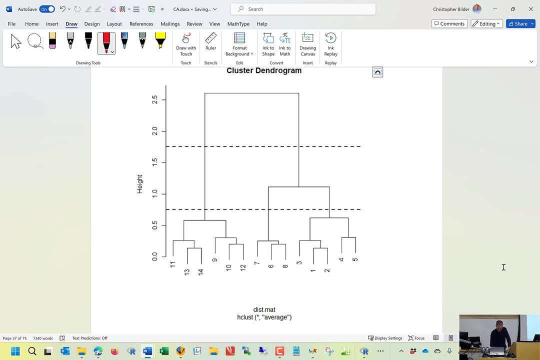 Perhaps also, let's see. this is the same as what we had with furthest neighbor, So this would be 1,, 2,, 3,, 4, 5.. 5 clusters might make sense as well. Now, 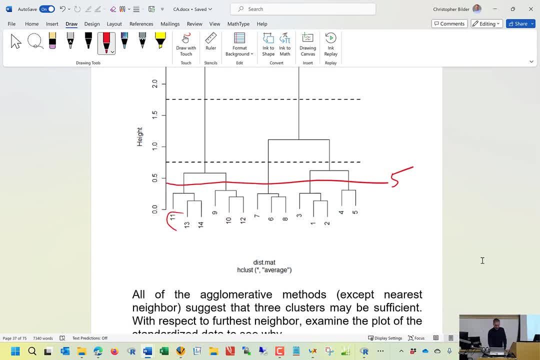 you might be also wondering: why are all these numbers, let's say, at the same level on that x-axis? Why don't they just draw that way? And the reason why R does that is it's trying to avoid overlapping of the numbers. 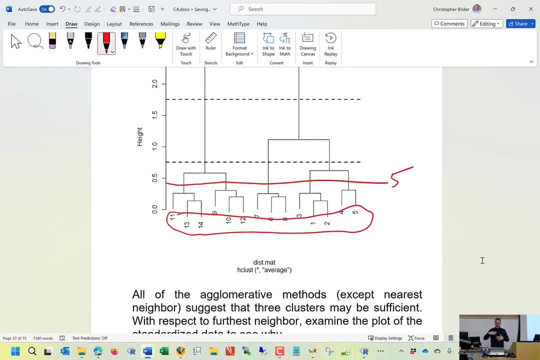 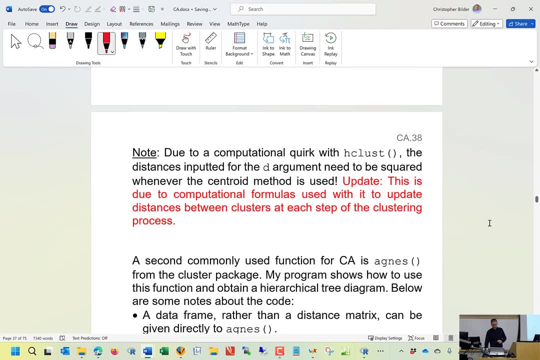 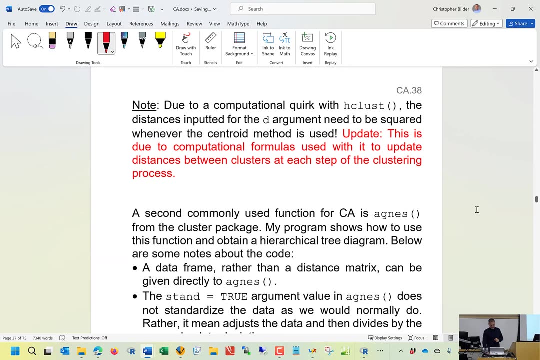 Because if I had, let's say, 100 observations, you would have to try to draw them up or down in that plot. Okay, Now, when you use the centroid method, this is something very odd. I haven't seen this in other. 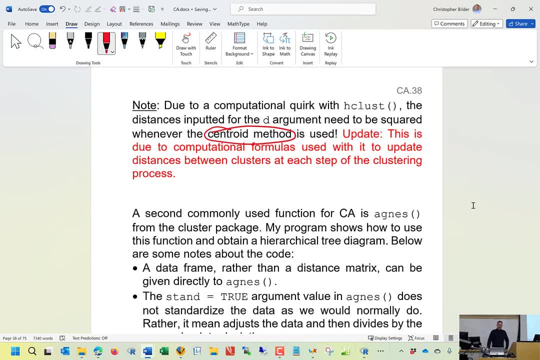 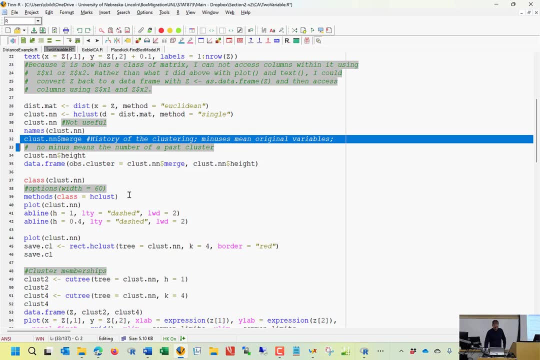 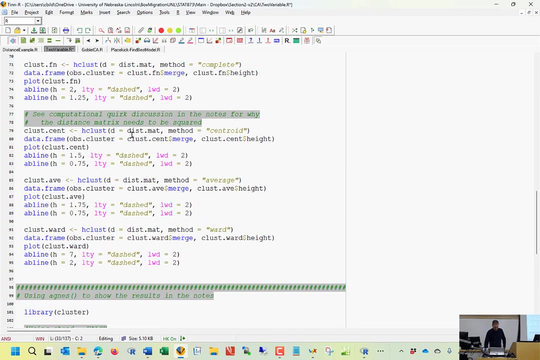 software packages before. When you give distances in each cluster, the distances need to be squared. Okay, let me look at my program here. So, in other words, all you need to do, it is correct on the web, All you need. 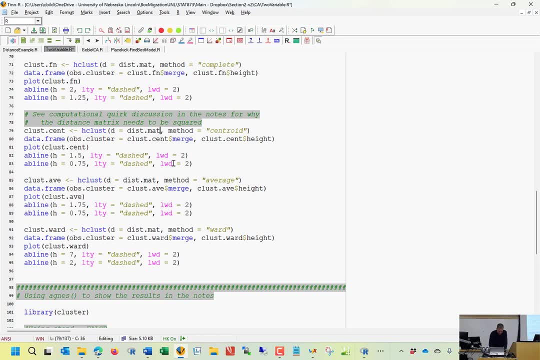 to do is when you use the centroid method. let me just specify centroid. you're going to use centroid, But you need to give it a set of distances that are squared. So if I just simply take this dot mat, square it. 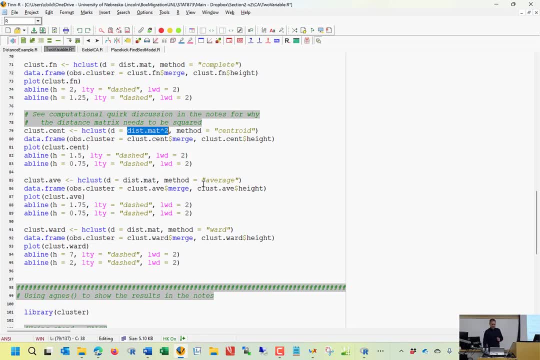 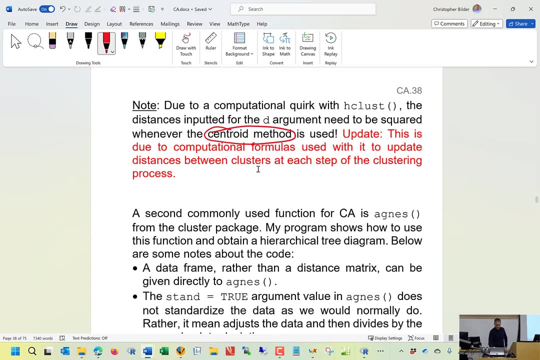 caret type two. this is what's going to get me Now. why So? as I say, it's a quirk, computational quirk, And I was. I don't like computationally to be intuitive and stuff, or if. 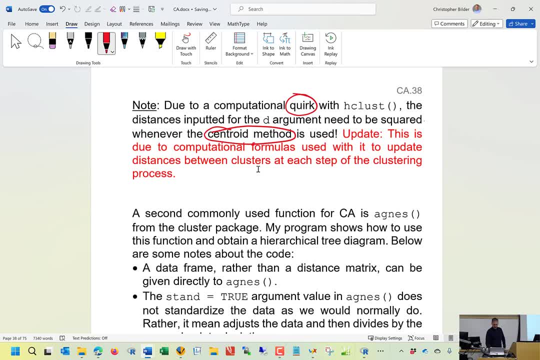 something needs to be done, it should just be done automatically, And I was looking into this a little bit more yesterday and here's why I should have this in there before in the notes. It's simply because remember what the centroid method. 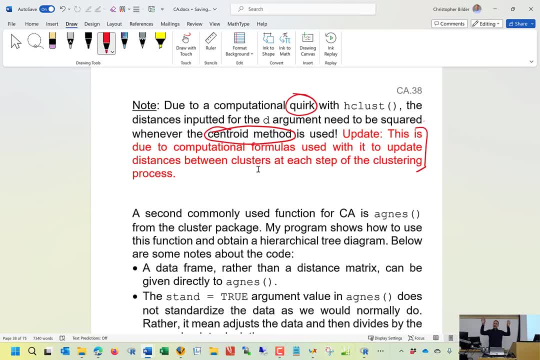 does. The centroid method is to find the average of all these observations, and then I find the distances between the averages. This is different from the average method. Obviously, there's some similarities in the terminology, But now let's say I had. 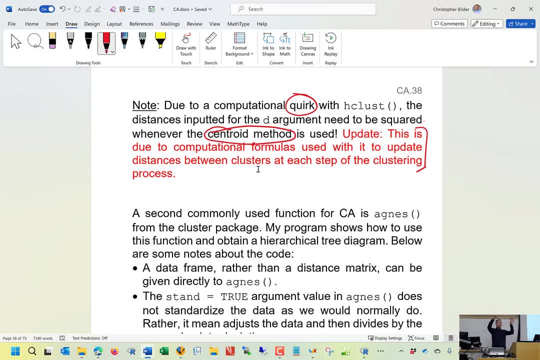 five observations and I had to compute the mean of all six observations again, And so as you go through the clustering process you're going to have to continuously update where that center of that cluster is by continuing to use the average, And I 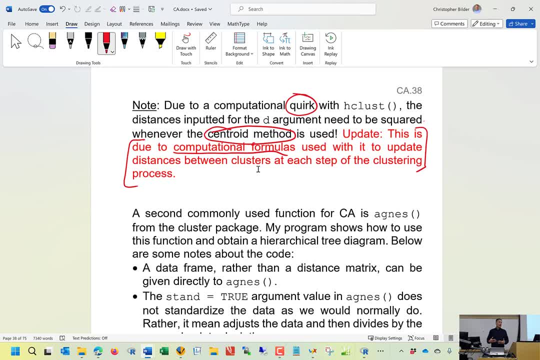 haven't looked into that yet, but I think that's going to be a little bit more complicated than what I was talking about earlier. So what we're going to do is we're going to look at the number of observations that are in the 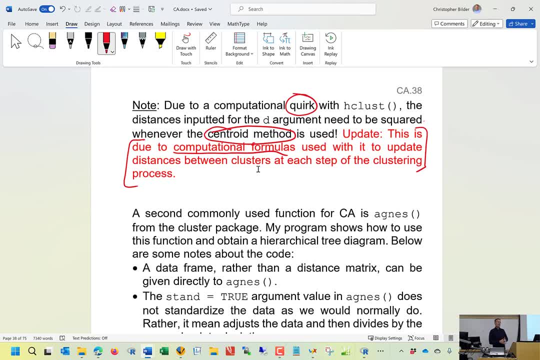 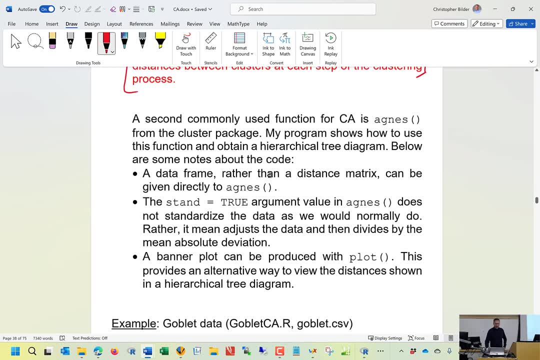 cluster, So I haven't looked at it in depth Now. I haven't really seen it actually explained in other books and stuff before either. And people rather than, let's say, using HCLUS like we've been doing, they use a function. 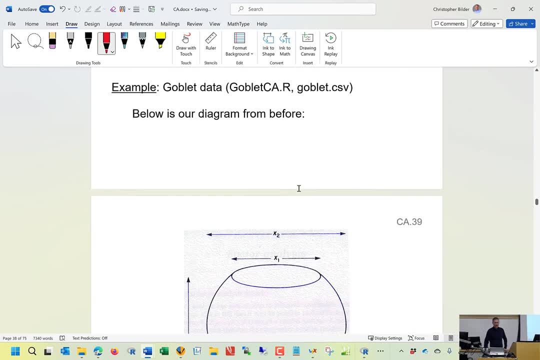 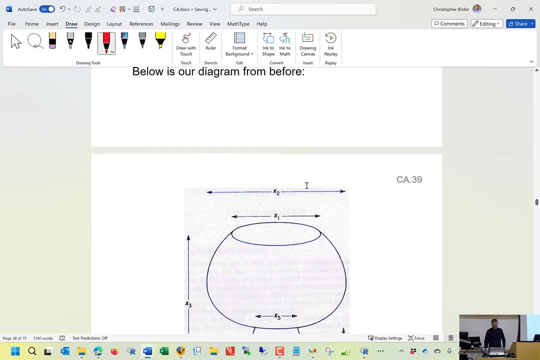 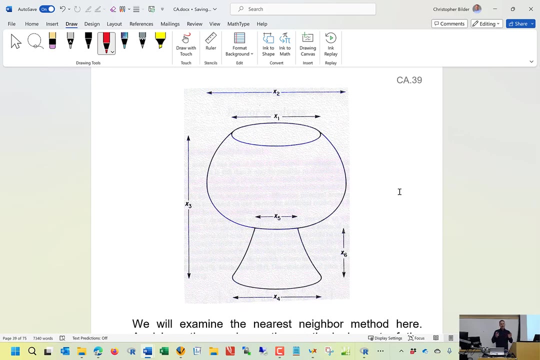 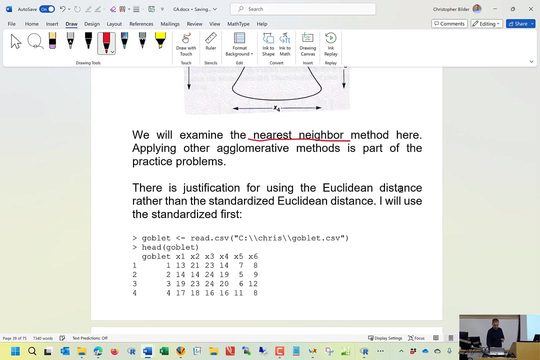 called AGNES, And this just gives you some information about that. Perhaps I don't need in the notes, but I have it there still. So let's take a look at now the goblet data and do some analysis of the goblets. 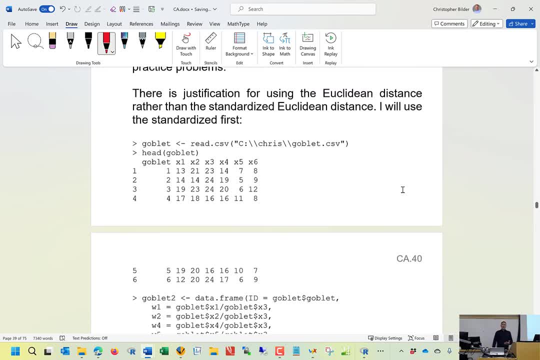 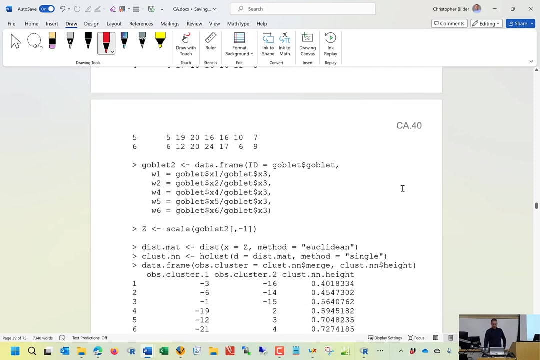 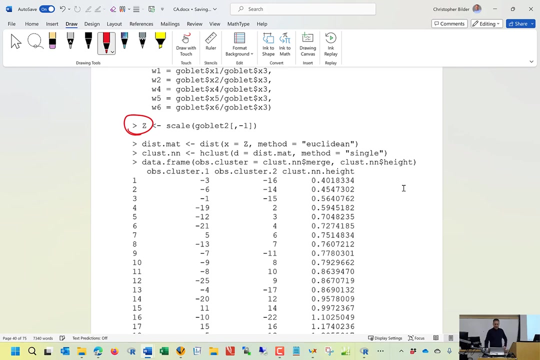 We're going to look at this with respect to the nearest neighbor method, So we're going to also use standardized Euclidean distance. This is one of the few times we've done this before. I then find my standardized values as what we've. 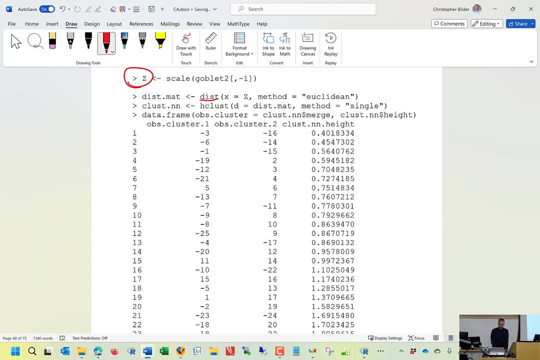 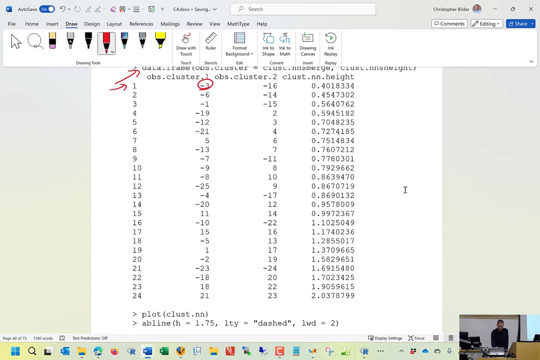 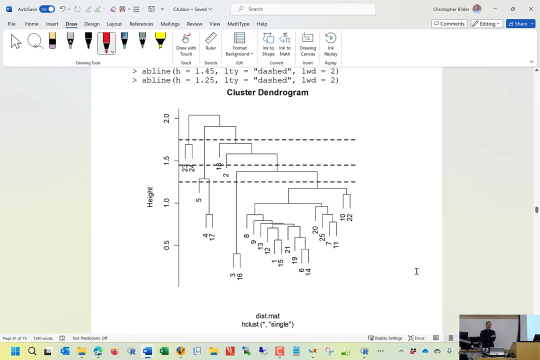 done before, put it into an object called z for the lack of a better name, And then I summarize everything in a nice little data frame here, And so what this means is that when r starts the clustering process- observations 3 and 16- 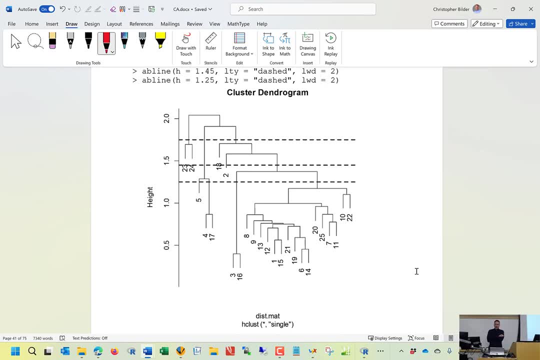 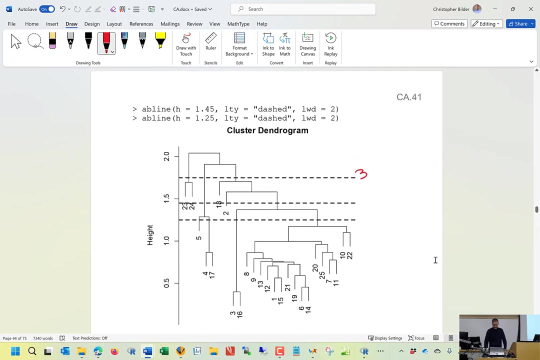 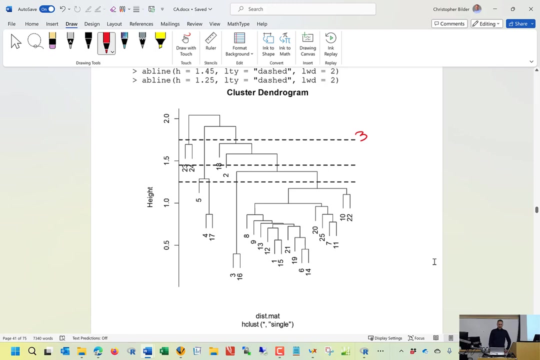 are joined first. The last thing that we need to do is to designate what potential places to, let's say, cut the tree would be, So we can see for the highest horizontal line. we have three clusters there, So 23 and 24 is in. 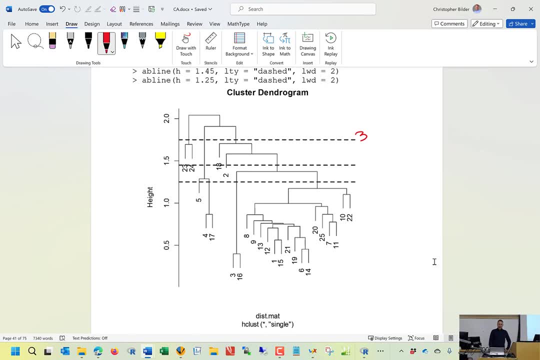 one cluster, 4,, 5, and 17. those goblets are in another one And all the other ones are in the third cluster. Now I also have six clusters. You have to be careful there because, again, since ours is trying to, 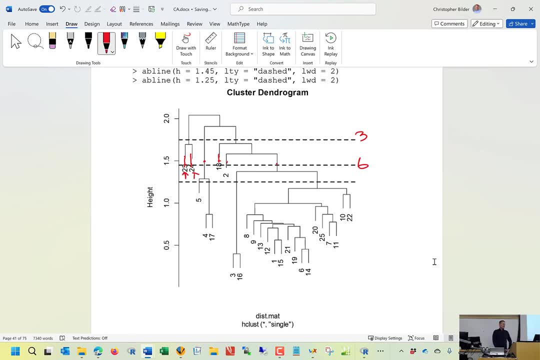 avoid the overlapping of these numbers there I still need to account for this would be the case where we have, let's say, one, two, three, four, five, six, seven, eight clusters as well, And so to make these judgments about. 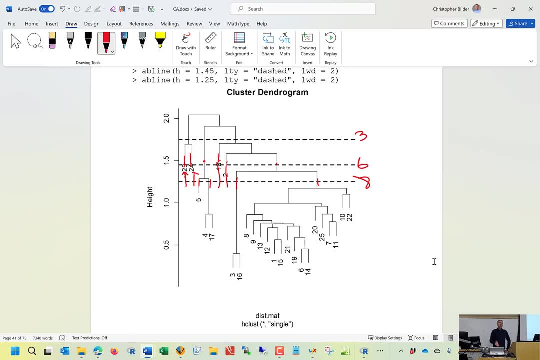 where I drew the line between these two clusters. Why didn't I choose two? Why is three preferred over two? The distance Notice when I go from three to two. I look at this distance there. So that's why it makes sense to. 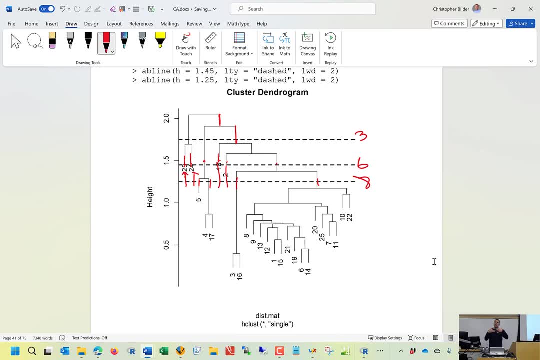 draw the line at three, not at two, And since there can be multiple choices here. but when I grade you on a test, how would you decide the distances? I was just looking at the plot there. I'm looking at these distances from. 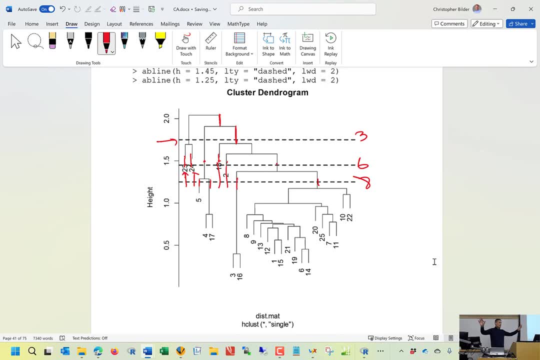 let's say, going from five to four clusters, four to three to five to four, six to five and so on. And so when I saw that that distance was relatively larger, That's why I thought, okay, that would be a. 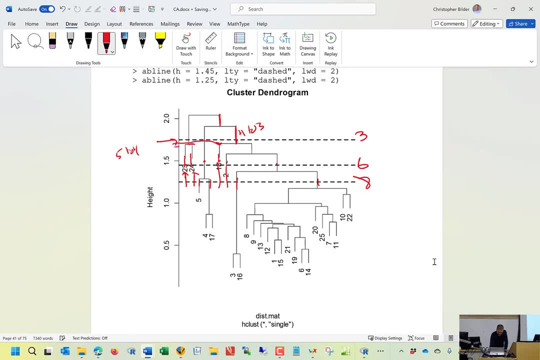 good place to draw that very small distance there, And so it would not make sense to draw the line there. So, for example, if you go from six to five, the distance would decrease. So if you continue, even with decrease, we see 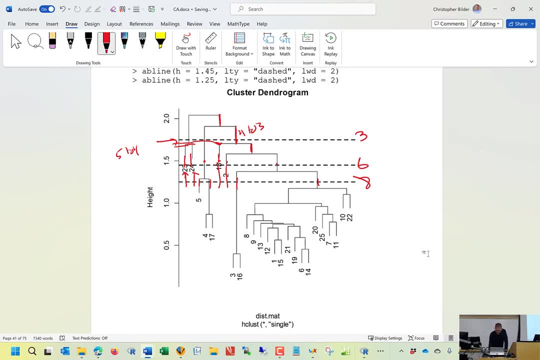 the decrease from six to five until well, maybe we need to back up a little bit. So when I go from seven to six we see that that distance there actually went down. The relative, I mean, I should talk about the. 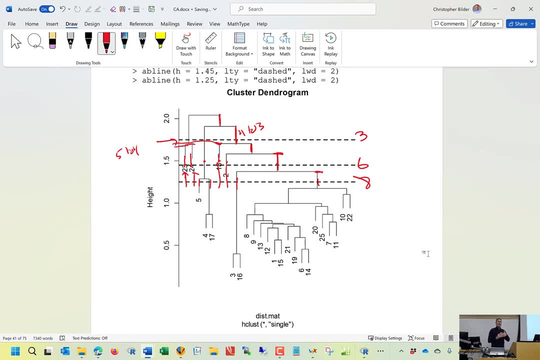 change in the distance, We see that that distance goes down, so that's why using five clusters would not be justifiable. I'm looking for jumps in these distances where the distance goes down. So my question: I should say that so. 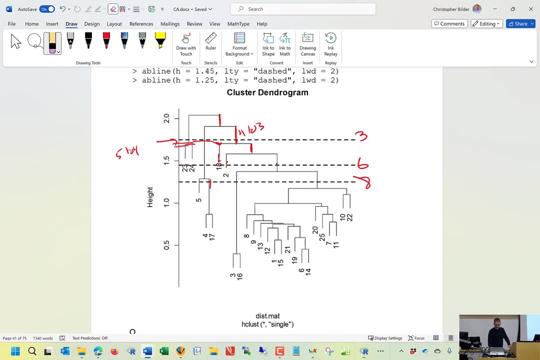 why we choose six over three, why we choose three over six. Okay, I'm sorry, From this plot alone I don't think it makes any sense. If I also look at this plot, I see that if I had six clusters, 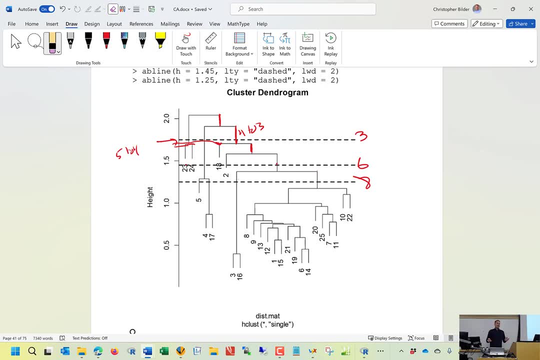 23,, 24,, 18, and two would all be in clusters of size one. then that calls into question: okay, do I also have these three other clusters that are all quite different from the rest? I'm going to put them. 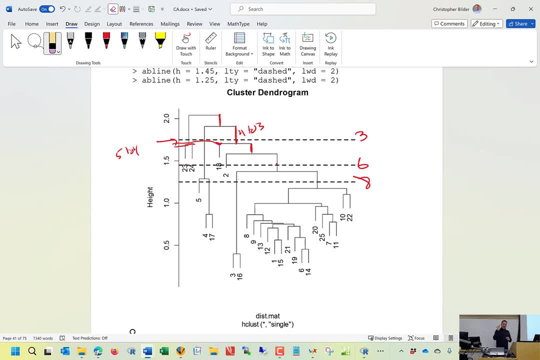 in each of their own groupings. That kind of defeats the purpose of, let's say, finding clusters that are similar to three. or should I just use three, I'm sorry. should I use six or should I use three? I should. 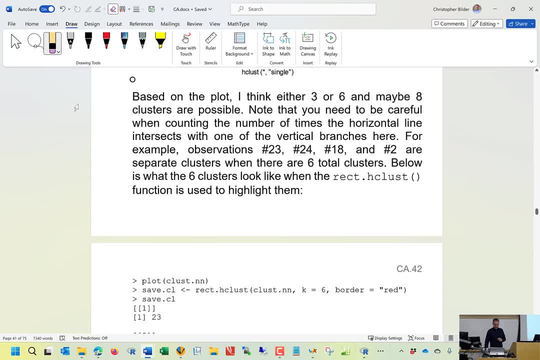 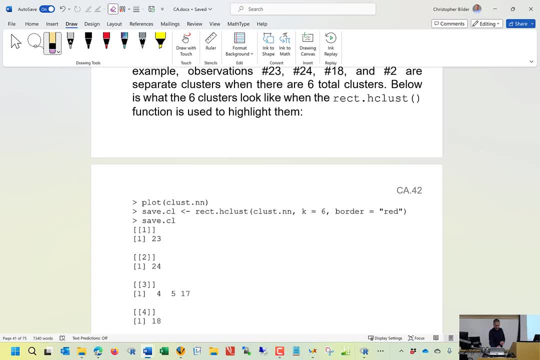 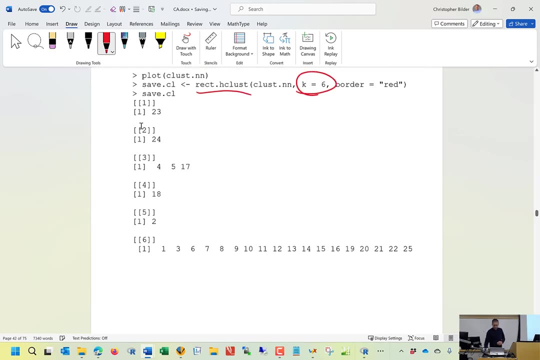 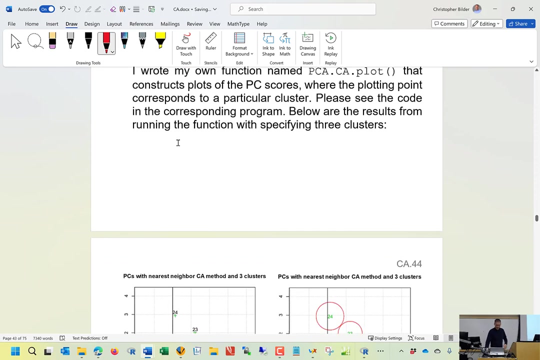 just put it that way, okay, So stay tuned. Any other questions about this diagram? Well, what if let's see so again, we can see how everything is actually kind of diagrammed out for you, and this is something. 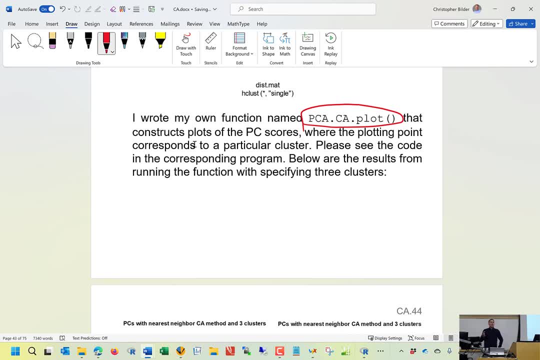 that can be very helpful. So previously we used principal component analysis to kind of come up with an informal way to group the observations. You can classify your choice for clusters. You know, in the previous example where we had 14 observations and we 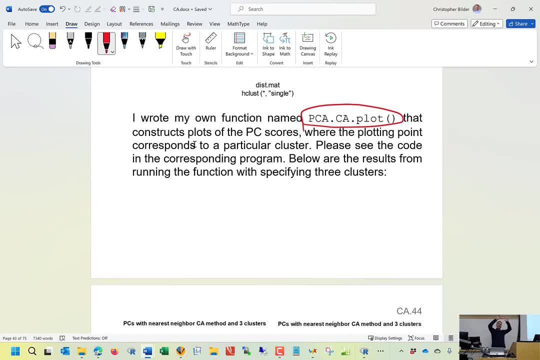 had two variables we could simply draw, let's say, x1 on the x axis, x2 on the y axis, and we could see graphically: okay, yeah, that makes sense to you. So, if you have, let's say: 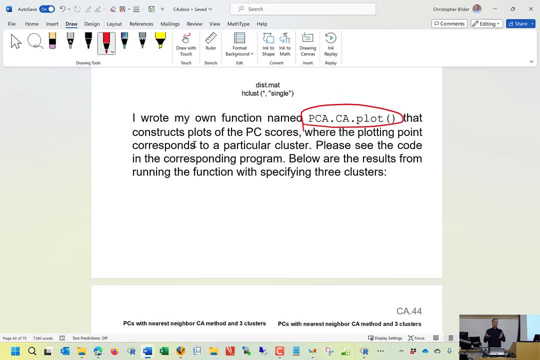 two or three principal components that explain most of the variability in your data, then that should be just as good as in the case where we had just two variables and we looked at a two-dimensional representation. You know, with that principal component analysis you can. 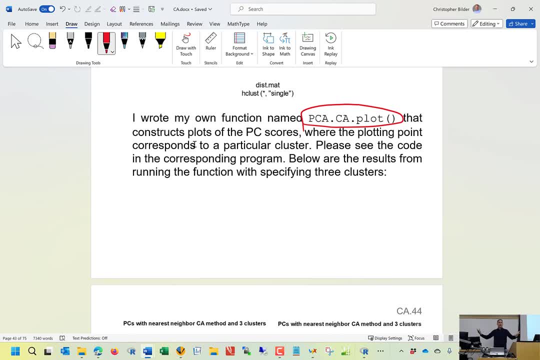 see that the observations are close together, so that makes sense to put them in one cluster, And so that's what we're going to do. next, I've written a function called pcacaplot to help you in this process. You do that. 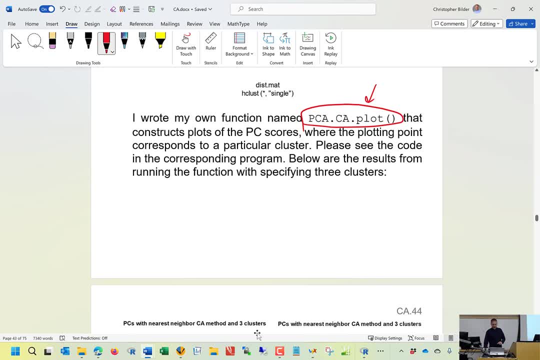 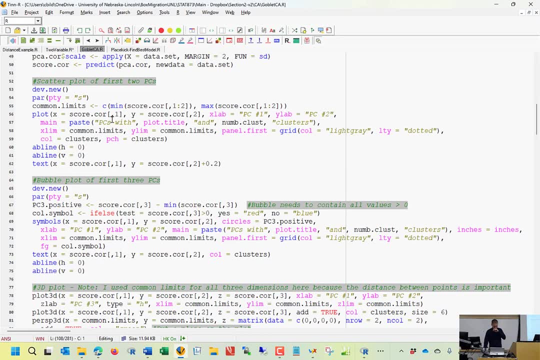 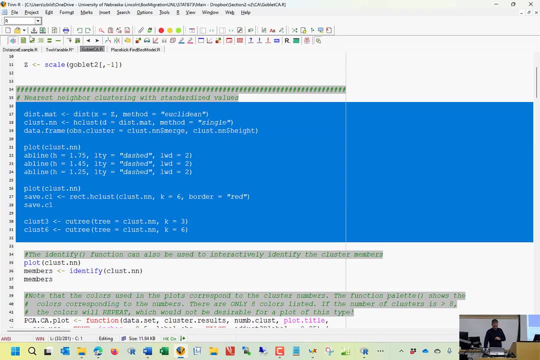 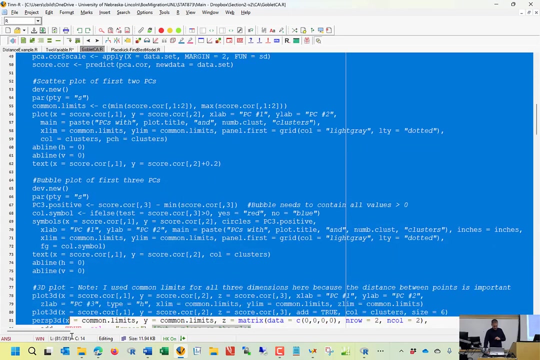 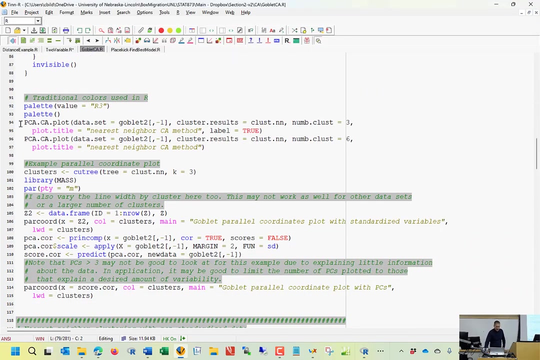 in your own cluster analysis. Take a look at that function on your own. We will look at how to run the function. next. Let me do some stuff here. Okay, So to run this function, I first specify where my data is. My data: 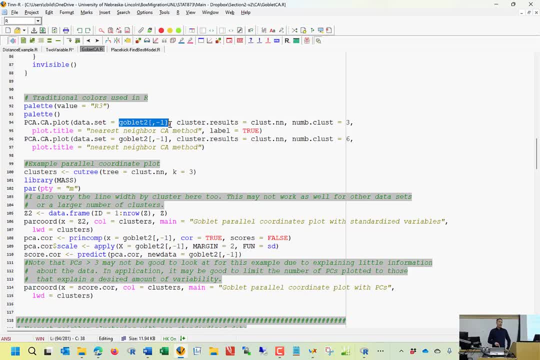 is in goblet two, It automatically. this function will automatically find the standardized values. I'm sorry, Back up a little. Notice how I have a negative one there. That first column was the observation numbers, And so what it's going to. 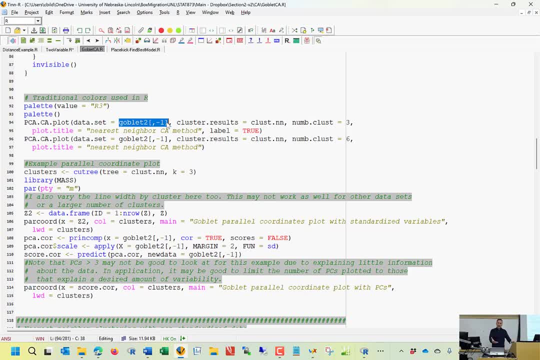 do is take goblet, two the remaining variables in there and it's going to use principal component analysis using the data. How many clusters do I want to actually show on my plots of these principal component scores? How about three clusters I put? 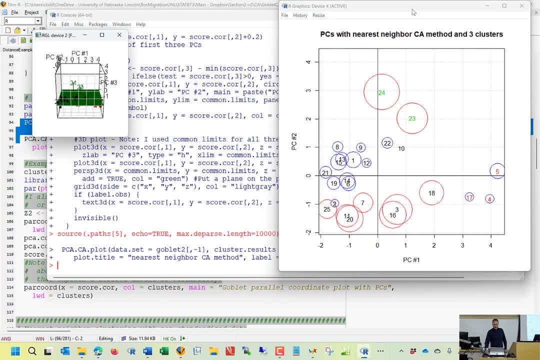 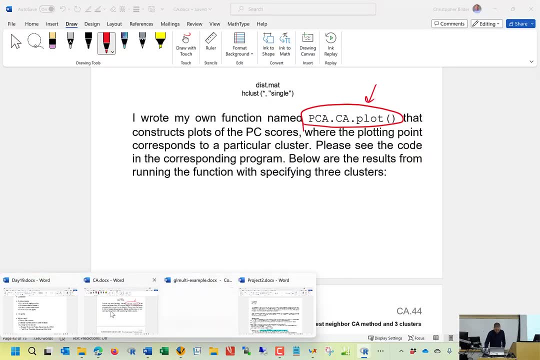 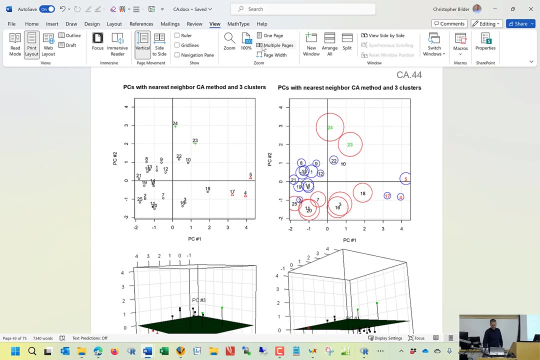 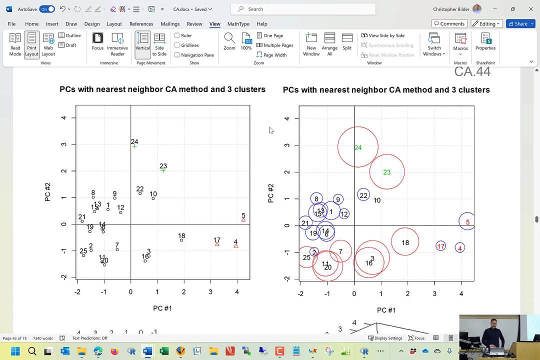 a nice little title on it And also I want to label the points. Okay, So we get this here. So I'm just going to go to this. Actually, we get three plots. Excuse me, Let's see here. There we. 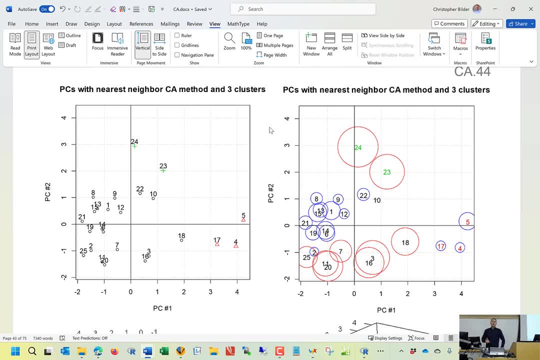 go So the plot on the left, the plotting point corresponds to a cluster. So for what R calls cluster one, based on what R notes, for what R calls cluster number two, the plotting character is going to be the plotting character number two. 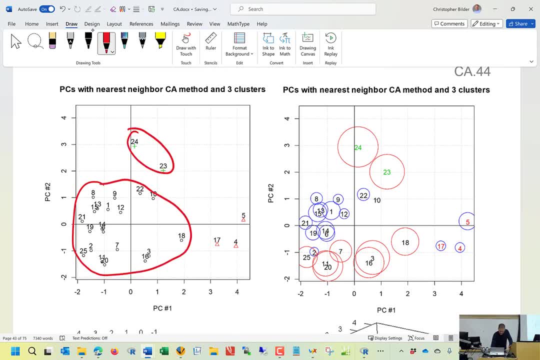 And it's going to be what R refers to as a triangle. And so we can see that we have two principal components And in this analysis, we had- oh, I remember off the top of my head it was like 87%. 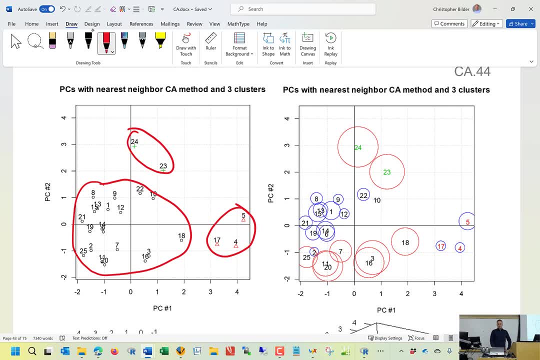 of the total variability explained by two principal components. So I'm thinking, okay, wait, a second, 18 is with this cluster over there. Is that really something that should be done? Well, now, take a look at this, Look at this. third, 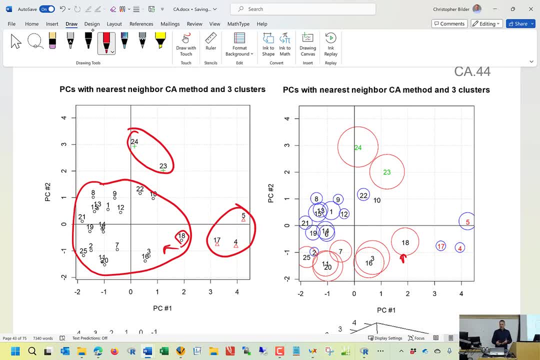 principal component, how you know bubble is. It's a large bubble, So it is, you might wonder. well, wait a second, you know, look at some of those bubbles there. relative to excuse me, let me just make. 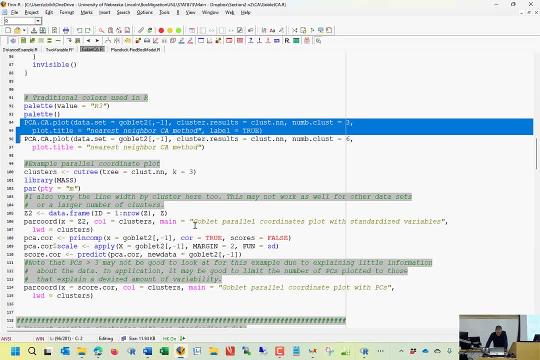 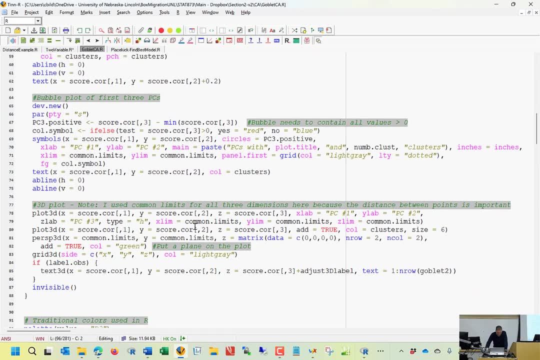 sure I got this right. Okay, yeah, So the okay, that's what I did. Yeah, sorry, I just had to remember what I did before. So you see red and blue bubbles. Red corresponds to bubbles that are have a. 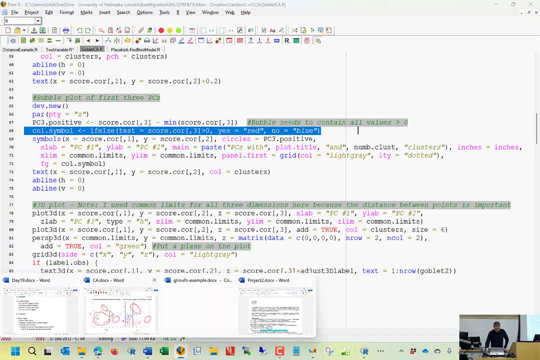 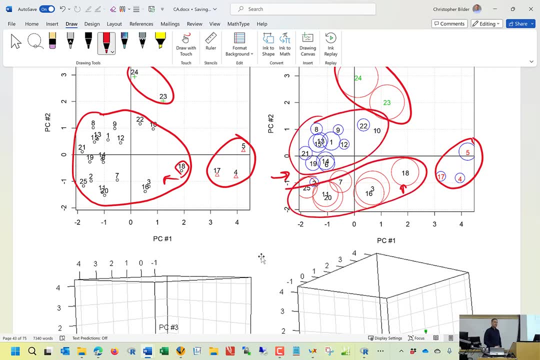 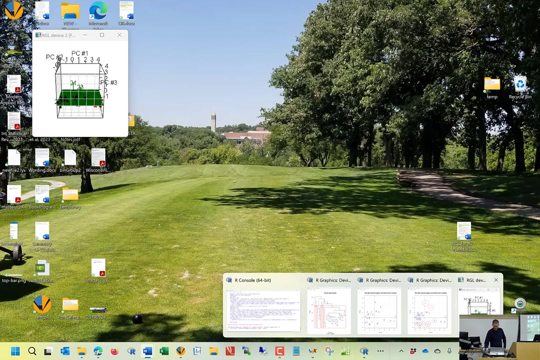 third principal component: that are positive, blue ones are negative. Sorry about that, And so they're there. So that's kind of interesting, But I'm putting them into the same cluster. Well, you know, this third principal component is actually explaining. 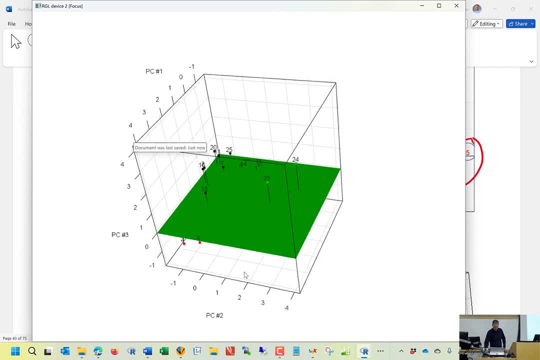 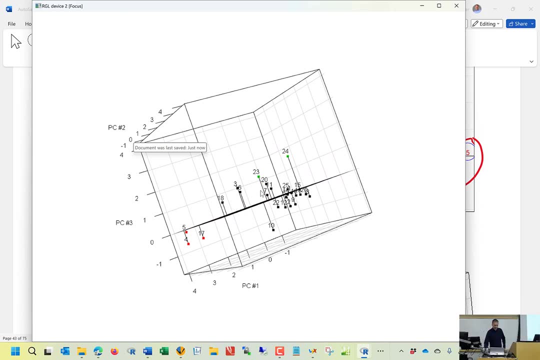 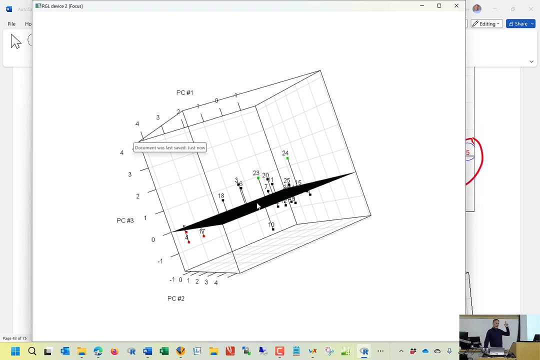 much variability of the data, So maybe that's not that big of a deal. And let's take a look at the first scale, to be exactly the same length. So you know, by doing the bubble plot the way I did, sometimes that can. 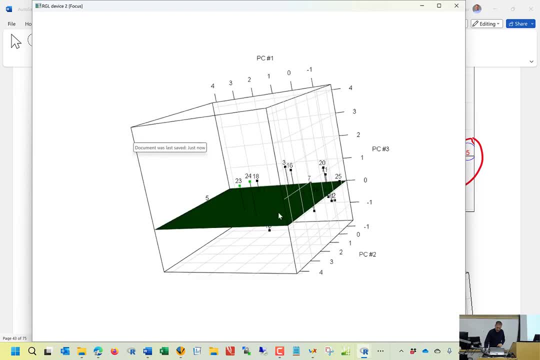 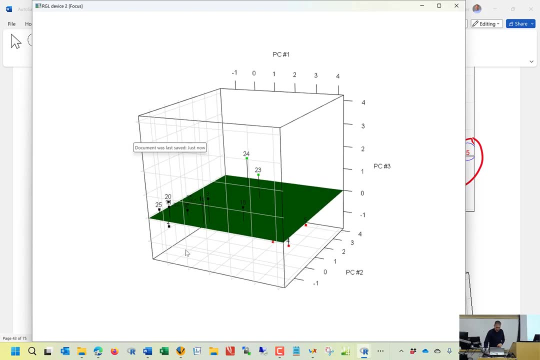 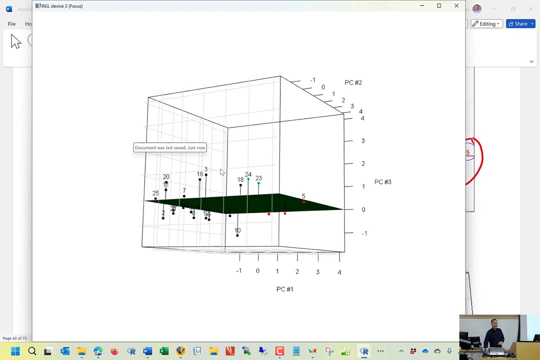 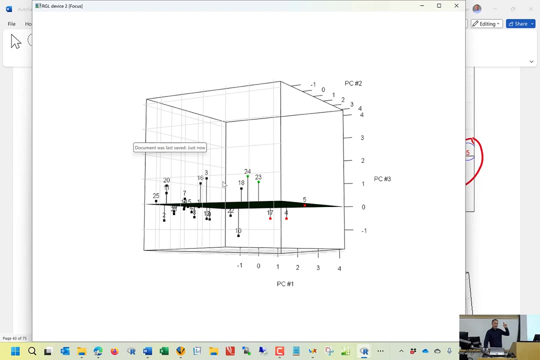 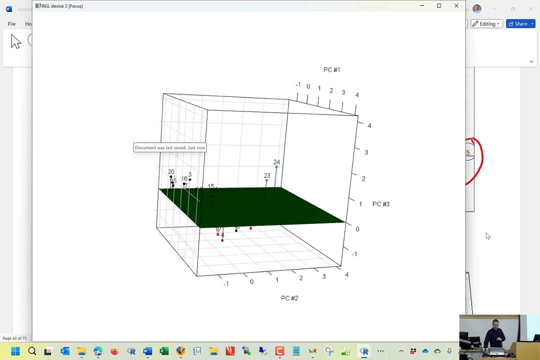 distort stuff, because that third principal component is definitely not as meaningful as the first and second, And so what we can see here here's an example of a three dimensional plot. So this is a three dimensional plot, And this is a three dimensional plot. 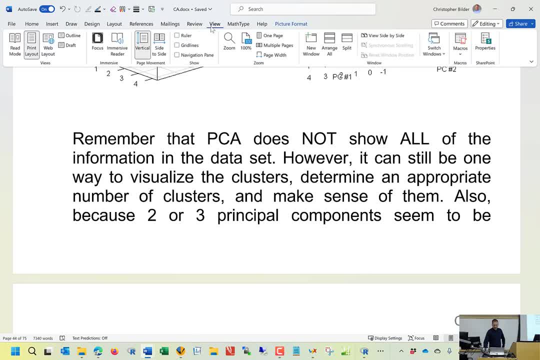 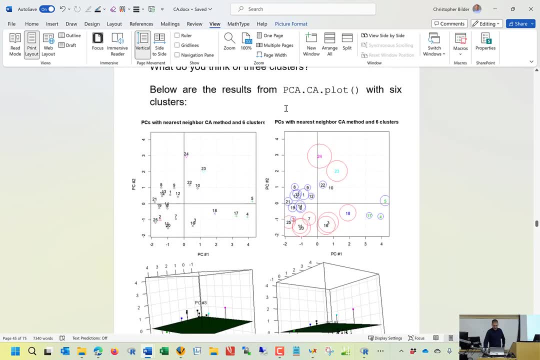 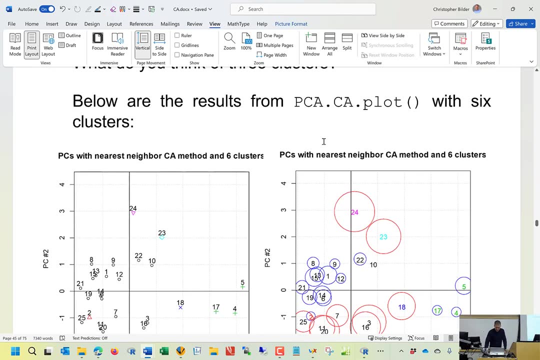 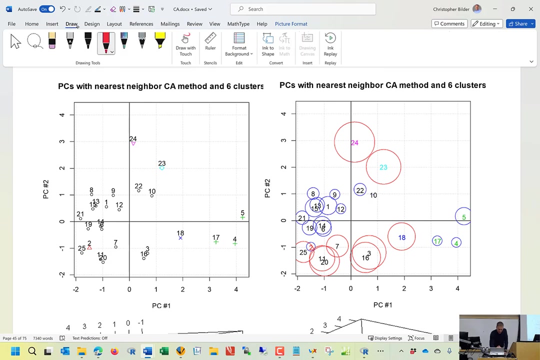 So you know, I seem to be okay with this, Or I should say I am okay with this. Now what if we use six clusters? I'm going to try to get through this quickly. This is what we get. We draw. 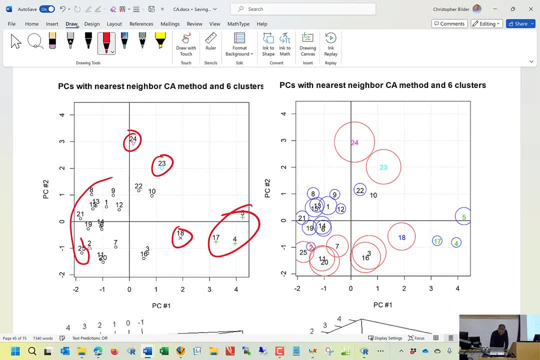 lines around this stuff. So we have cluster here, cluster here, here here, This is the number two. So you know, I mean, just from looking at this, I would think 23 and 24 should be joined together. 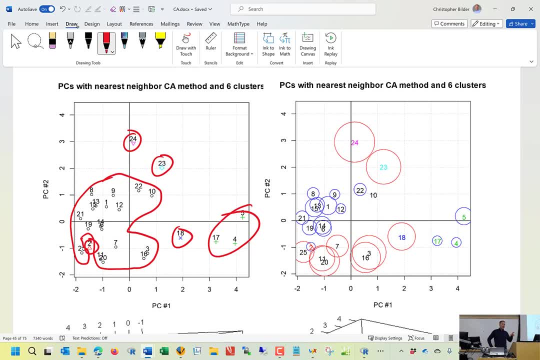 But they're not. Look at number two. Maybe six clusters is inappropriate Now corresponding to this. I don't think that this clustering method is actually finding the true clusters. Let's compare this to when we did the bubble plot here. Why? 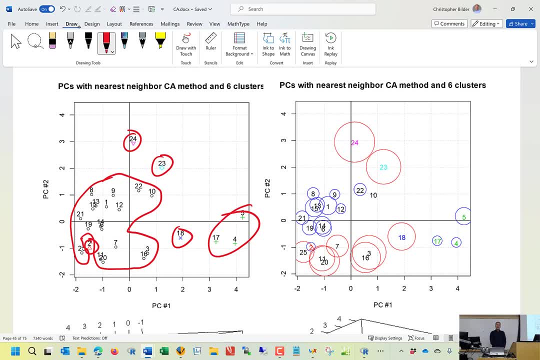 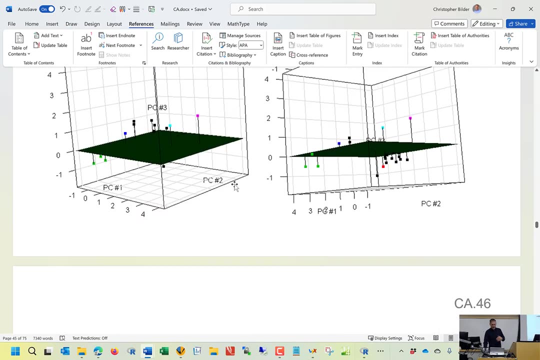 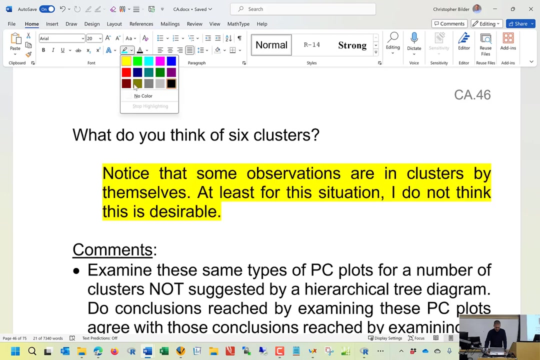 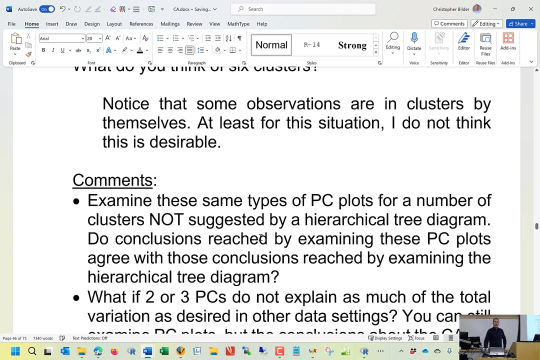 was two separated from the rest. Well, we can do that from the other ones, but then again, remember this third principle component is really not explaining much variability of the data And you can look at all this in three dimensions here. Three: 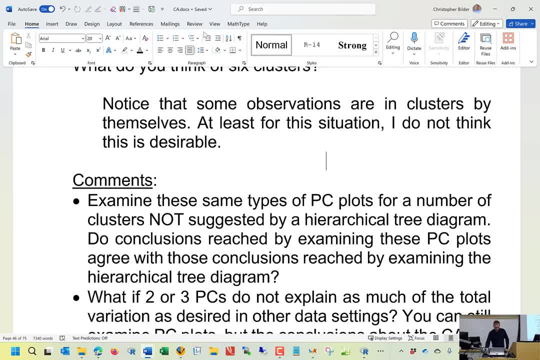 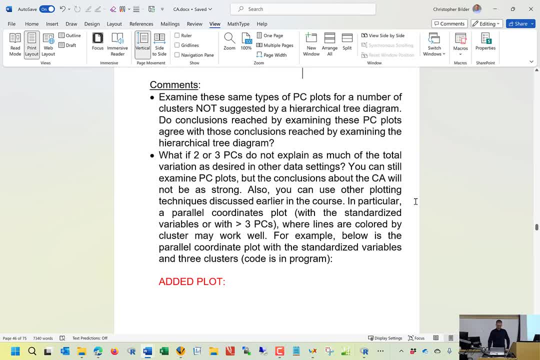 would be better. Okay, let's see here. So some comments. you know. examine these same principle component plots Now for, let's say, five clusters. Use that to justify, okay. yeah, that's why I don't think. 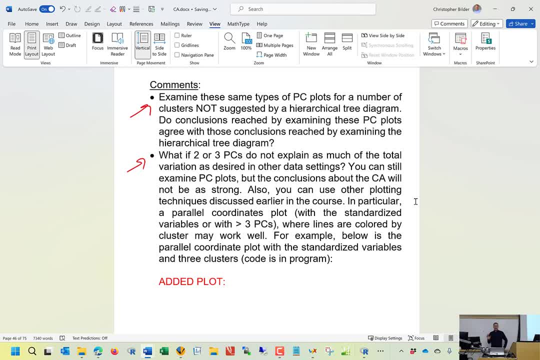 let's say, five clusters is appropriate And that agrees with, let's say, the hierarchical tree diagram. So you could be missing out on important information. So I would still look at these plots, But what I would also do is do some of 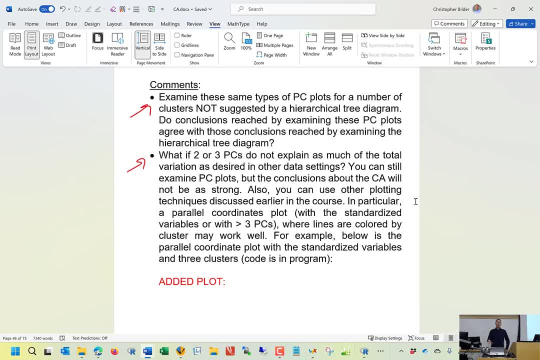 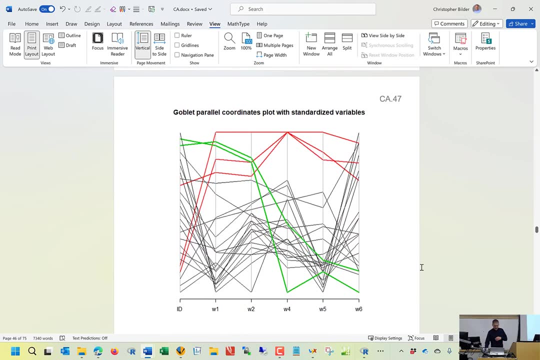 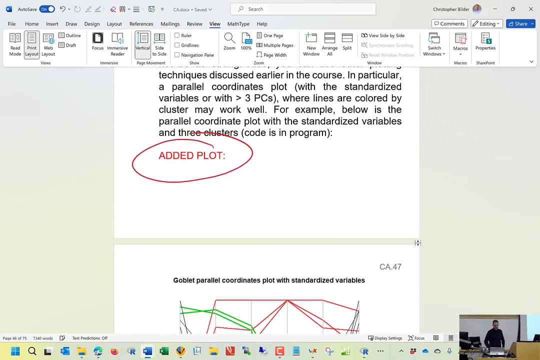 these other plots that we have available that can represent these higher dimensions, such as a parallel coordinates plot. So you could do a parallel coordinates plot, because they're not very meaningful. So, for example, here's: this is a plot that I actually added. 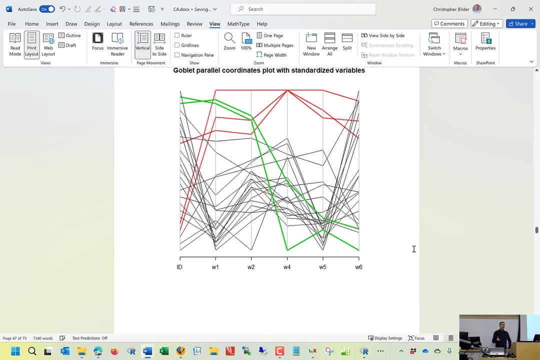 We've done this plot before, essentially, but not exactly in the same way. So here's the original variables. okay, with three clusters, where I designate three clusters would be justifiable. Notice how these reds are standing out from the rest. Notice how. 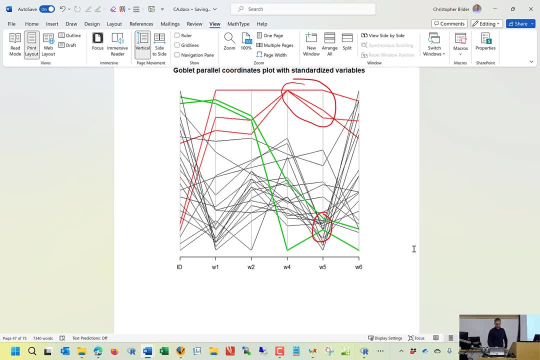 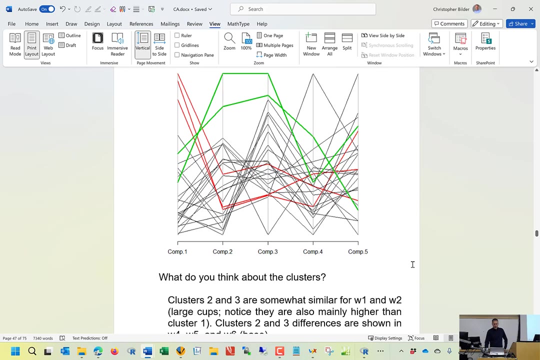 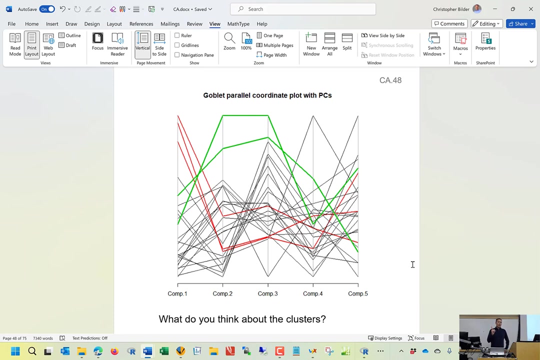 the greens at times are standing out from the reds and at other times standing out from the blacks. This is what I want to see. if I want to actually use this, You could also do this with principal components, but because I know two to. 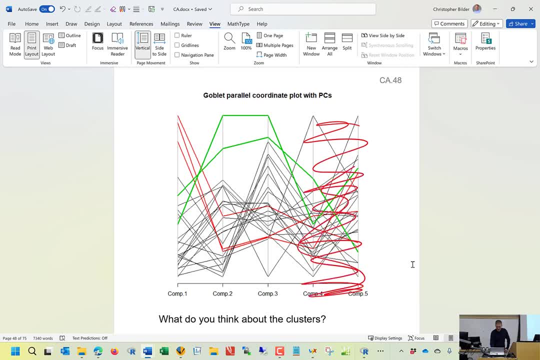 three principal components are justifiable. I don't need four, I don't need five. I would ignore this side here. But once again we can see for principal component number two and for principal component number one, that really separates out the red. 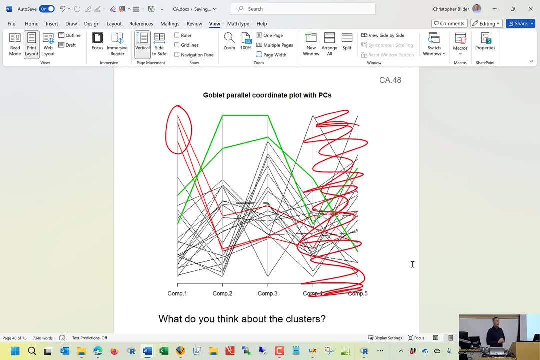 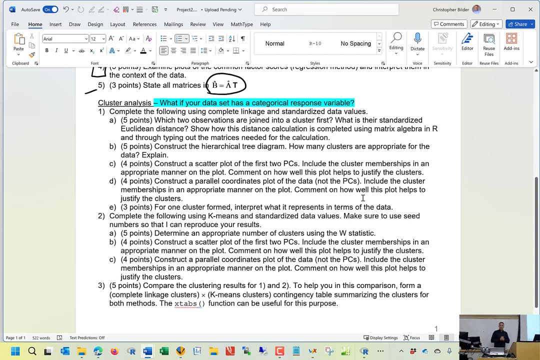 That corresponds to observations four, I think 15 and 17.. The green is 23 and 24.. So you can use those plots and this is what you will need to do at times for your project. So this is the background. 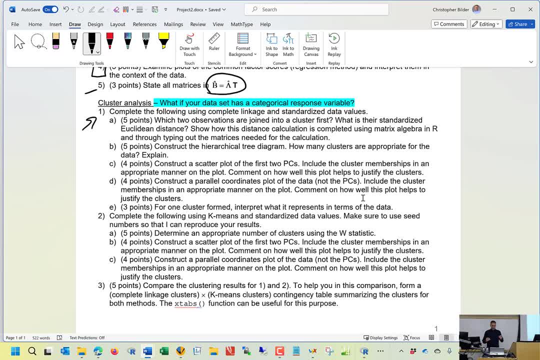 to really get started on the cluster analysis part of the project Number one: use complete linkage. use standardized data values. Now it will be good practice to use some of these other hierarchical methods on this project. Let's just use the complete linkage. 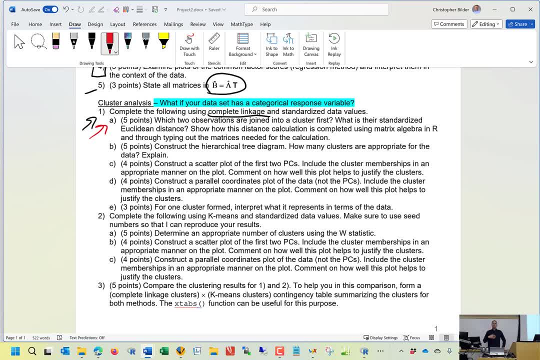 for this neighbor, Part A, here Run H cluster. Tell me which two observations are joined. first, Give me the corresponding distance that R gives you between two points. Do that here with the standardized, Just to show me that you can do it. 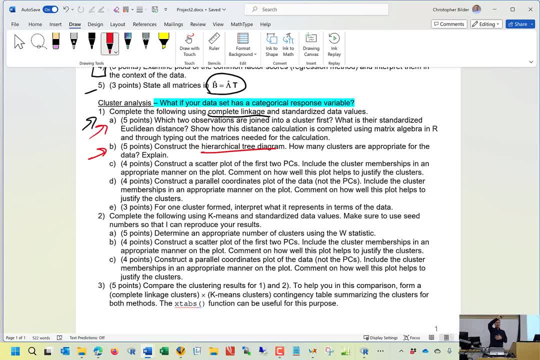 Part B: do this hierarchical tree diagram. How many clusters are appropriate for the data? based upon the data, Give me the written justification. Part C: now do a scatter plot of the first two principal components. Include the cluster memberships in an appropriate manner. 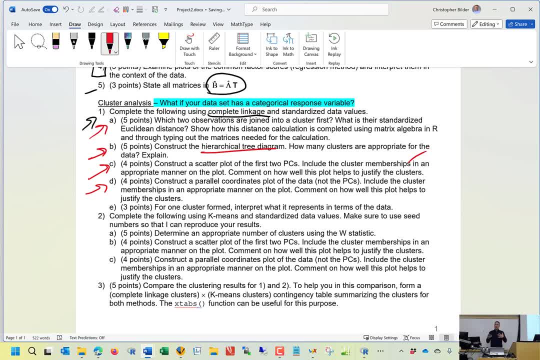 of the plot, like what we talked about. Put the cluster memberships on the plot. Tell me how this helps you separate the stuff out. Take one of the clusters that you have chosen to find. Interpret what you're doing. Do a similar thing. 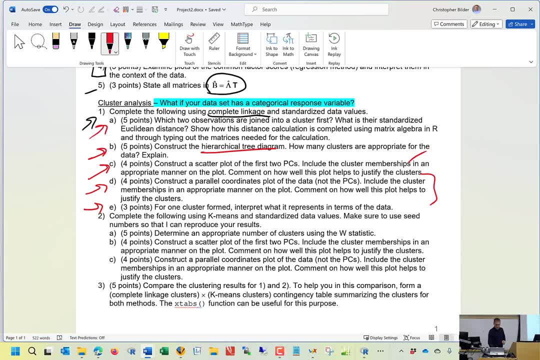 here. So that's number one. Now, remember that cluster analysis is used in situations where you don't, let's say, have some natural classification of your cluster. We had a number of explanatory and independent variables with it. Cluster analysis wouldn't be appropriate.